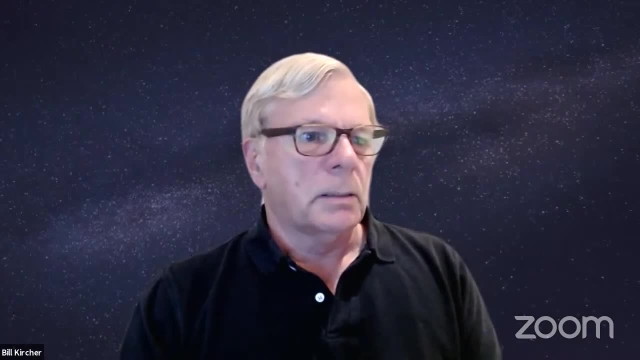 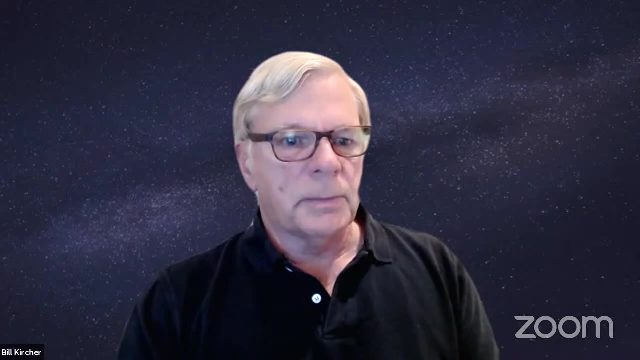 knowing that people may also be watching via live stream. excuse me, If you are participating in the Zoom session. if you could please remain muted, because any background noise can be very distracting and somewhat hard to track down, And also if you have questions. 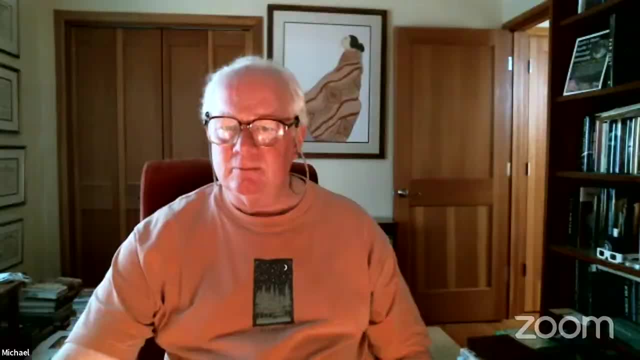 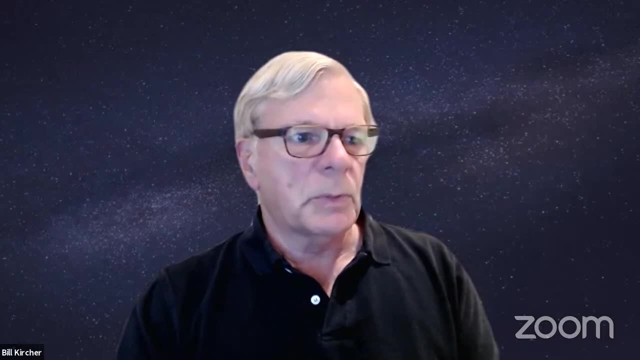 please feel free to type them into the chat stream. We have a lot of ground to cover tonight, and so I'd prefer to address any questions at the end of the presentation as opposed to as we go along. There also is a question that Liz Triggs has typed in: What type of telescope do you have? 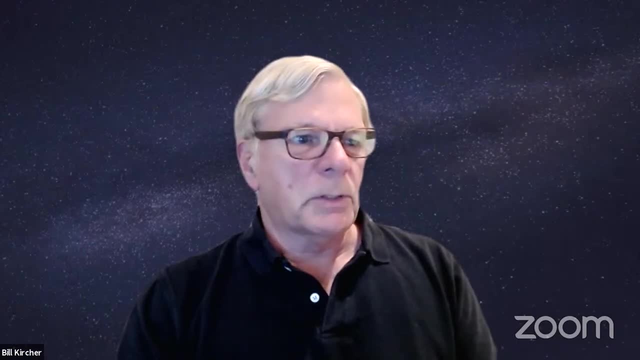 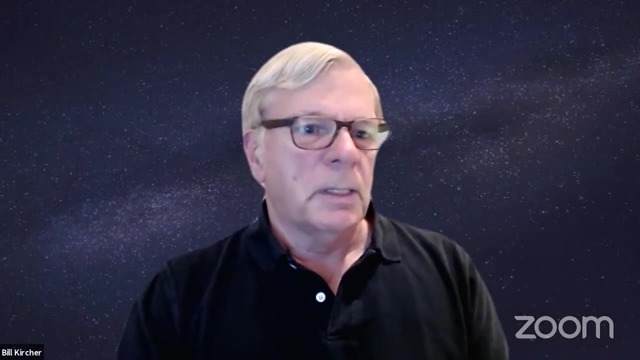 If you have a chance, if you could let us know what kind of a scope you have? Very, very interested to hear that if you have a scope, Some of you may not have a telescope- From the names of those who have logged on so far. 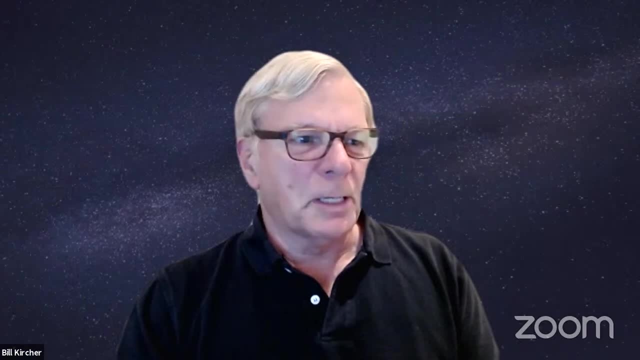 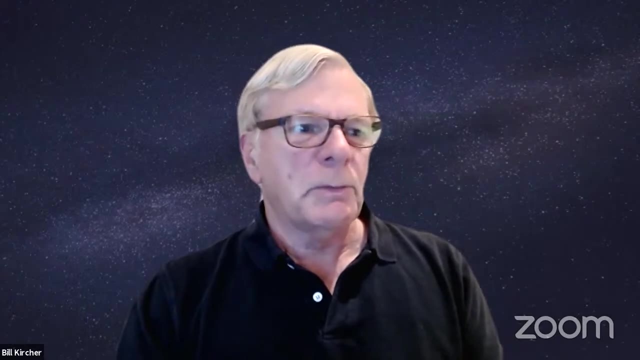 some of you, I know, are experienced astronomers, but thank you for joining us. But the program is going to will be at a level so that, even if you're just starting out, hopefully this will all be clear and understandable to you. But if it's not, 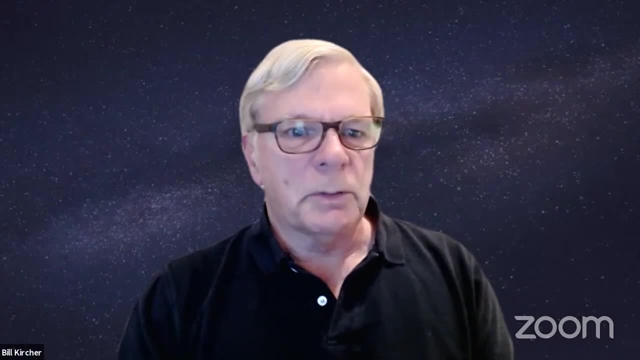 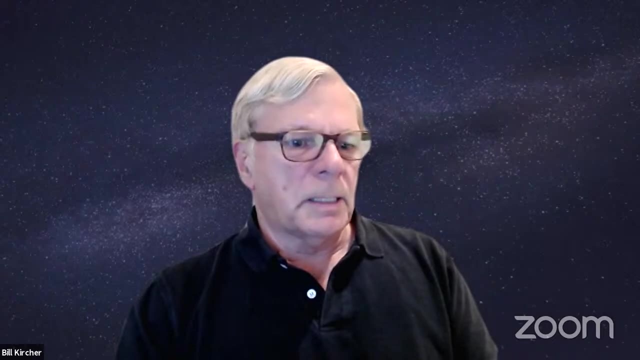 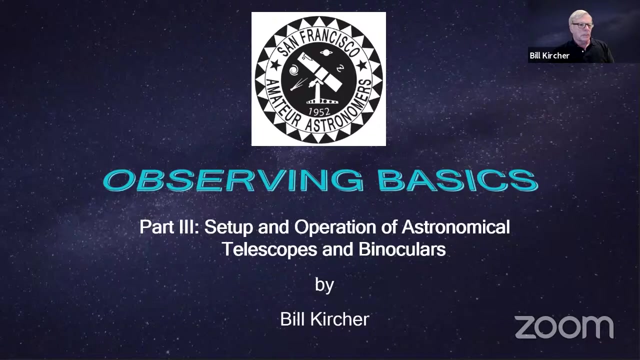 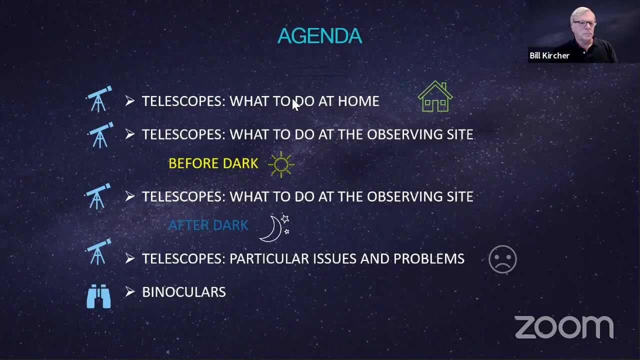 please feel free to type your question into chat and we'll try to address any concerns at the end. So I'm going to structure this in segments, Starting at- well, starting at the beginning. So let me share my screen. So the beginning. here's our agenda. So the beginning is at home: What you can do at home. 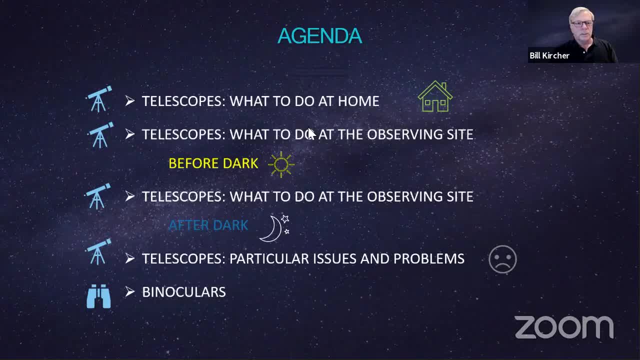 Once we cover that, we'll move on to what you should do at the observing site before DART and then the observing site after DART. We'll move on to from that to discuss some particular issues and problems and then address binoculars. 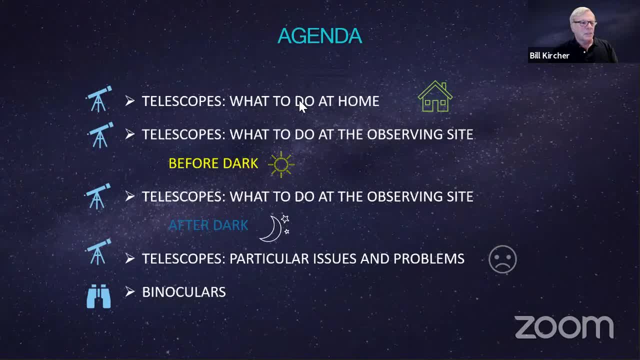 The reason for starting at home is that this is the easiest place to practice, to become familiar with your telescope You have. you can do this during the day you have daylight. you have access to the internet, books, materials, manuals, tools. 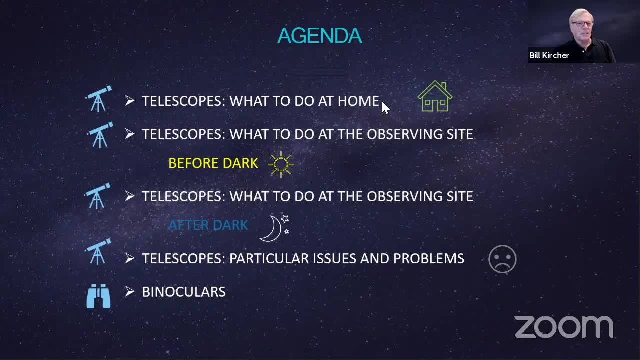 And it's. the more you can do at home before you get to the observing site the better, Because once you get to the observing site, things start to happen, And then it's dark. And doing things in the dark when you're not familiar with 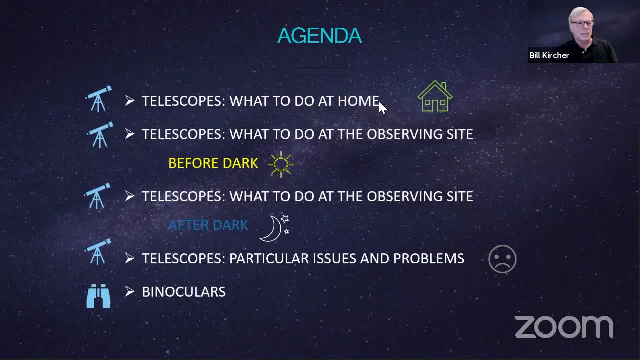 with them is much more difficult than doing them in the daylight. I'm going to assume, for purposes of this presentation then, that you are starting at home, And then we'll take a virtual trip to the observing site, Basically a virtual star party put on by the club on MtTAM. 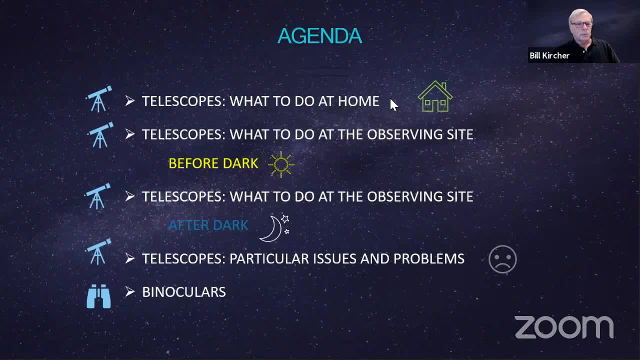 And so the idea is, you start at home becoming familiar with your telescope, and if there's any issues, you can address them before going to the star party in a week or two weeks or something like that. Now you don't have to do this, it's just easier to do it if you have the time, if you can make. 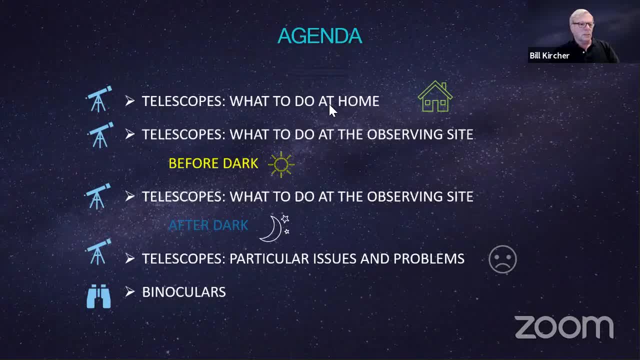 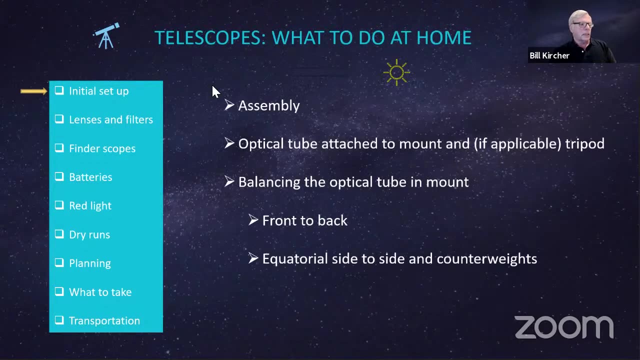 the time. So let's then go on to the first stage of this. what you can do at home, And so you'll see on the left, is sort of a checklist with an arrow at the top, the initial setup, and then we'll just sort of go down this list As far as initial setup is concerned. if you 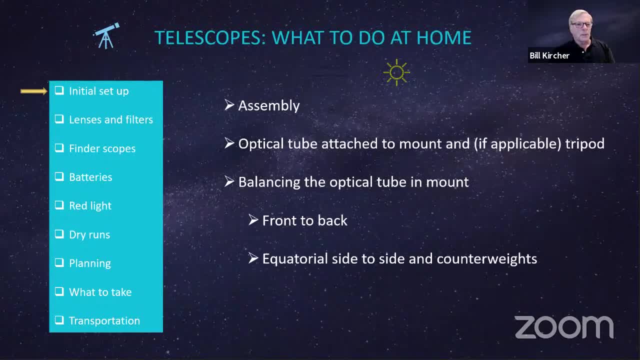 just got your telescope, you haven't perhaps even opened the box. well then, you get to start at the very beginning, because there will probably be at least some assembly involved, and then you put your telescope together. If you have a Dobsonian, you mount the telescope in the 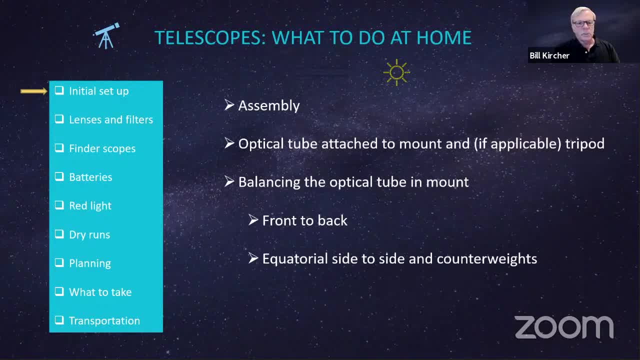 mount. If you have a tripod mounted telescope, well then set up the tripod level it, then the mount head, then the optical tube. There are lots of different kinds of telescopes and I can't cover all of them, so use your manual. If you have questions, go on the internet. 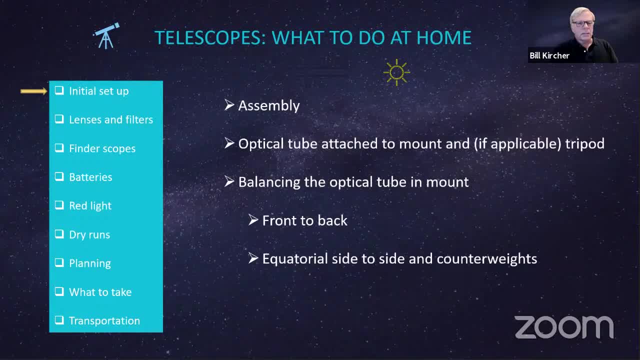 The more popular telescopes. there is actually a lot on the internet. I'll put a link in the description to help you, including YouTube videos. But get that telescope set up to make sure you have all the parts. and if you have a telescope, 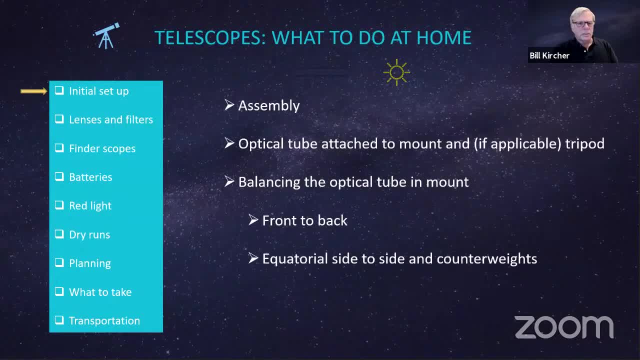 you haven't used for a while. re-familiarize yourself with it. If you're missing anything, are there any problems? then you have some time to try to work that out. Do be careful with the optical tube If you're just setting your telescope up for the first time. 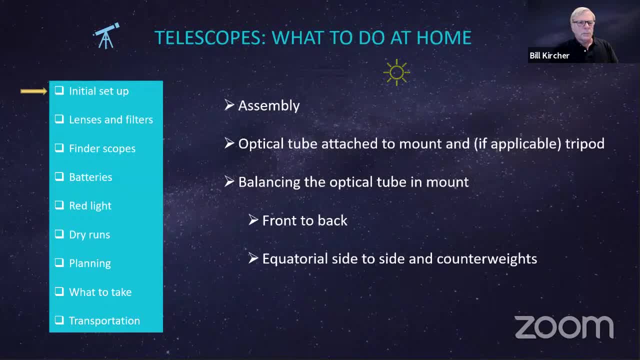 optical tubes need to be handled with care and some mounts are a bit tricky. For example, I have a dovetail mount on my telescope and I managed to not attach the optical tube correctly, so it ended up on the floor. Fortunately nothing broke, but I had quite a collimation job ahead of me. 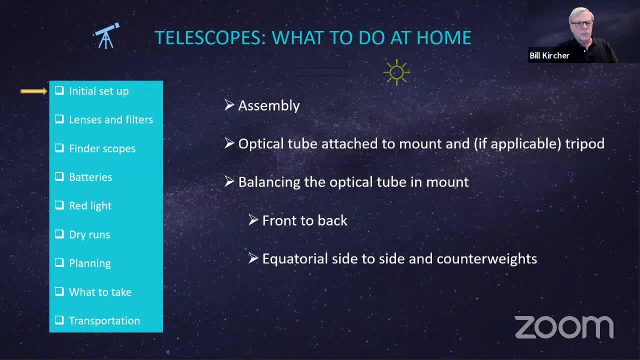 Telescopes also, if they're in first use, need to be balanced. Dobsonians particularly, and equatorials need to be balanced, but all telescopes really should be balanced front to rear and with the equatorials side to side, because you have counterweights. 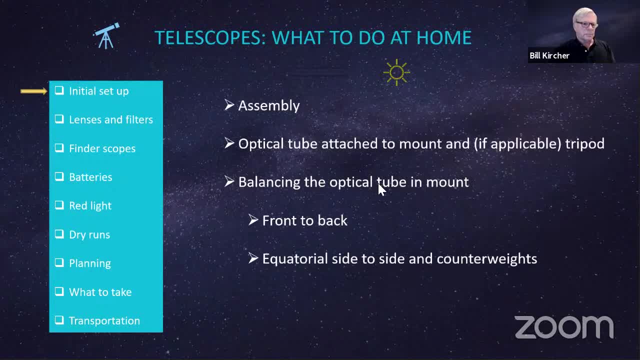 Consult your manual on that. Next, let's talk about lenses. Telescopes come with at least one lens, typically a low power lens. They might come perhaps with an additional lens, a higher power and or a Barlow lens. My telescope came with one lens and then I added a. 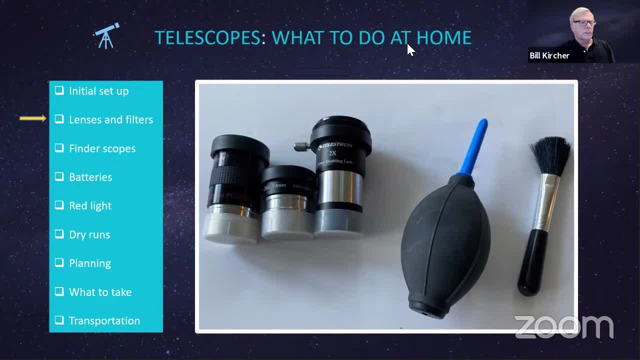 little red dot to that eventually. so the low power lens, I have a little red dot I'm going to use as a pointer On the left, 25 millimeters low power. Later I bought a package: a 10 millimeter, which is a higher magnification, and then a two times Barlow. 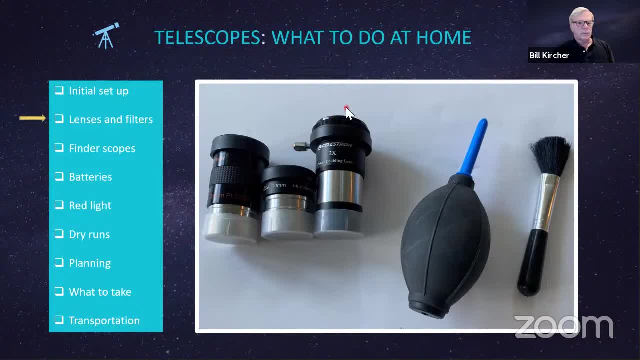 which multiplies the two lenses on the left by a factor of two, You can also get a Barlow that does three. Take your time on this. Magnification is overrated really. There are lots of other things that go into a good, decent viewing image and if you don't have a good image, to start with magnification's. 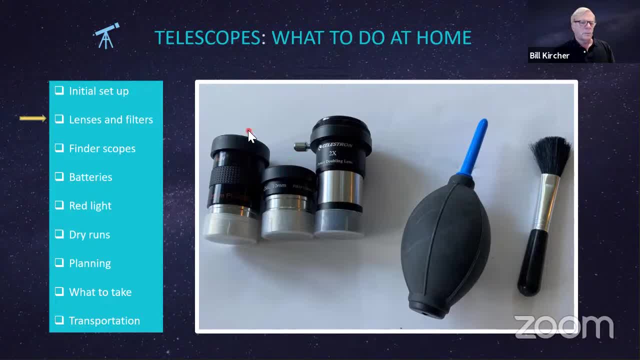 probably not going to help. It's not going to make it better. My advice: if you only have a low power lens, try it out, See how it goes. Then, when you're ready, add to it, maybe with a higher power lens or just a Barlow that will double the magnifying power of the lens you started out with. 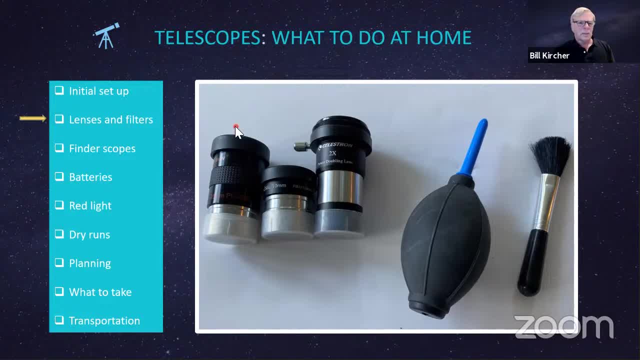 Then proceed from there. I would advise against buying a package of lenses, a set. It would just have lenses in it that you'd probably never use and may not be the highest quality. Lenses are not like eyeglasses. Eyeglasses get smudged- you wash them. Lenses- 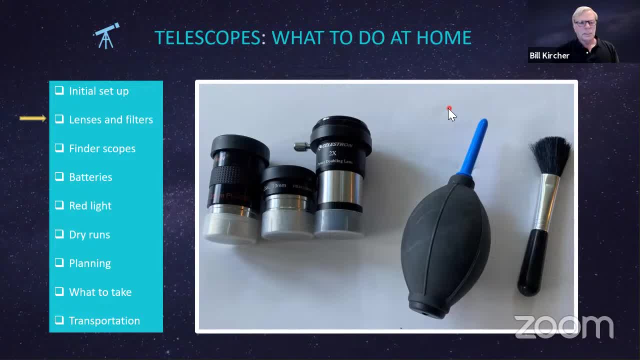 should not be washed. if you can possibly avoid it with any kind of fluid, because they have coatings that can be damaged. If you have lint or dust on the lens, use well. this is a squeeze ball that squeezes air on the lenses to clean them off. You can also 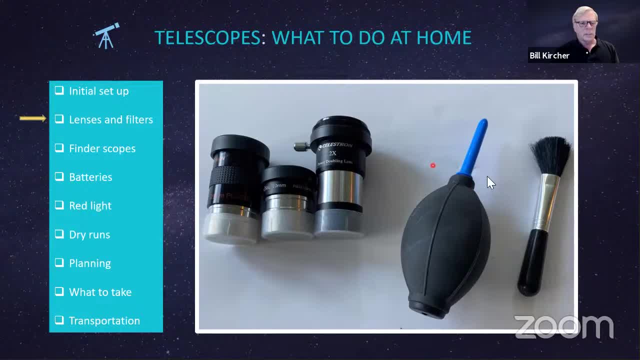 buy cans of compressed air, perhaps at a camera shop, and then a soft brush at the right, Very soft. Keep it clean and that should be all that you use Now. the corollary of this is: try not to put a thumbprint on the glass face of your lens. Handle those lenses carefully. Keep your lens. 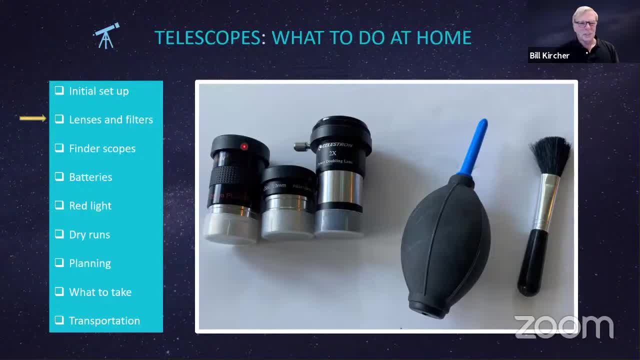 caps on them. Keep track of your lens caps. You could replace them, but it's a hassle. The lens caps also protect them in case they fall from damage. I later bought other lenses, but this is what I started with and it was fine. 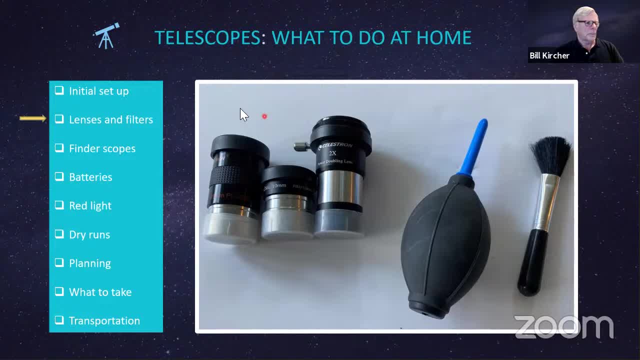 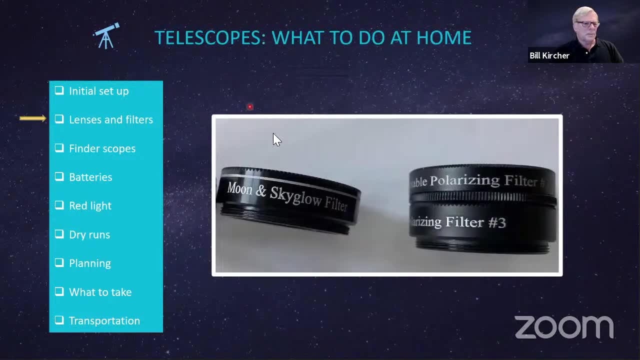 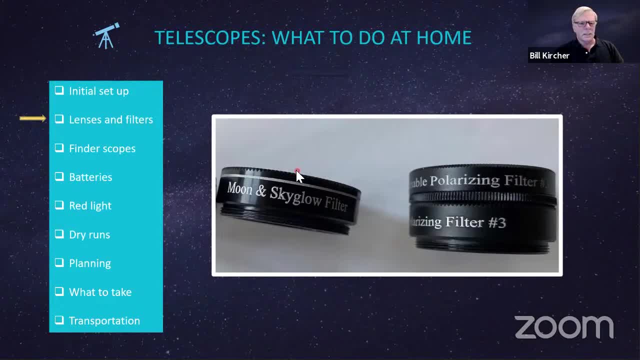 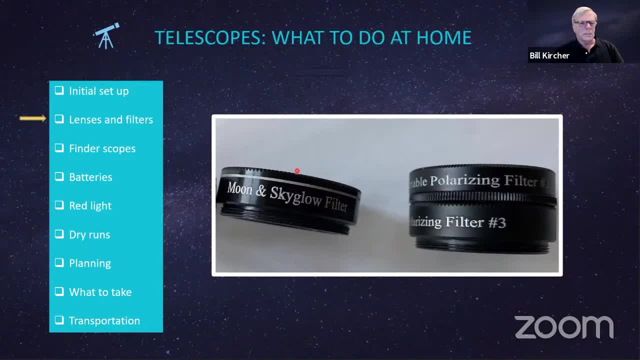 San Francisco where there is a lot of sky, glow and reflected moonlight. It makes the image improves the contrast, makes the background darker. The polarizing filter on the right- this is a variable filter. You don't need a variable filter, but some kind of. some of them are just called moon filters And the moon is so bright. 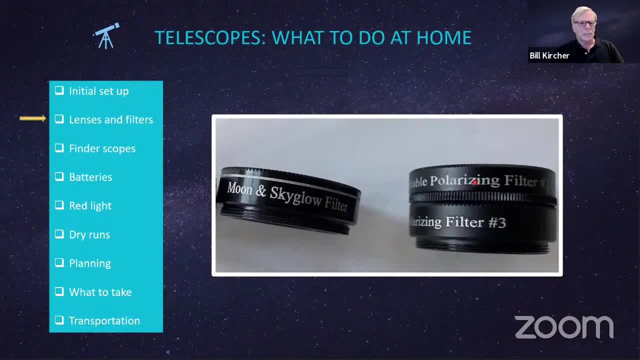 This really improves the observing experience if you're looking at the moon. There are, I think, so many possible filters- perhaps hundreds of them- that you could get Again. I would advise against going out and getting a set of filters. They probably won't be the filters. 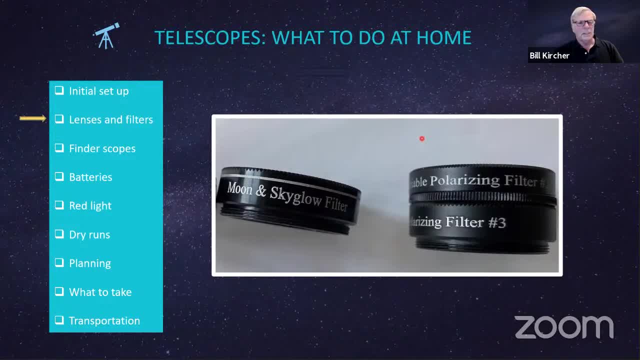 you actually need or want. Maybe one or two of them will be, But again, I would just buy them one by one as you feel a need. If you're looking at Jupiter and you want to make out some more detail and you think a particular filter would help you, fine, buy that filter. 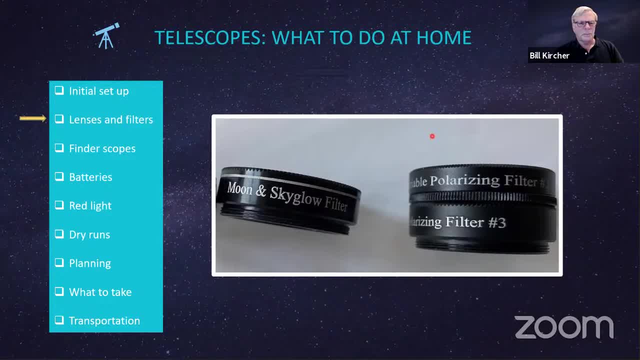 Ditto with Mars, ditto with perhaps a nebula that you want to observe, But do it sort of mindfully and progressively, rather than just going out and buying a set of, say, six colored filters. But that's what I would advise. 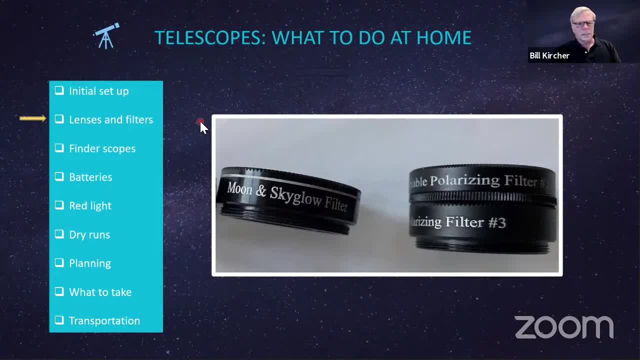 Okay, finder scopes. next subject: Very important, because without the finder, you're really probably not going to see any stars, You're going to see nothing. You're going to see no stars, You're going to see only the colors of the stars going around, People that have a lot of light in common. 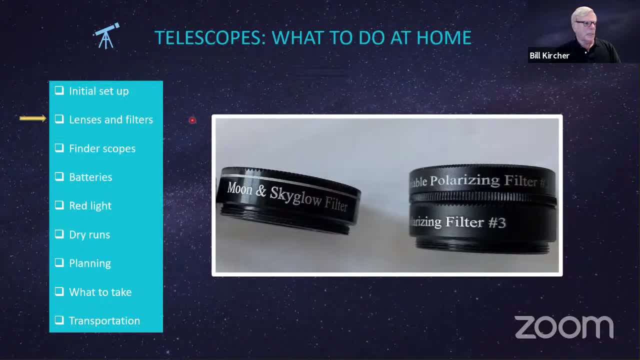 going to see much. Even if you have a go-to telescope that's mechanized and will go to objects, you still need to align it. You still need to find objects to align on stars and center them, And the finder is key to all of that. So let's look at finders. So I have in the next. 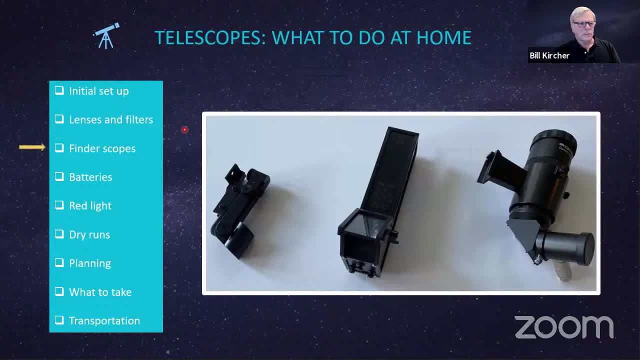 slide. I have three finders. These are my three finders. The one on the left is a red dot finder, what I started out with, what came with my telescope. I ditched it after a while. Actually, it's still around. You'll see it later, repurposed for a different use. Hold that thought. 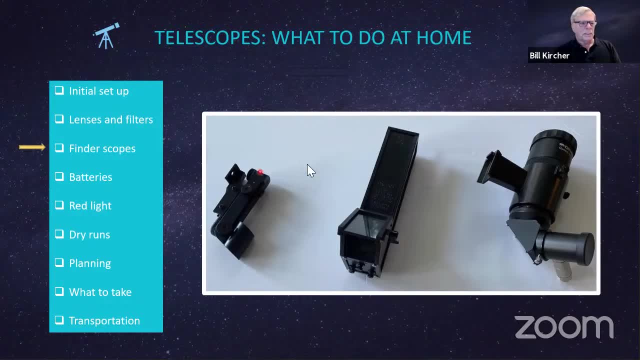 I moved on to a telrad. Both the red dot and the telrad are what is known as reflex finders. They have batteries and LED lights and they project a pattern on a screen. The red dot projects a little red dot, The telrad projects a kind of a bullseye. 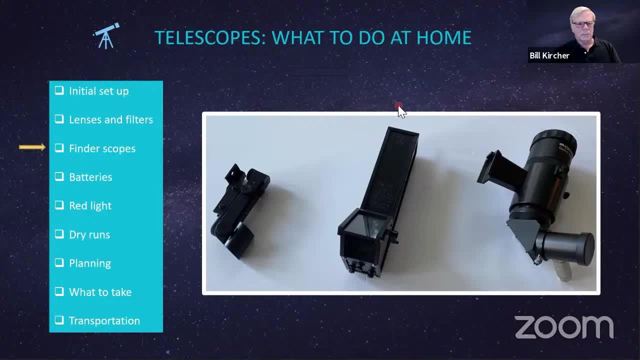 target image. that's very useful, very popular- So popular that star charts and software applications like Stellarium and, I think, SkySafari actually include the telrad reticle so that you can compare what you might see through the telrad. It's kind of bulky and if your 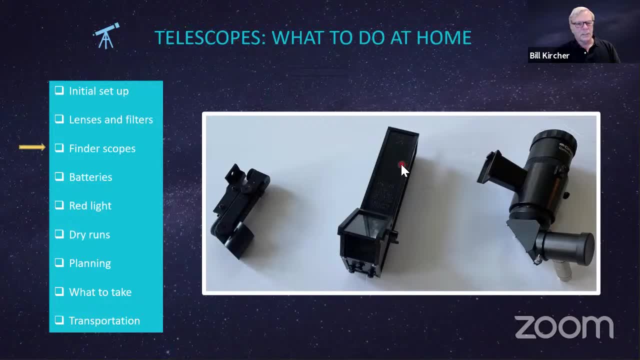 telescope is too small. there is an alternative to this. I highly recommend the telrad. The red dot finder works. It worked for me. It's just not as good as the telrad. And then on the right is a magnified finder known as a. 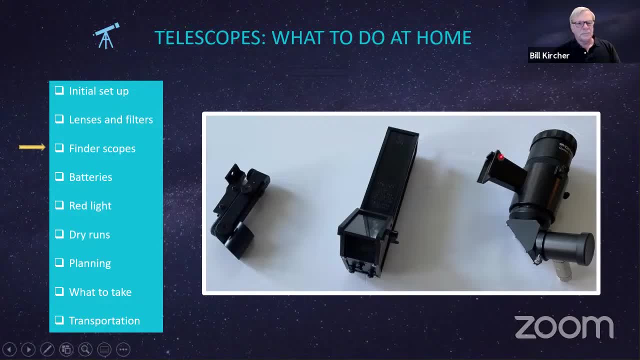 well, I'm not sure how to pronounce it, but it's R-A-C-I finder- right angle corrected image finder that is magnified. Sometimes, when things are magnified, the images are inverted. They might be upside down, They might be a mirror image. This is a true image. 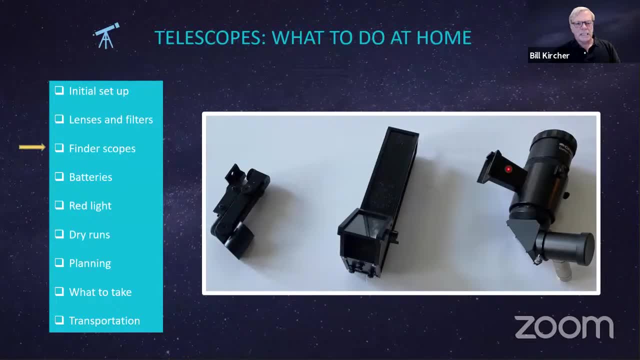 And that's helpful when you're hunting around trying to find something. It's a nine times 50 Orion. The magnification is nine times The aperture is 50 millimeters. It's quite capable and it's about it's well. you might think of it as like half a binocular. 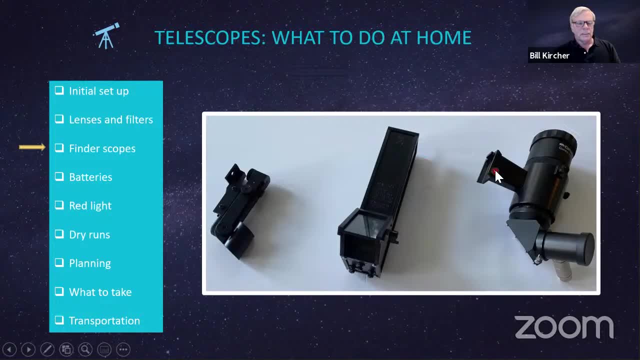 And I use both the, both the telrad and the magnified Find finder, And I'm going to give you a demonstration of that later, how I use the two together to find dim objects. So now let's look at how this is mounted. 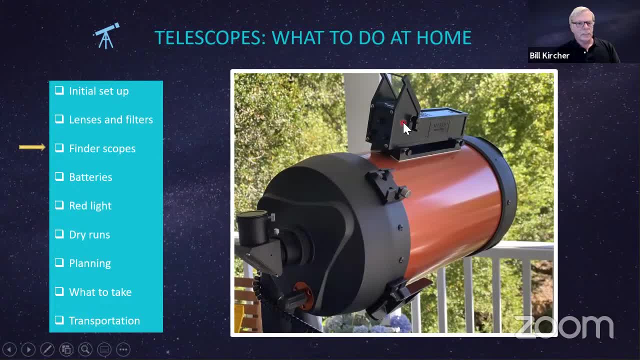 So here is the telescope, my Celestron 8SE, with the telrad on top. mounted on top, It sits in a base and can be removed from that base for portability and then easily reattached. Here over on the right is a handle that turns it on and then increases the. 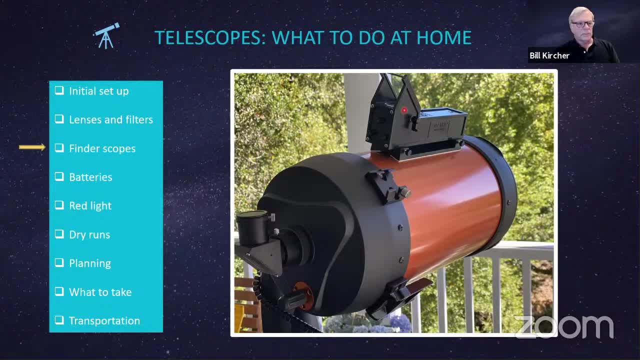 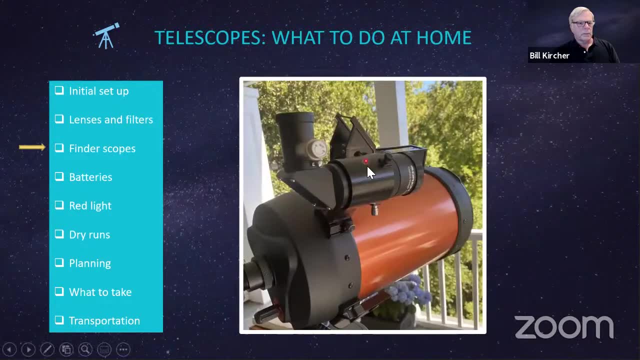 brightness of the bull's eye that you see as needed In the next image. Okay, now here is the Orion magnified finder in the foreground, also mounted with the telrad in the back. Next slide is the rear view. Okay, Okay. 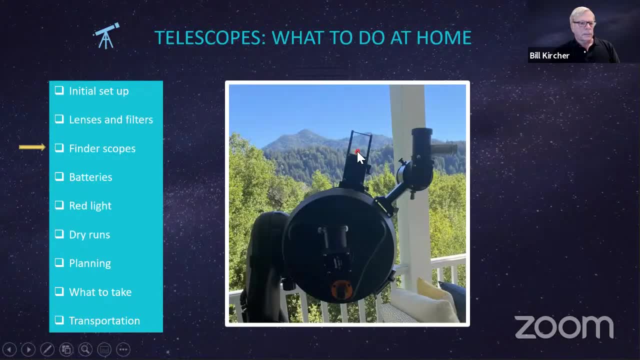 Okay, Okay, Okay, Okay, Okay, Telrad, and to the right of it the Orion Magnified. I have the Telrad slightly off center to leave space on the left so I can mount a camera, a small camera, which I do occasionally. 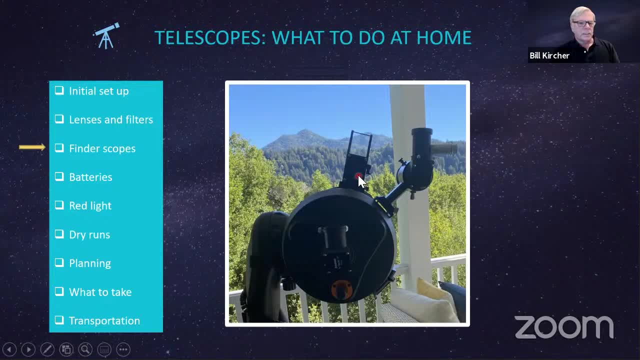 Not shown here. obviously The Telrad could be mounted anywhere, because the base attaches with adhesive tape, and so it can be moved. If you don't like your mounting, you need to adjust it. The other finder needs a mounting bracket. It needs to be screwed in somewhere so you have fewer. 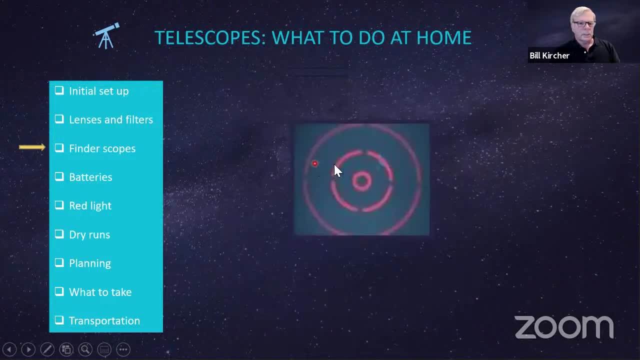 choices. So here is the bullseye, This is what you're going to see, the reticle, Three concentric rings with little spaces in them, and the goal is to have the center bullseye over the object that you want to observe. but you can use the other concentric rings too. And again, 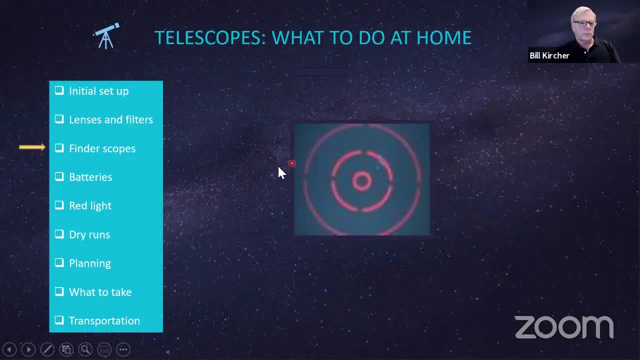 I'll demonstrate, I'll show you how to do that. Very good for star hopping. So sometimes telescopes come with really cheap, useless finders. Again, I wouldn't be in a hurry. Try to use it if you can, but consider an upgrade down the line. 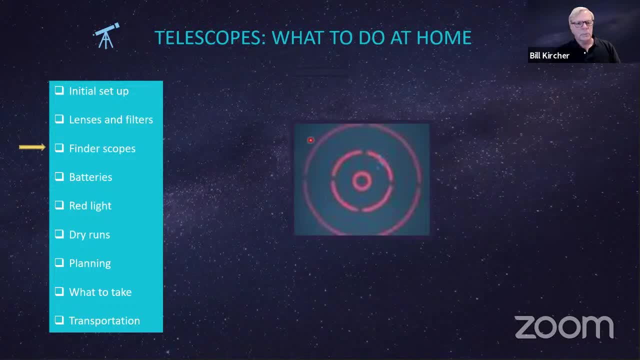 Maybe something like the Telrad would be your first upgrade, and then maybe you go for a magnified finder too. Wait as long as you can. a consideration, Cost is a consideration. They're not really expensive, but I would just take it. 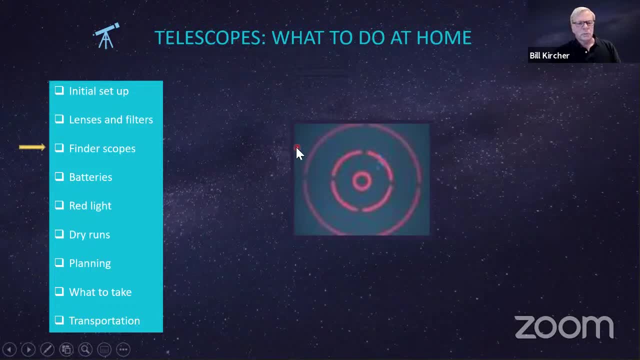 step by step. The main thing is: you do want to be able to find objects, and if you can't find objects, then that's an issue that does need to be addressed as a priority. Okay, batteries Only relevant if you have a mechanized telescope that runs off of external 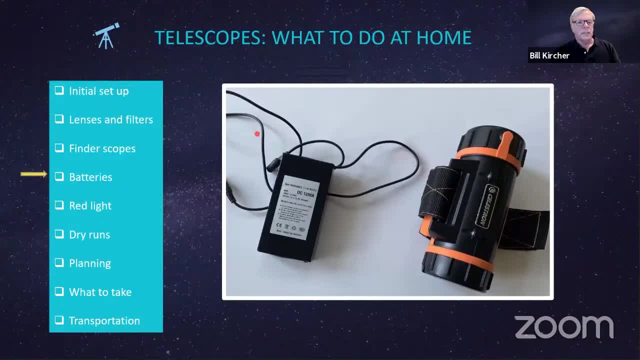 battery power. Some of the motorized telescopes have their own internal batteries that are charged in a manner similar to well charging a cell phone: You just plug it in and it eventually charges. I have an EV scope that is charged in that fashion. It does not need an external battery. 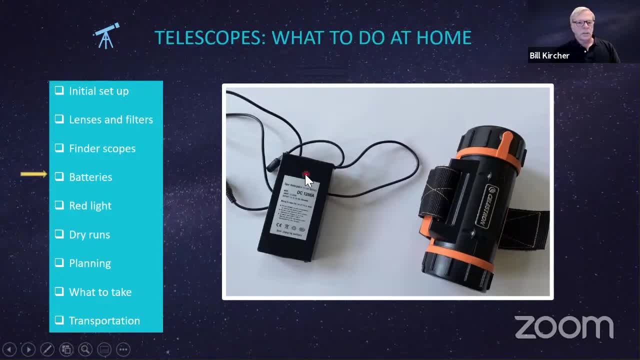 but the 8SE does. I started out with a smaller battery on the left. It was fine. After I added an astroimaging camera I thought I might need a little more power, so I got from Celestron the battery on the right. 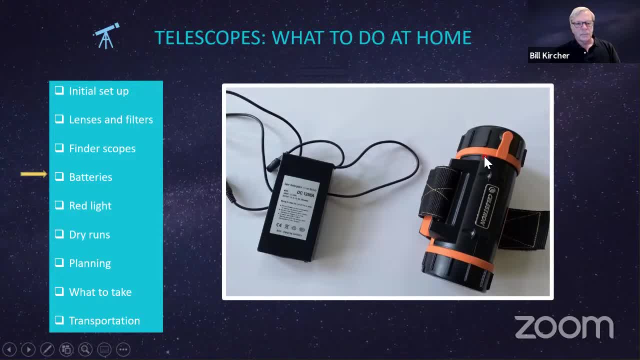 Good, capable battery, plenty of capacity, doubles as a light, has a port for charging another device like a cell phone or an iPad, and it has a Velcro strap so I can attach it to the tripod, which is an advantage. It puts it up where I can get to it and keeps the cord out of the way. 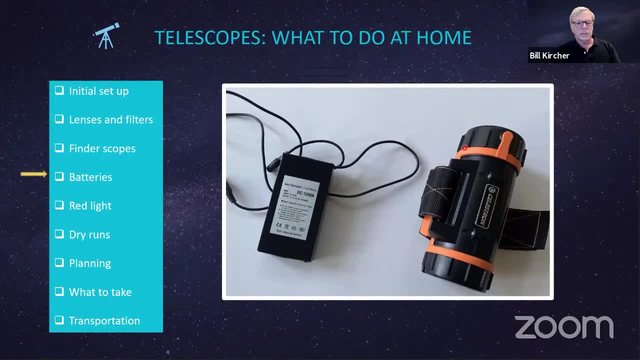 But many people use external batteries. I have battery packs that sit on the ground. They have a higher capacity and they are very popular as well. So, whatever you do, make sure you have a battery. Celestron wants you to install AA batteries- I think something like 12 of them for my telescope- and they don't last very long. 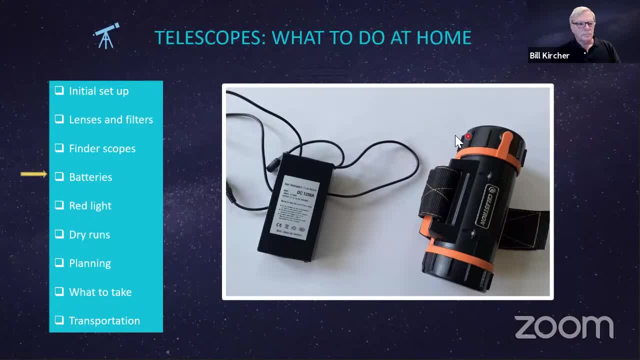 So you will need an external battery. So I would prioritize that, If possible before your first star party. if you have a mechanized telescope, If not, if it's manual, then you can skip this step. or if you have an internal battery, no issue. 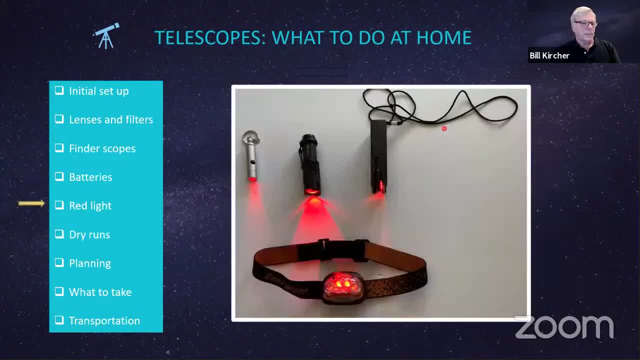 Red lights very important. White lights are frowned upon and worse at star parties because white light destroys your night vision. Red lights are better, although it's possible for a red light to be too bright too. Here's three choices. The one on the left is small. I think it's made by Orion. It can fit on. 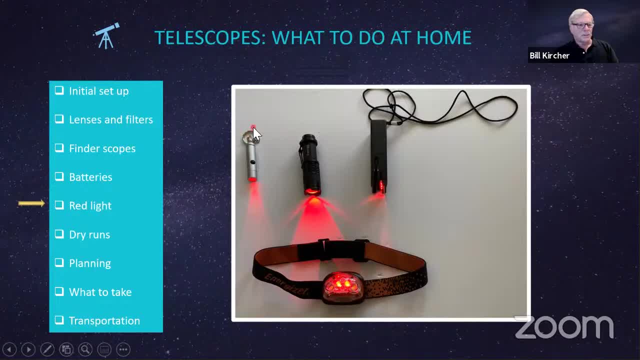 your key chain, which is an advantage, unless you're prone to lose your keys too. But it's really an embarrassing, humiliating situation to be at a star party and not able to find any red lights. Then you're in a position of needing a red light so you can find your red light. 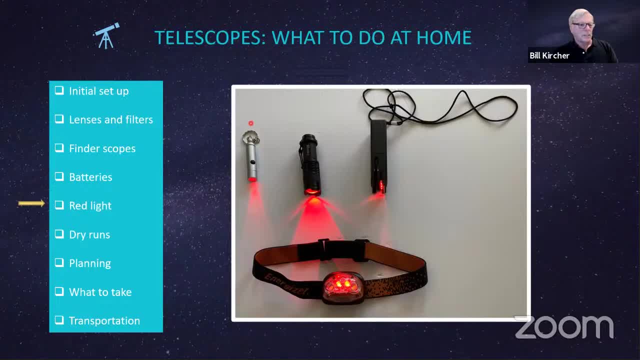 meaning you're probably going to ask for some help. So I have a couple of them. I always have an extra, But this little one on the left- if I can't find any other red light there, it is- The one in the middle has a more powerful beam. The one on the right is adjustable. 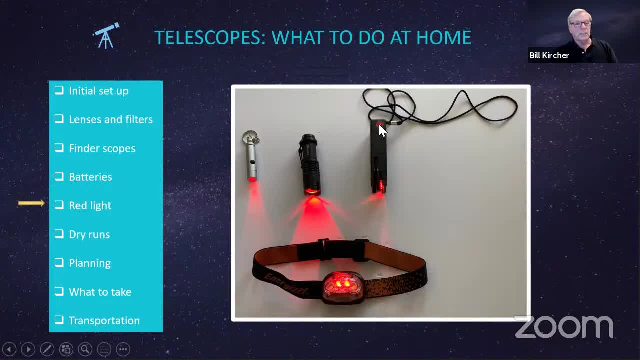 I'm actually missing part of it. It has a lens on the front of it, But this is very nice because you can dim it if you want, And it has a lanyard so you can wear it around your neck, which makes it harder to lose, but not impossible to lose. And then the headband. 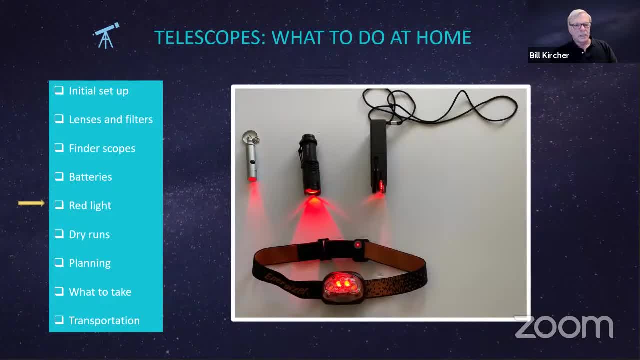 you can buy these at a hardware store, at a place like REI. One problem with them is they cycle between red and white, So to turn it off you're going to have to cycle through the white lights or just leave it on. But of course this is handy if you're setting up your telescope. You want to be hands-free. 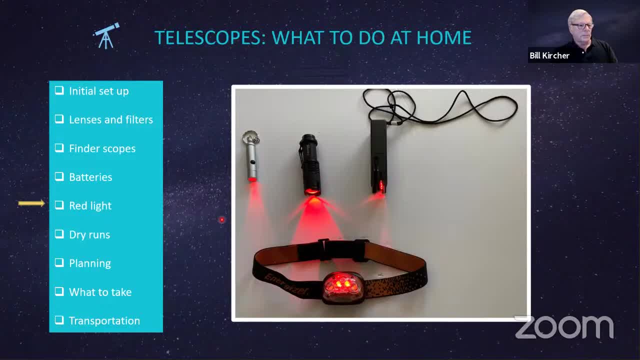 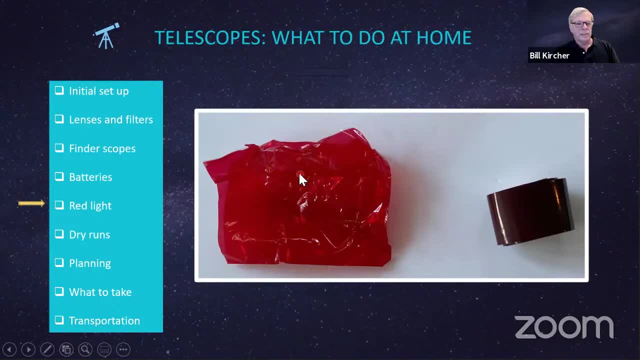 On the subject of red lights, here's my kind of backup. On the left: cellophane, red cellophane. Put it over a conventional flashlight with a rubber band. Now you have a red light. On the right is tape. It's taillight repair tape. You can buy it at an auto supply store. 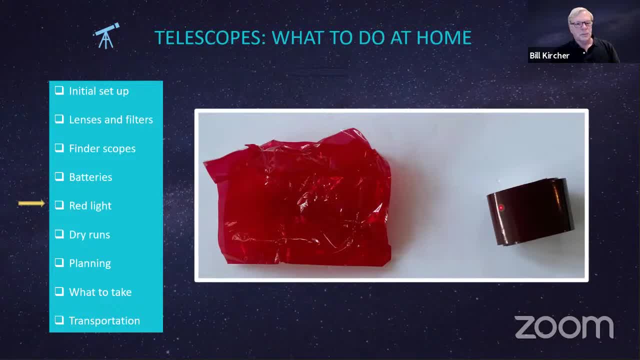 And it comes in very handy, and I will show you just why in a later portion of this program. So I keep this with my accessories and a small pair of scissors, because I almost always use this Red tape, auto supply store taillight repair tape. Okay, now here's another thing I suggest you do. If you have time, Do some dry runs at home. You set your telescope up, maybe after you set it up or maybe independently. if you need more time, I would suggest doing some dry runs during daylight. You won't be able to see any stars. I mean, you might be able to see the moon outside, but you won't be able to see. 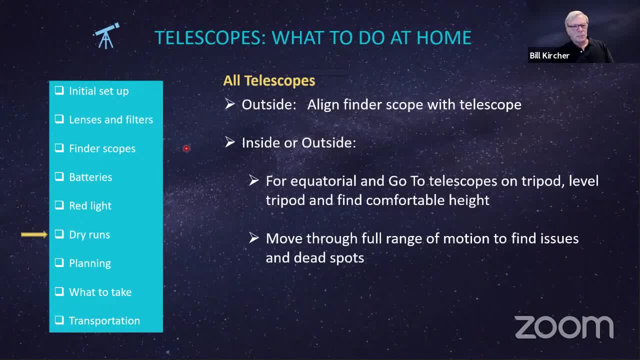 anything else, Of course, the sun will be up. Stay away from the sun, obviously. What you can do outside with any type of telescope is align your finder scope to the telescope. Find a distant object that you still can see through both the main telescope and the 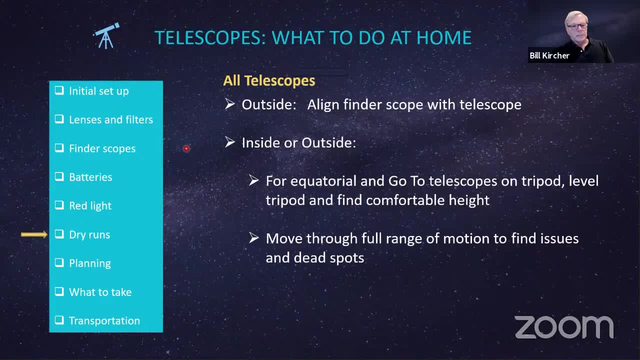 finder scope and center it in your. and something easy to recognize: center the object in the lens- low-power lens- of your telescope and then look through the finder. Is it centered? If not, there are adjusting screws. Adjust those screws so that it's also centered in the finder. and now 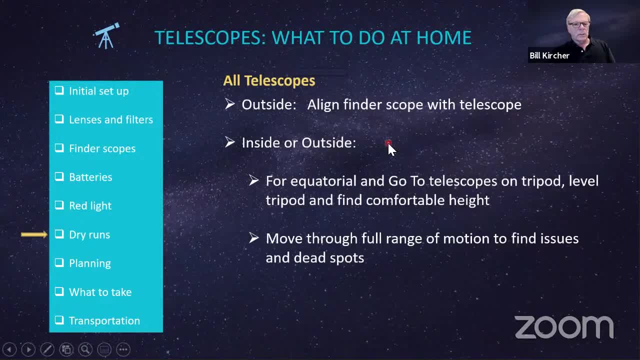 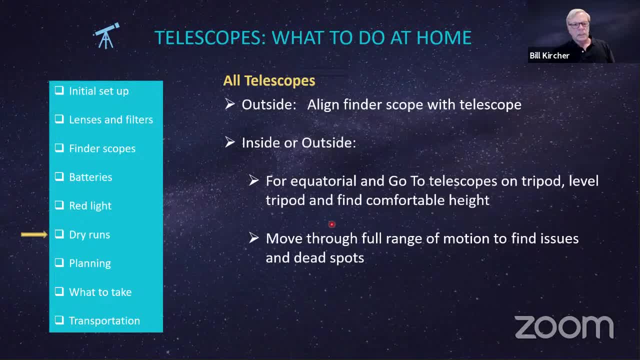 the right height so it's comfortable to view through the lens of your telescope. The fact is telescope if you have a Wi-Fi connection and use an app like Sky Portal with a Celestron Practice moving the telescope around with a controller. There are different speeds. 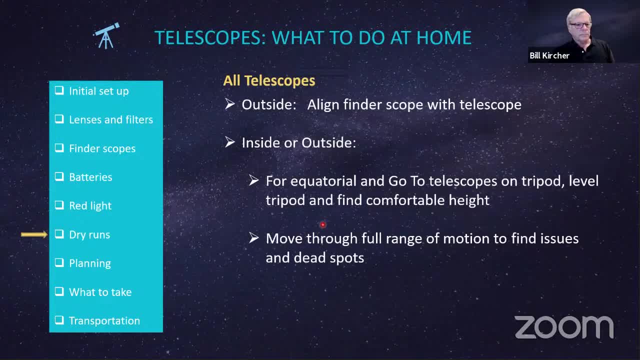 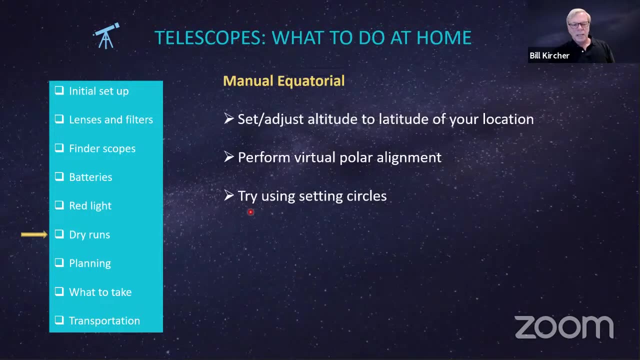 When you get close to the object, you use a slower speed. That's the minimum I would do, but you can go a few steps further. So let's explore that. So, with the equatorial mount — this is a manual equatorial mount — if you haven't, 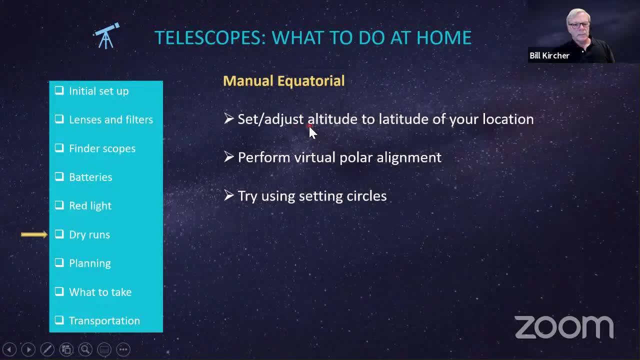 already done so. adjust the polar axis to correspond to your latitude In the San Francisco Bay Area. it's about 38 degrees, and that's an adjustment that will stay until you within for 30 minutes. There are a couple of steps that you can do So. first, adjust the polar axis to correspond to your latitude In the San Francisco Bay Area. it's about 38 degrees, And that's an adjustment that will stay until you. 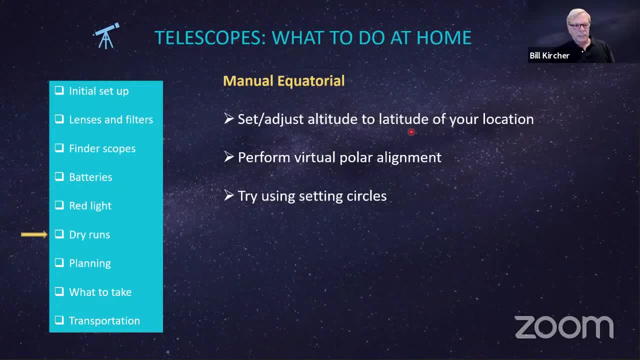 move the telescope to a location that has a different latitude, And then I would perform a virtual polar alignment. You can't see Polaris, but you can pretend, And once you do that, then you can. if you want, try using the setting circles Now. 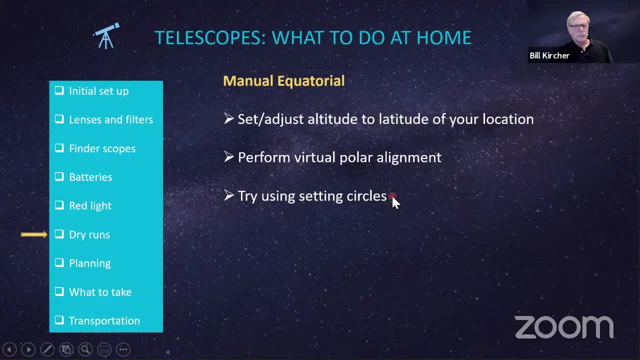 that's a topic I'm really not going to have time to go into. If you do decide to try it, then you'll need to use a manual or a book or something online. There's lots of material online about how to do this. Some people think using setting circles is a help to locate objects. 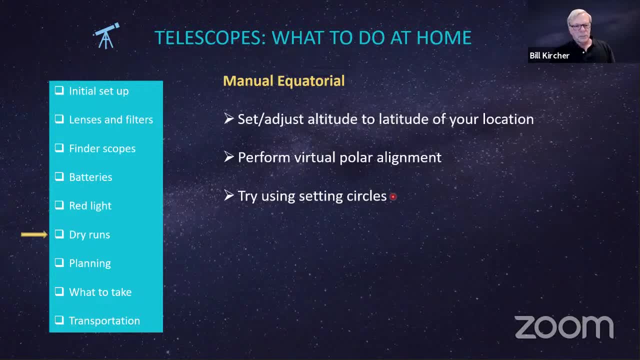 Other people would say not that much of a help because the setting circles on these telescopes tend to be fairly small and fairly approximate, But it's something you could at least try. once I owned an equatorial mount telescope manual- equatorial mount. 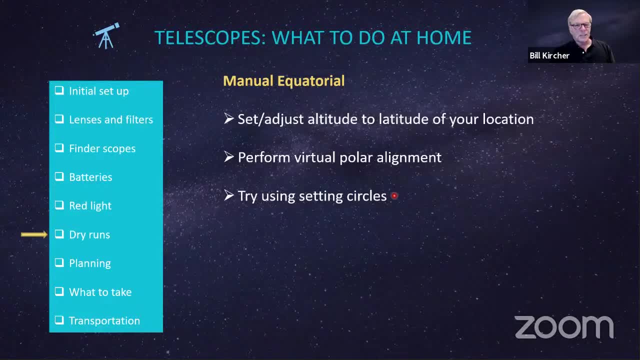 telescope for quite a while and actually never once used the setting circles. But don't let that discourage you: In those days we didn't have YouTube videos, So perhaps if I could have resorted to these other materials, I would have tried it. But I would at least take the step of 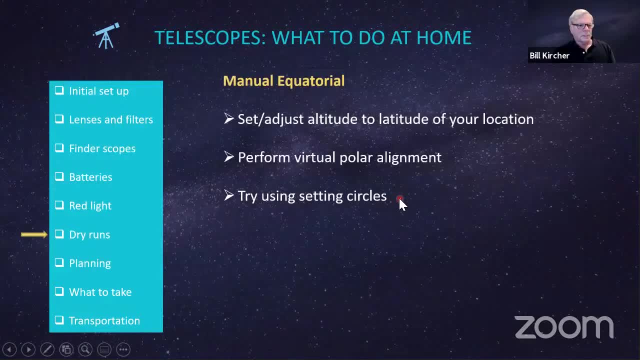 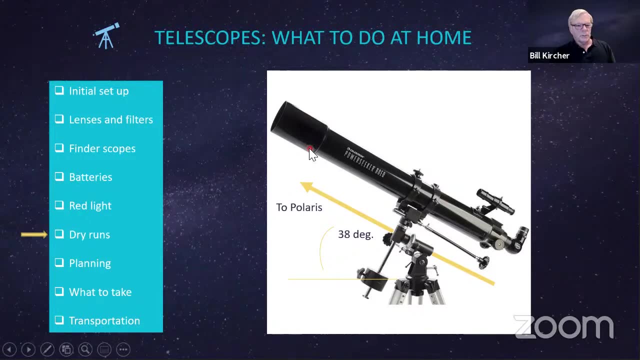 just getting your feet wet with a polar alignment, Okay. So how would you do that? Well, aim the telescope to the north, to true north, because that's the first step in your alignment. Make sure you do have the 38 degree angle if you're in the Bay Area, If you're 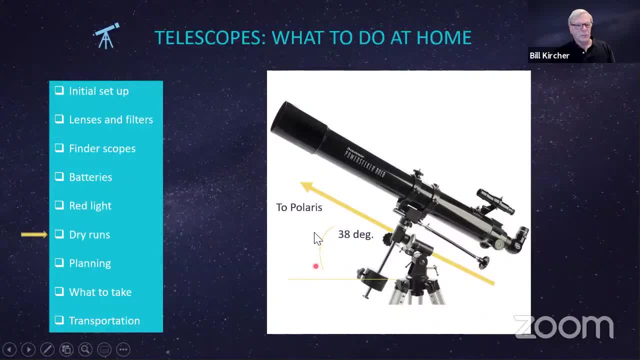 in a different area, then you need to figure out what your latitude is here And then pretend like, once you have this aimed north, like you're going to look through the telescope at Polaris, with the telescope in the home position. This is the home position depicted here. Telescope is: 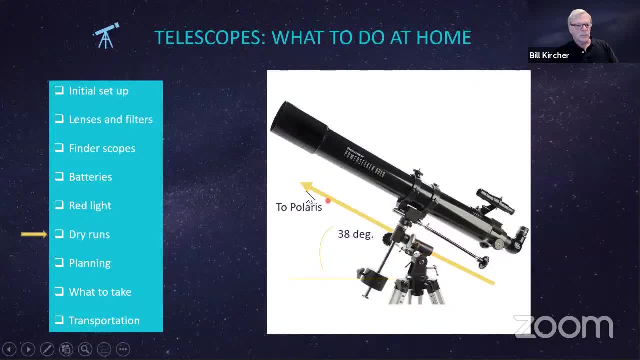 directly above the polar axis, Which is the yellowish gold arrow here. Directly above it, not to one side, not turned one way or another. Directly straight above it, With the counterweight straight down. So that'll always be the way that you'll have the telescope when you align it. Now, speaking of north, did you know? 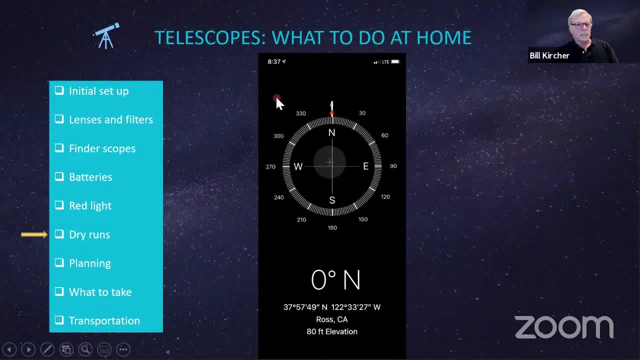 that- and this is a screenshot of an iPhone- it has a better view of the telescope than the telescope. It has a built-in compass under utilities that will show you which way north is, And it will also tell you, of course, what your latitude and longitude are- Information that could be useful. 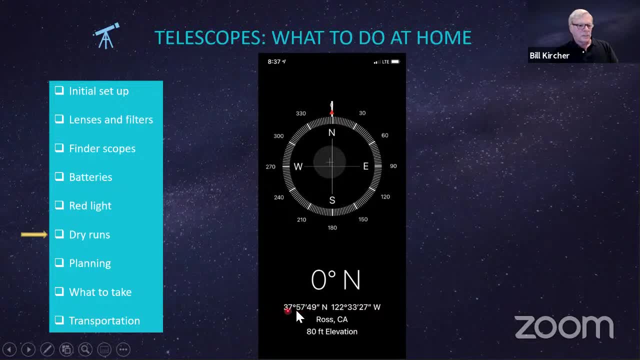 in setting up your go-to telescope. And here's the roughly 38 degrees, 37 degrees, 57 minutes that I referred to as the latitude in the San Francisco Bay Area. The iPhone can also be used to level your telescope. See this tiny little plus sign. 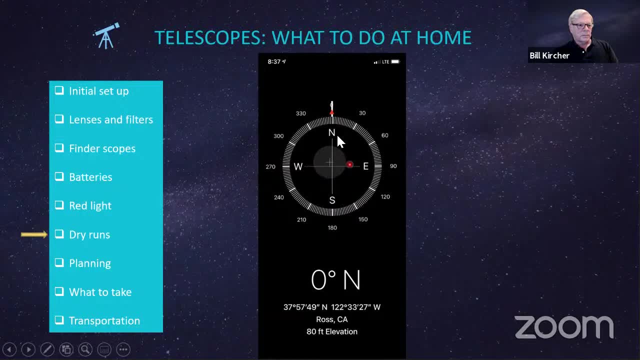 In the middle And then a larger plus connecting the north, south, east, west. This is intentionally not level. I wanted to show you how. if it's not level, the small plus sign in the middle is off-center. But if you align these to all of these lines, align it perfectly. 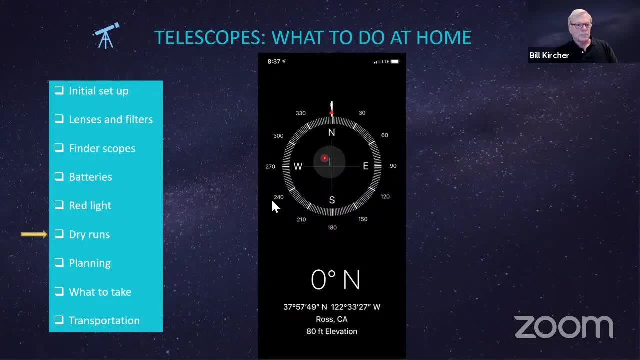 then it will be level, So you can use this to level your tripod. I'm not familiar with Android phones. I would imagine there's something similar or you can get an app that will help you with that. I think I mentioned equatorial mounts and 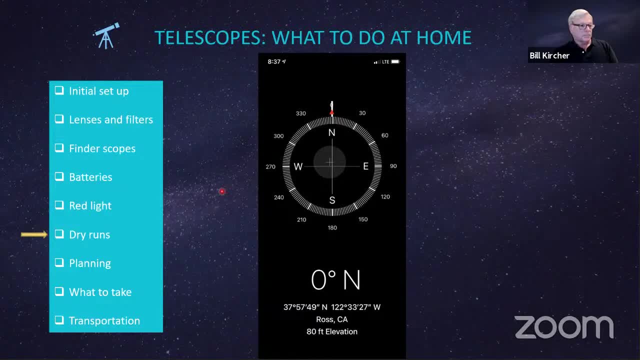 go-to mounts should be leveled And actually any telescope should be at least approximately level to increase the ease of using it. But critical if you have a 6.5 or a 5.9 is just an equatorial mount that you expect to track accurately. 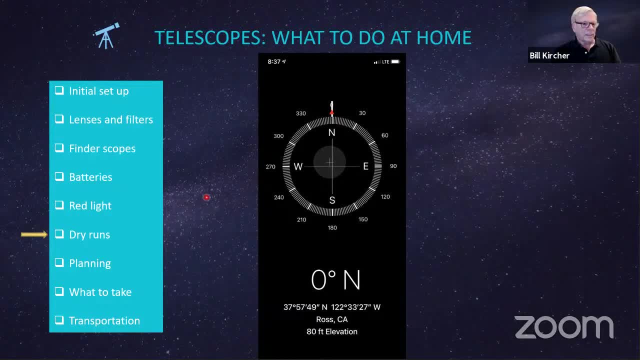 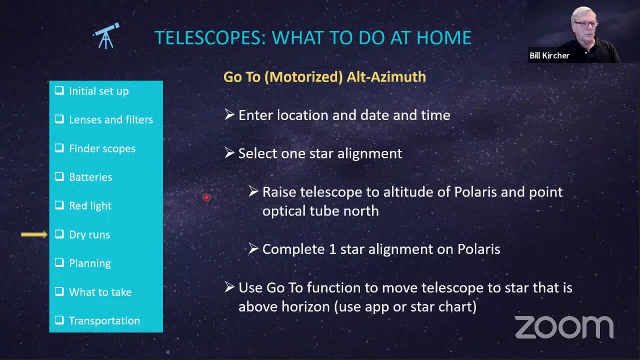 Okay, Planning is the next subject. You don't have to plan, You can just show up in the mountain, but you will improve your experience if you do that. I'm sorry I went on to the next subject I forgot. I think we have enough time to do this. The next slide covers using your go-to mount to 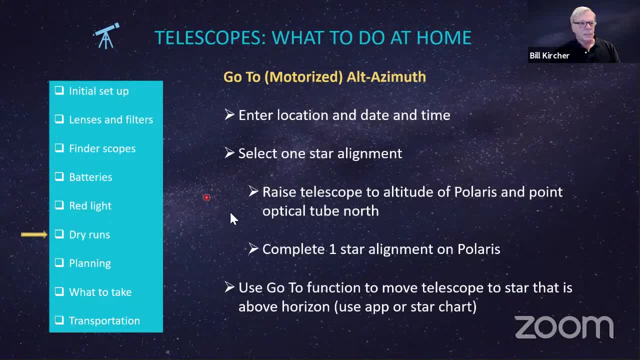 practice with it. The next slide covers using your go-to mount to practice with it. The next slide covers, now i've set this up to to be an alignment of a celestron se series mechanized go-to telescope. i think mead is similar, but you might have to tweak this a bit for me and it's an alt azimuth. 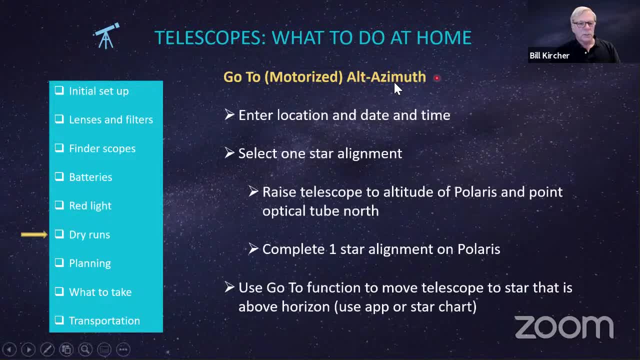 mount. i think this would work on an equatorial mount, that is is also a go-to mount, mechanized go-to mount, but you might have to tweak it a little more. so the idea is you're going to do what we call a one star alignment, and that one star is polaris. 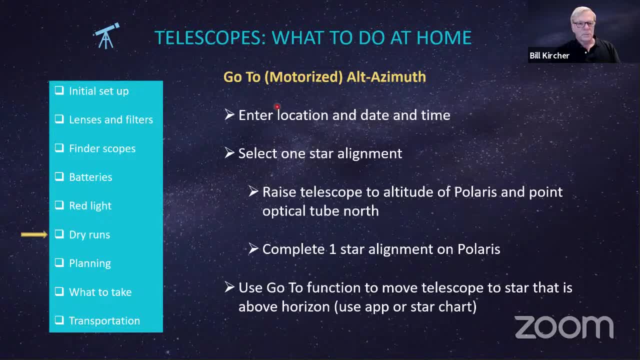 so you can do this in your living room. turn on the telescope it. when you start the align sequence, it will prompt you to enter your location and the date and time. if you've already entered the location previously and it's still accurate, then you don't need to change that. it will remember the location, but not the date and time. 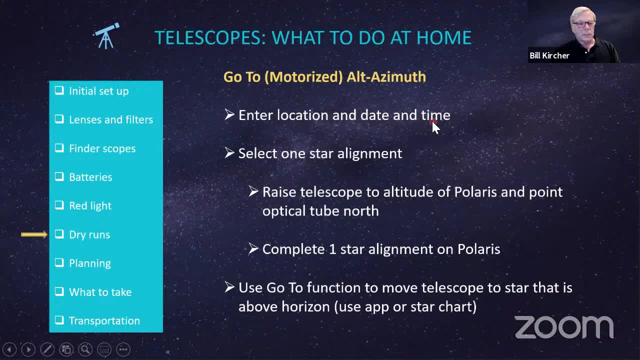 so enter the date and enter the time in 24 hour format. choose the pacific time zone- daylight savings time now, and every time you turn on the telescope you'll have to repeat the date and time. if you have a gps module and you're outside, you will probably acquire the location, date and time independently, but we're not. 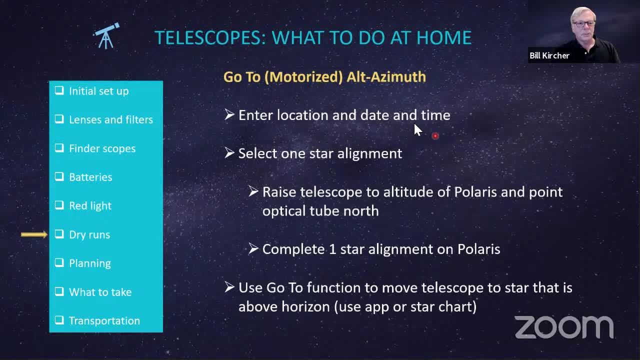 outside and my gps module doesn't work very well, so i i just do it. i put the date and time in um and then select from the menu one star alignment. you'll have a choice of one star, two stars or three stars. i choose one star. aim the telescope north, to true north. 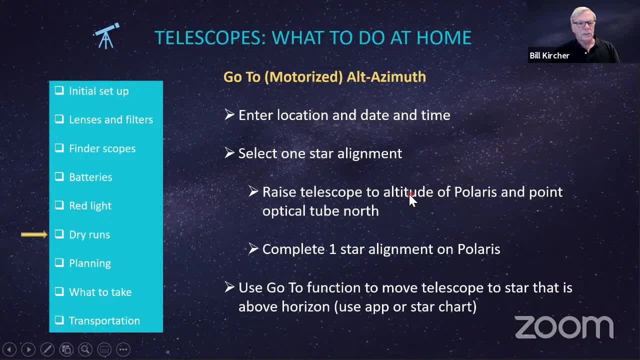 raise the telescope so the other side of the telescope is on the other side of the telescope the optical tube is at that 38 degree height. just you know guesstimate it. you can't see polaris, you don't really have to measure. just sort of guess what. 38 degrees would be somewhat less than 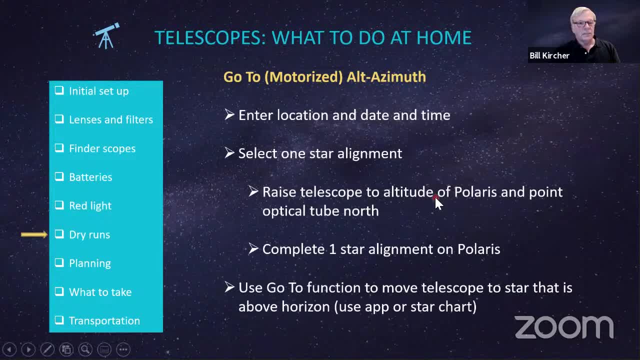 45 degrees um. but if you want, there is a menu item where you can get a readout of your altitude, of your optical tube, and if it confirms that you're at 38 degrees, well, even better, and then align the telescope. you're now aligned on polaris and polaris is always there, it doesn't move. that's why we use 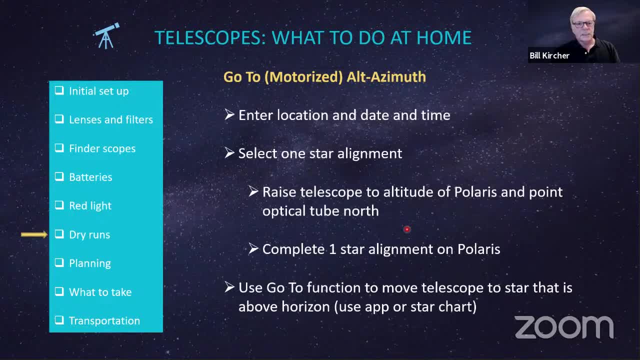 it. it's at the celestial pole and, um, you're good, now perform a go-to, tell it to go to a star that you know is up, even though you can't see it because it's daylight and also because you're in your living room. pick one today. i looked at my planosphere and i picked capella, a very bright star. 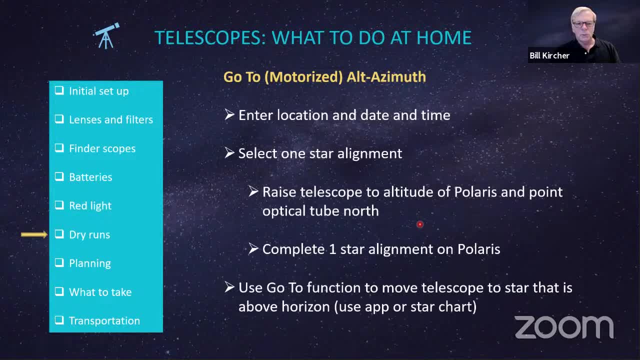 uh, so tell your telescope to go to capella. if it won't do that, there's a problem. you may need to backtrack what is the problem. or if it moves, but it doesn't move to where you think capella should be, looking at your planosphere, there's a problem. maybe something wasn't entered right, maybe something. 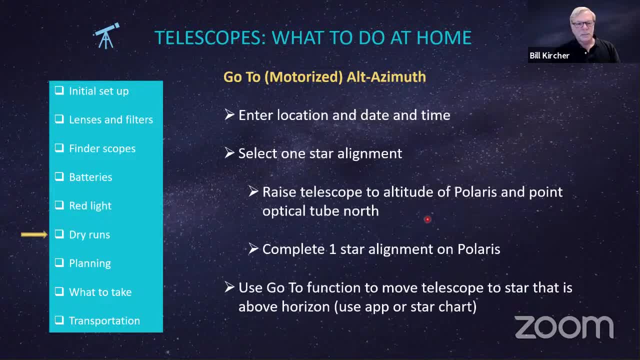 with the date and time. much better to to resolve these issues in your living room than in the dark on mount tan, where you will be frustrated and waste a lot of time potentially. um, and so you. you can repeat this as many times as you want, as long as the object is up above you. 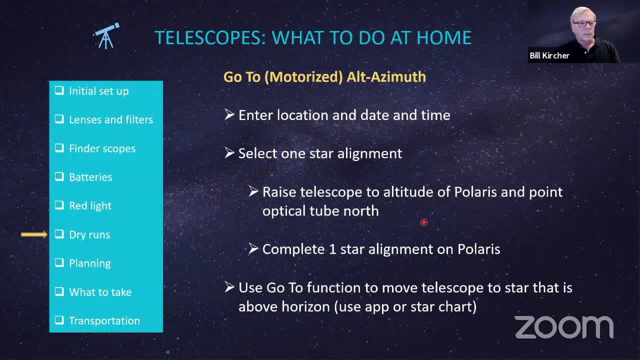 at that time of day during the daytime. i highly recommend this. um, it takes a while to get comfortable- comfortable with the sequence that you need to go through to align your telescope so that it will go to objects all right. now on to planning. this is another thing that i recommend. 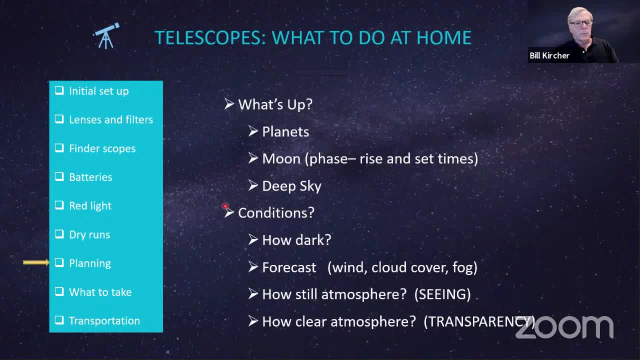 you do do some planning before a star party, and you can do this closer to the date of the star party. check out what's up there on that particular night, the planets maybe. i think this time of year jupiter and saturn are up. uh, when do they rise? when do they set? what constellations will they? 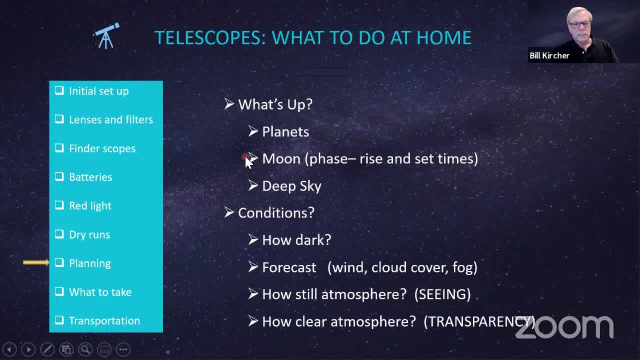 be found in the moon. we try to time our star parties to coincide with the new moon and the moon, but moon phases and rise and set times are relevant, among other things. the moon is bright and so it won't be all that dark if a full moon is up. 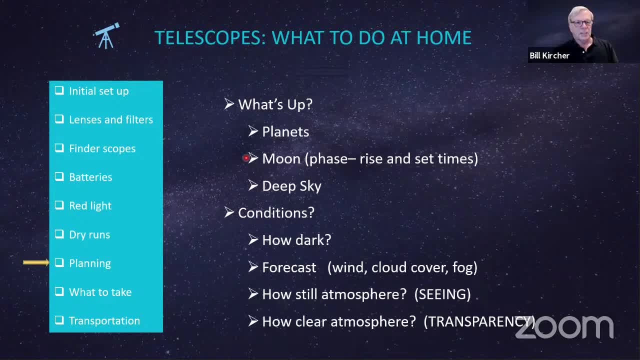 and maybe you want to then say, okay, i'll look at the moon. um, it's, it's, it's, it's. it's a matter really of prioritizing what you're going to do, based on what's going on and what the conditions are, and you need to have a or you, you eventually will, i think, find you have a kind of a a need at. 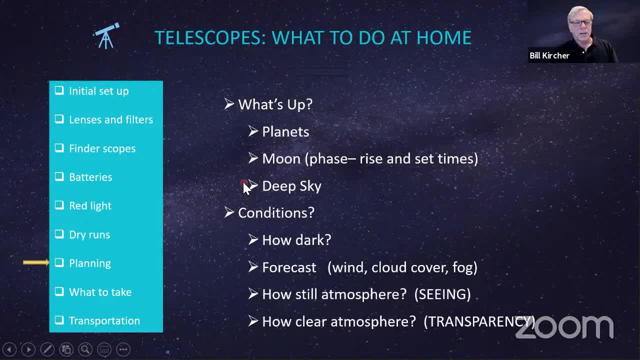 least a for some sort of a loose plan that prioritizes objects. you're going to start with the planets, then you, if you have time, you'll move on to something else. but if the fog comes in, then well, actually, if the fog comes in and it's overhead, that may be the end of the star party. but 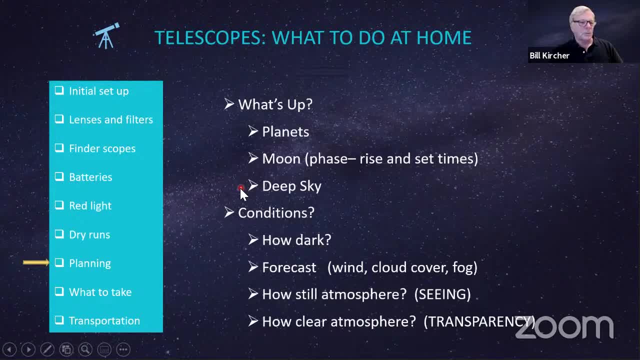 anyway, i won't go on, i won't belabor this, but you know, have have some, have some flexibility is what i'm saying, because conditions may turn out to be different than you think they will be, or they can change. so let's talk about conditions. how dark will it be? well, as i mentioned, if the moon is up. 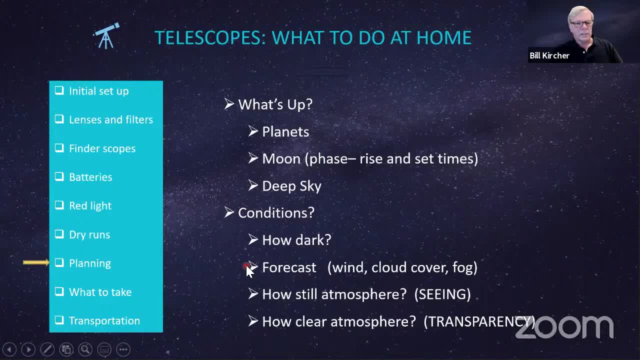 not that dark. uh, if the air is not very clear, it can reflect ambient light from san francisco. how still is the atmosphere? we call this seeing, if the, if it's relatively still, that's a good chance, a good opportunity to see planets If there's. 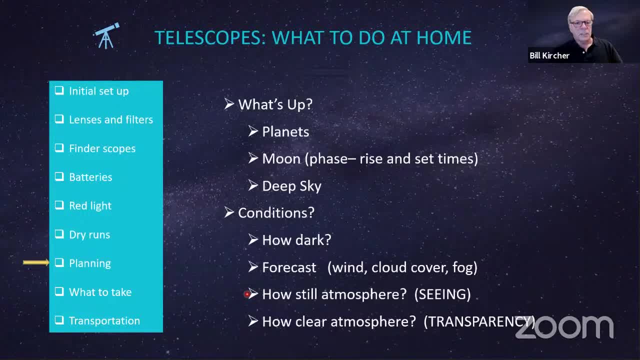 turbulence. the planets may not be very clear, You may not be able to see much detail, But if it's dark and the air is clear, that would be a good situation for viewing faint objects, maybe galaxies or nebula. The clearness of the atmosphere we call transparency. 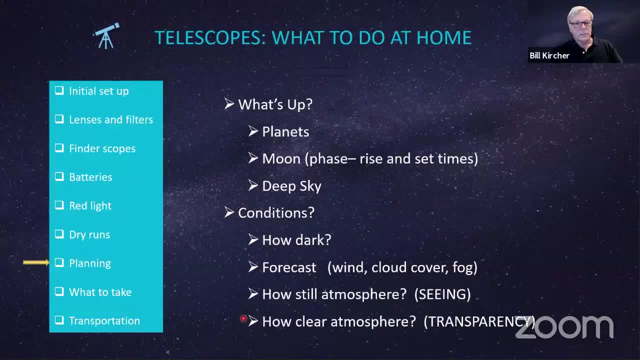 And it depends on pollution: dust, smoke, unfortunately- and water vapor in the air. So I usually try to have sort of a list, just as a rough list, maybe 10 items on it that I might want to look at If I want to observe deep sky. I'll try to find objects that are good this time of year. 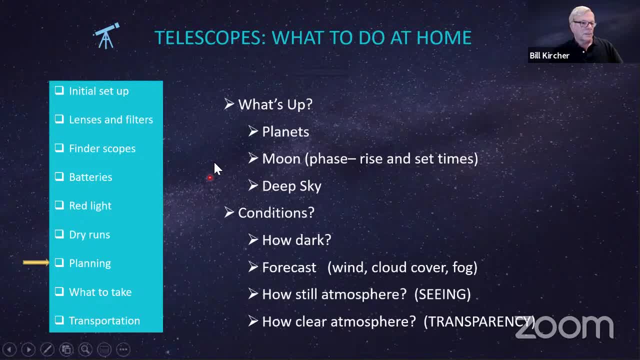 they're bright. Okay, so a list? I seldom get through my whole list. Maybe I'll only get through three or four items, or five items, And you're wasting your time. if you have 20 items. You're never going to get through all of them. 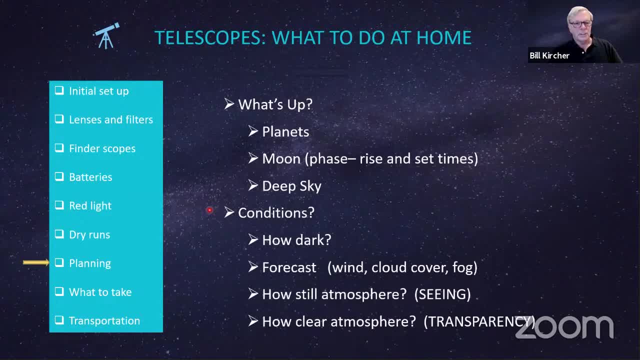 You're never going to get through all of them. You're never going to get through all of them. You're never going to cover that, even if you stay all night, unless you're a very skilled astronomer and everything goes just right. 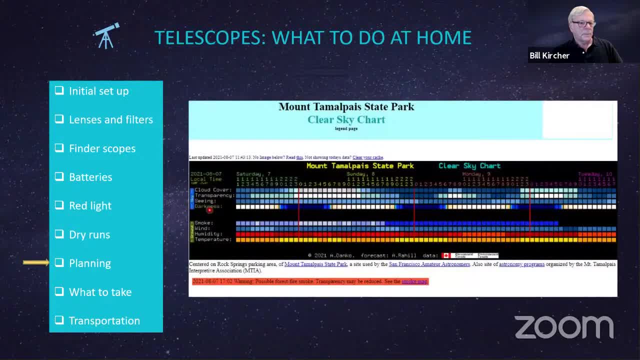 Okay. so the next slide shows the clear sky chart that you can access through our website. Go to stargazing tools. And this is a prediction. It's only a prediction of what the seeing conditions will be. cloud cover transparency. I did this screenshot on the. 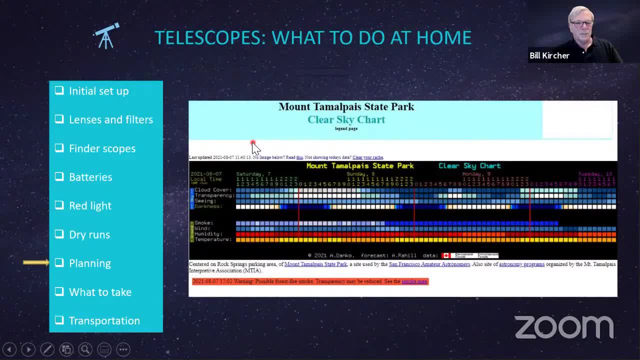 date of our last star party, And if you relied only on this, you might not have gone to the star party. As it turned out, I couldn't go, But those who did go said it was good. It was a good experience, Notwithstanding smoke, possible cloud cover, etc. So use this to plan, but don't make 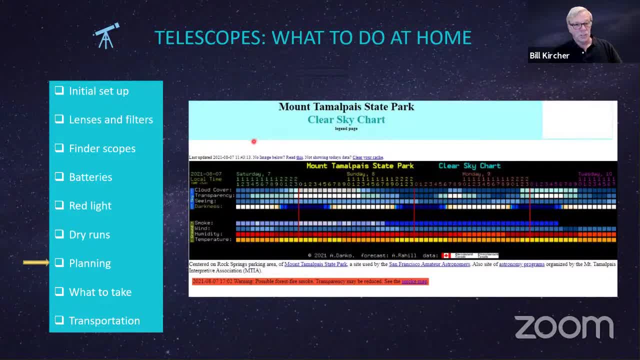 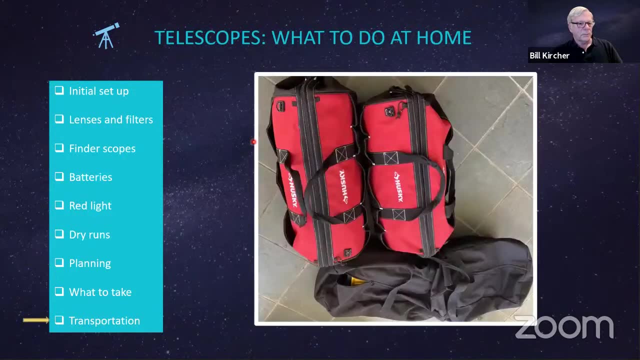 your decision as to whether you're going to go just based on this. It's just a prediction And this can change, and change quickly. What to take. Okay, everything we've talked about so far- lenses, red lights and so forth- But don't forget- Sorry, this is jumping around a little bit, Okay, don't. 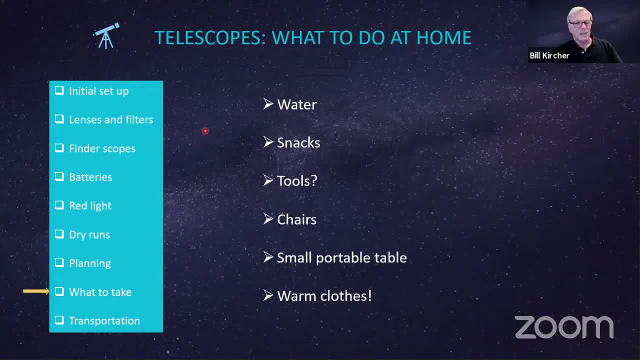 forget Snacks, water. My wife and I- it had been so long since we've been to a star party- we didn't bring these items. We were very thirsty and quite hungry. Tools: I usually bring a Phillips screwdriver. Maybe you'll bring some tools if you need them for collimation Chairs, something. 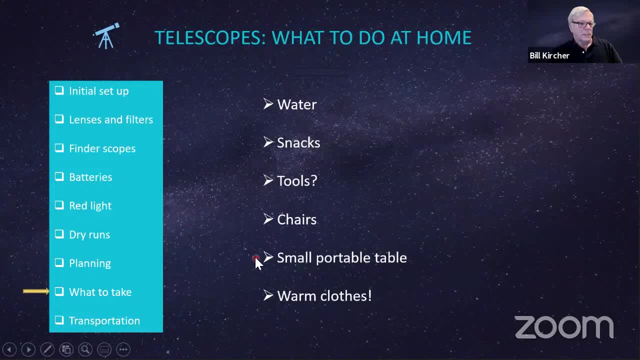 to sit in, Otherwise you'll be sitting in your car. A small portable table- Essential if you have a telescope that rests on a table, but otherwise very handy. Always bring warm clothes, even if it's hot out. You never know, If it's cold, it can get really cold In the winter. I would dress as: 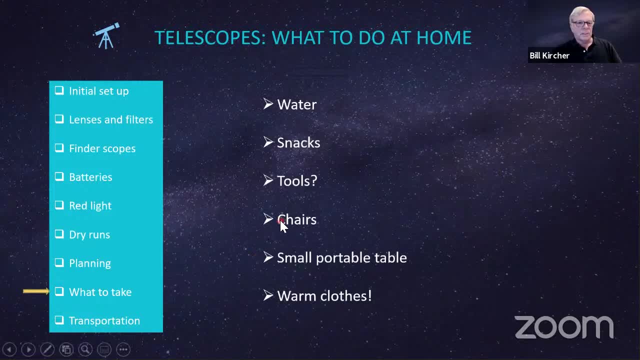 if you're going skiing. We went, my wife and I went to an event where it was very warm when we started And by the time we left- at 1030, we were, shivering notwithstanding, wearing sweaters and backpacks, And we weren't even on Mount Tam. So always have that backup Transportation. This is my. 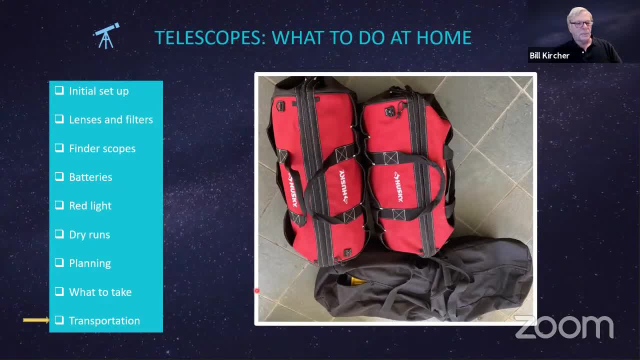 solution. I take my telescope apart and I put the optical tube in one of these tool bags and the mount head in another bag along with some other stuff, And then the black tube type carrier at the tripod And a couple of toolboxes in which I have lenses, filters and other equipment. 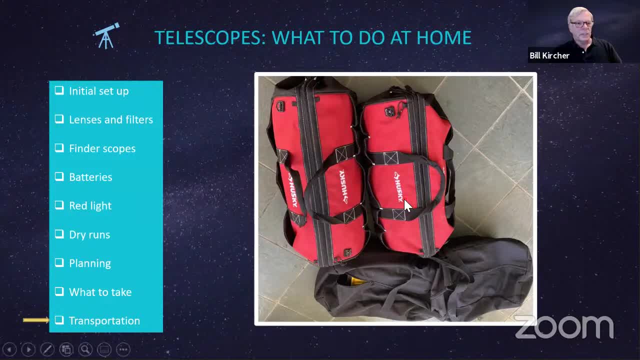 I like this. It's very portable, easy to stow. The tool bags protect the telescope and the mount head. I started out with one large case. It was too unwieldy to lug up and down staircases and try to get into my trunk. But it depends on your telescope. The point of this is be creative. 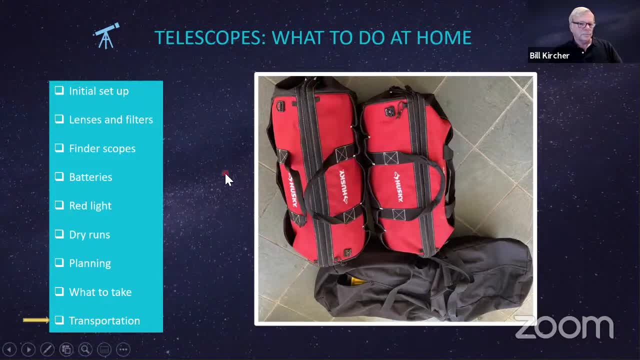 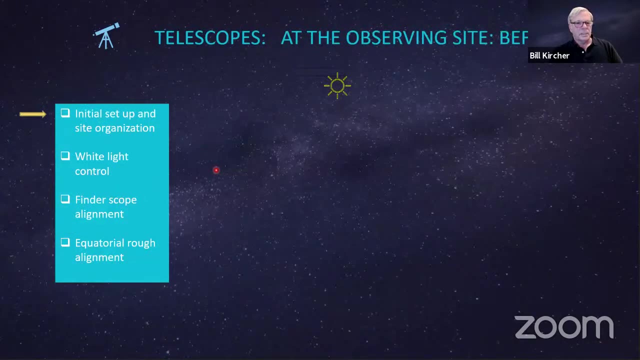 experiment with whatever works for you. Okay, So we've covered a lot at home. Now let's go to the mountain. virtually So, we're at the mountain, The sun is still up, It's daylight And there are some things to do. You're set up, which you've already probably practiced at home. 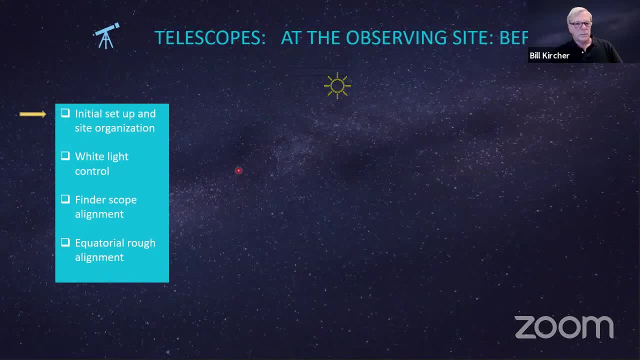 Organizing your site, figuring out where to put your car so that you can leave without disturbing other stargazers at the star party. Remember, everything you take out of your car you're eventually going to put back into your car. So have a plan. It's much easier to take. 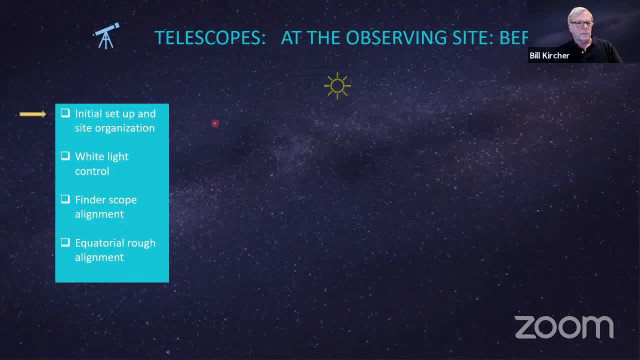 things out in daylight than to put them back in in the dark. You don't want to be down on your hands and knees looking for lens caps and so on. Give some thought to organization. Give some thought to white light control while it's daylight. 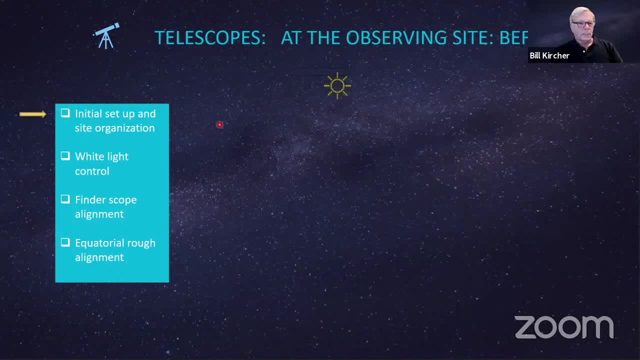 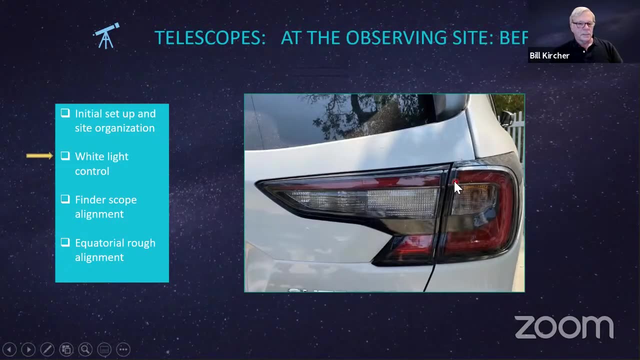 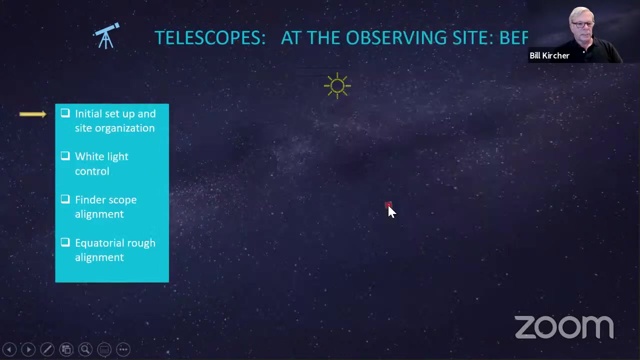 Okay, So white light control. Here's my A close-up of the taillight on my Subaru Outback, And I discovered at a recent star party that when I opened the tailgate, the white light portion of the taillight blinked twice. 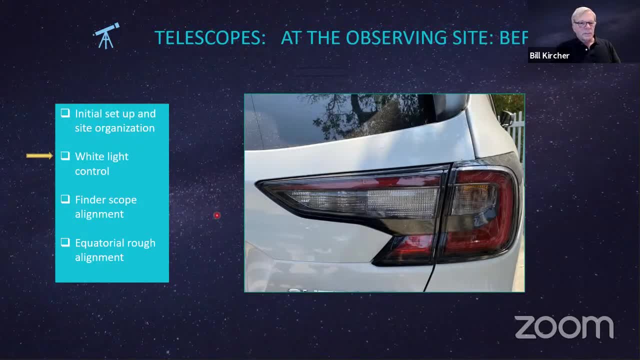 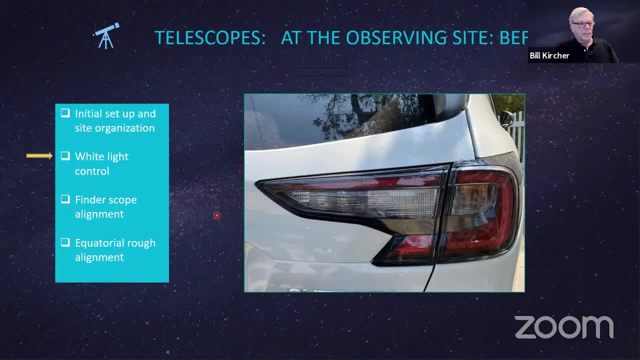 I opened the tailgate, it blinked twice more, And so on and so on. The solution that red tape I told you on and so on, and so on. The solution that red tape I told you on and so on, and so on. The solution that red tape I told you about that. you buy at an auto parts. solution: that red tape. I told you about that. you buy at an auto parts solution: that red tape. I told you about that. you buy at an auto parts store. put it over the white about that. you buy at an auto parts store. put it over the white. 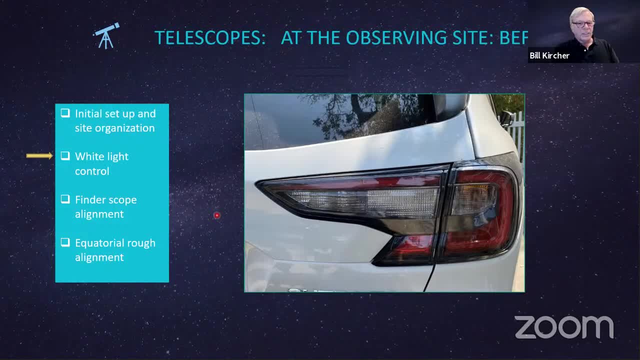 about that you buy at an auto parts store. put it over the white portion of this or over your trunk store. put it over the white portion of this or over your trunk store. put it over the white portion of this or over your trunk light or any other light that you. portion of this or over your trunk light or any other light that you portion of this or over your trunk light or any other light that you can't manage to turn off that light or any other light that you can't manage to turn off that. 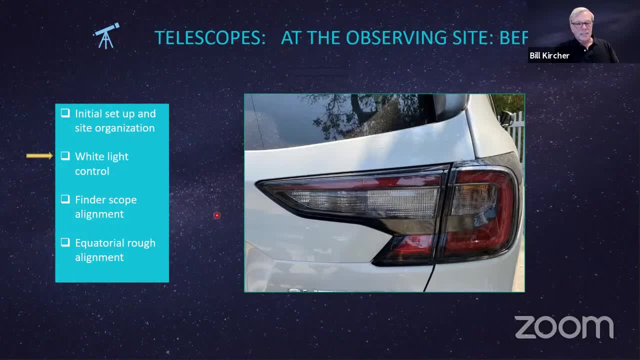 light or any other light that you can't manage to turn off, that may come on during the star party, can't manage to turn off that may come on during the star party. can't manage to turn off that may come on during the star party. My dashboard lights up when I 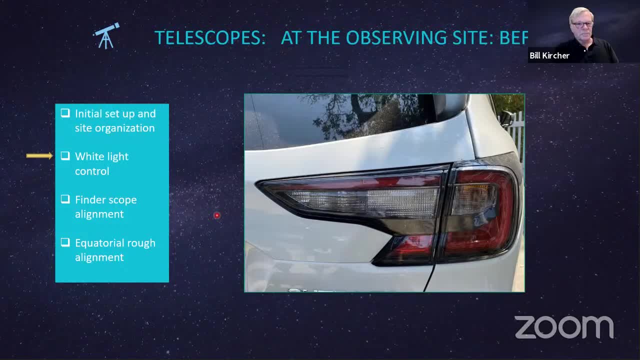 may come on during the star party: My dashboard lights up when I may come on during the star party. My dashboard lights up when I open the door. I throw a towel. My dashboard lights up when I open the door. I throw a towel. My dashboard lights up when I open the door. I throw a towel over it, a colored beach towel. open the door. I throw a towel over it- a colored beach towel. open the door, I throw a towel over it. a colored beach towel- The interior lights usually you can over it. a colored beach towel- The interior lights usually you can. 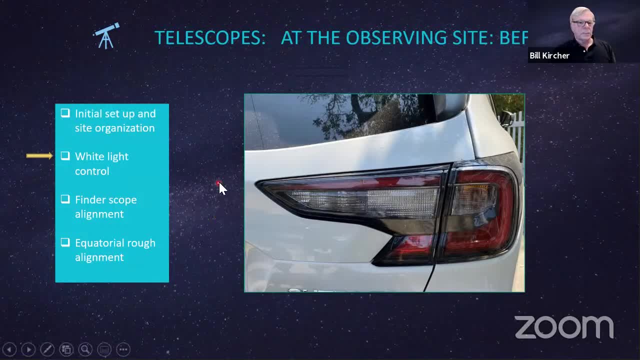 over it a colored beach towel. The interior lights: usually you can just turn off The interior lights. usually you can just turn off The interior lights. usually you can just turn off And take this opportunity to do something. just turn off And take this opportunity to do something. just turn off And take this opportunity to do something with your cell phone to dim the light. And take this opportunity to do something with your cell phone to dim the light. And take this opportunity to do something with your cell phone to dim the light on that. 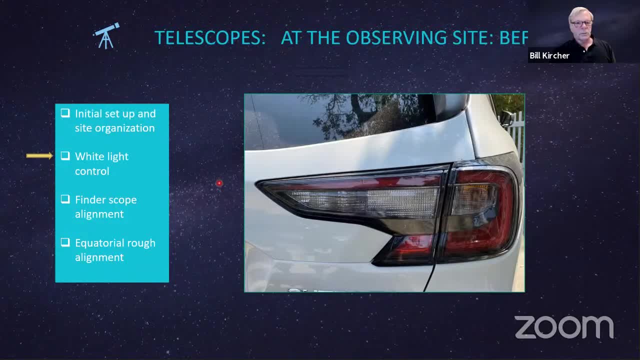 with your cell phone to dim the light on that. with your cell phone to dim the light on that. The iPhone has a setting where you can on that. The iPhone has a setting where you can on that. The iPhone has a setting where you can tint the whole screen red. 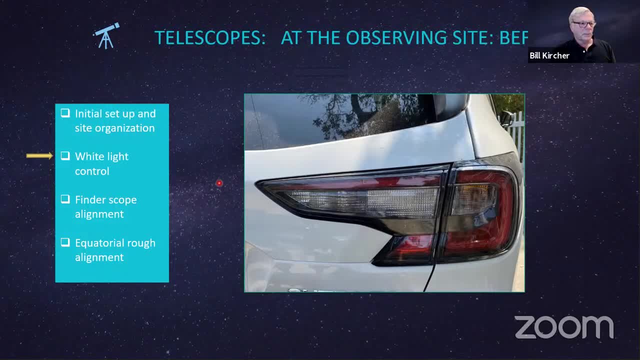 The iPhone has a setting where you can tint the whole screen red. The iPhone has a setting where you can tint the whole screen: red under accessibility. tint the whole screen: red under accessibility. tint the whole screen: red under accessibility. Android probably has something similar. 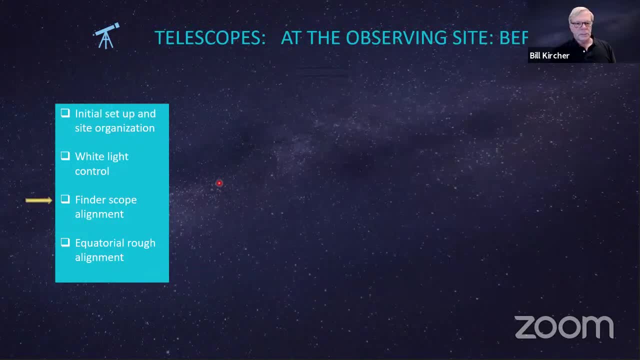 under accessibility: Android probably has something similar. under accessibility, Android probably has something similar. Finder scope alignment is the Finder scope. alignment is the Finder scope. alignment is the next subject. Okay, we already talked next subject. Okay, we already talked next subject. Okay, we already talked about that. If you did it once at: about that, If you did it once at about that, If you did it once at home and you have a fixed finder home and you have a fixed finder home and you have a fixed finder scope. maybe that's enough, but you scope. maybe that's enough, but you. 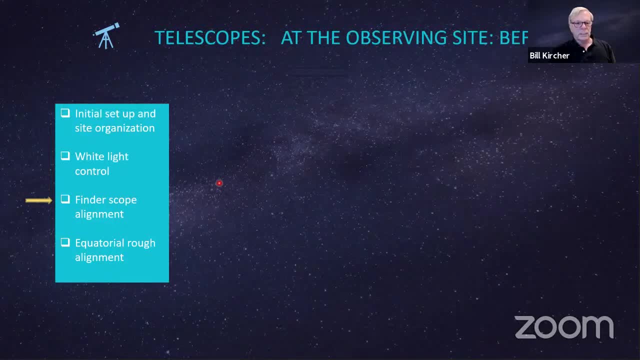 scope. maybe that's enough, but you might want to check it. I remove my. might want to check it. I remove my. might want to check it. I remove my finder scopes and then reattach them. finder scopes and then reattach them. 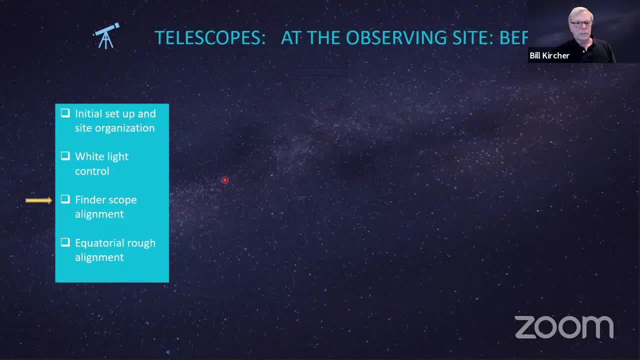 finder scopes and then reattach them. So I always check it and usually I So I always check it and usually I So I always check it and usually I have to tweak the finder scopes, have to tweak the finder scopes, have to tweak the finder scopes. Equatorial mount. this is the time you. 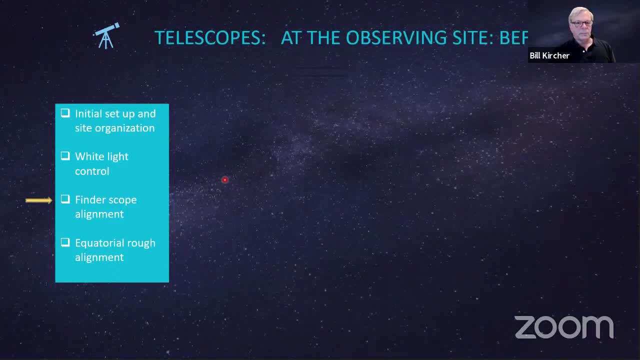 Equatorial mount. this is the time you, Equatorial mount, this is the time you can do the rough alignment we talked can do the rough alignment we talked can do the rough alignment we talked about before, about before, about before. Aim it towards the north, put it in. 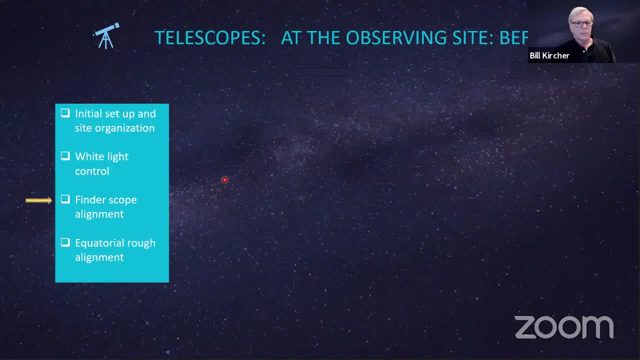 Aim it towards the north, put it in, Aim it towards the north, put it in the home position. the home position, the home position. You can do the same thing with your, You can do the same thing with your, You can do the same thing with your. go-to equatorial mount. 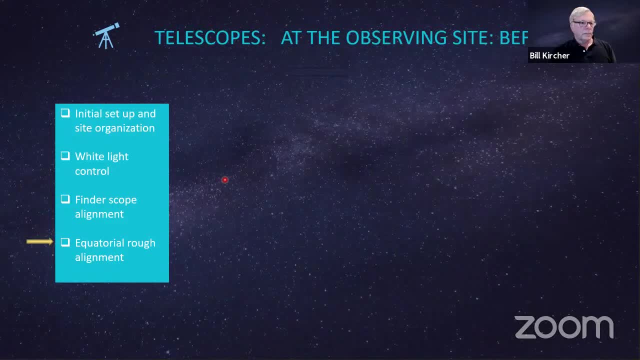 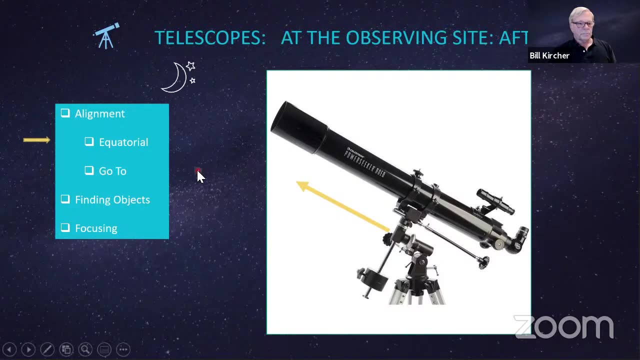 go-to equatorial mount. go-to equatorial mount, And now And now And now, after dark, after dark, after dark. So here's the manual equatorial mount. So here's the manual equatorial mount. So here's the manual equatorial mount again. 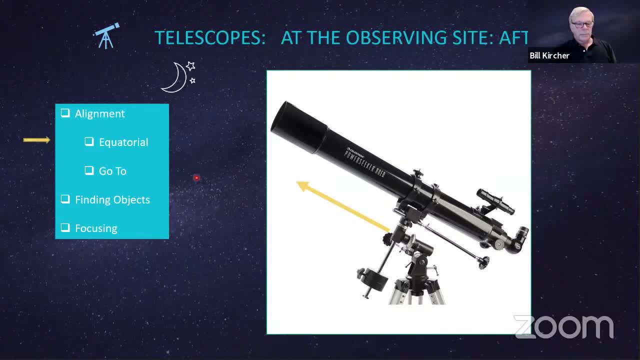 If you set this upright, and If you set this upright, and If you set this upright and aimed it to the north and put it in, aimed it to the north, and put it in, aimed it to the north, and put it in the home position, the home position. 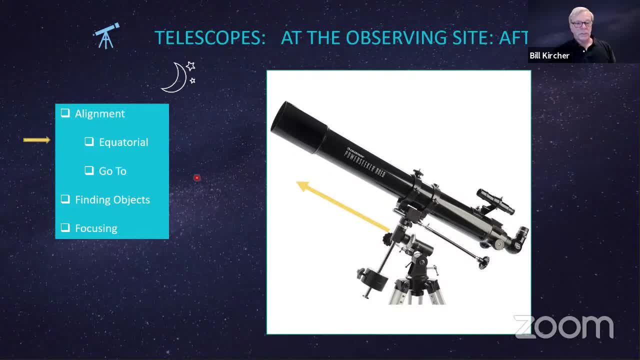 the home position. you hopefully can look through the. you hopefully can look through the. you hopefully can look through the eyepiece. and now Polaris is out, see eyepiece. and now Polaris is out, see eyepiece. and now Polaris is out, see Polaris. 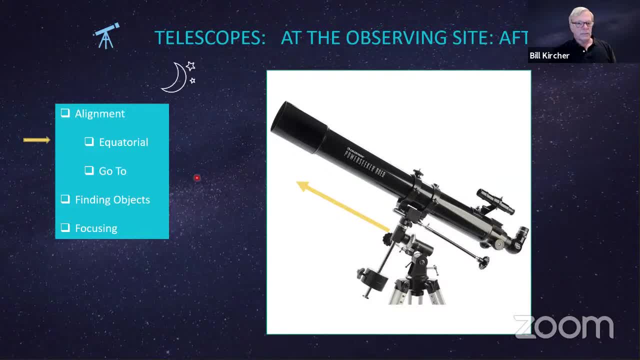 Polaris, Polaris. If it's not centered, then you need to. If it's not centered, then you need to. If it's not centered, then you need to move the scope so that it is centered. move the scope so that it is centered. 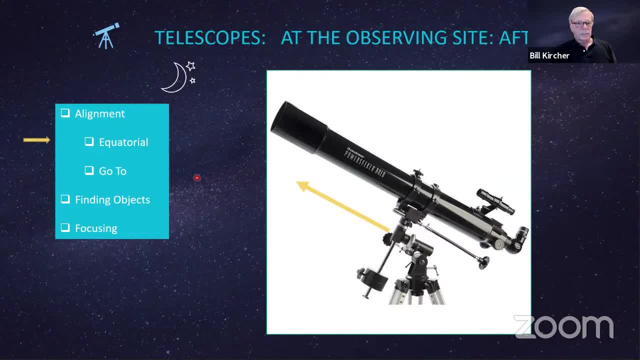 move the scope so that it is centered With the go-to equatorial, With the go-to equatorial, With the go-to equatorial. a number of the, a number of the, a number of the more recent and more expensive go-to. more recent and more expensive go-to. 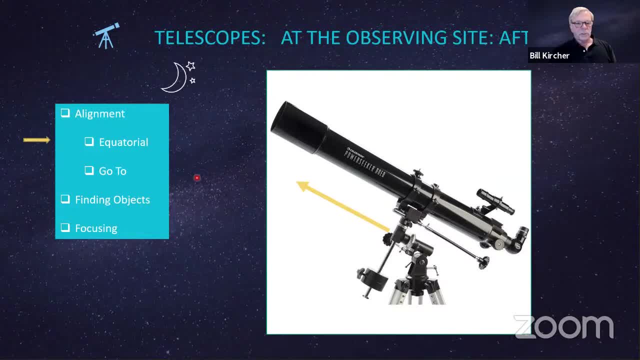 more recent and more expensive go-to mounts will have a mounts will have a mounts will have a finder scope. a polar scope that's finder scope. a polar scope that's finder scope. a polar scope that's built into the polar axis- built into the polar axis. 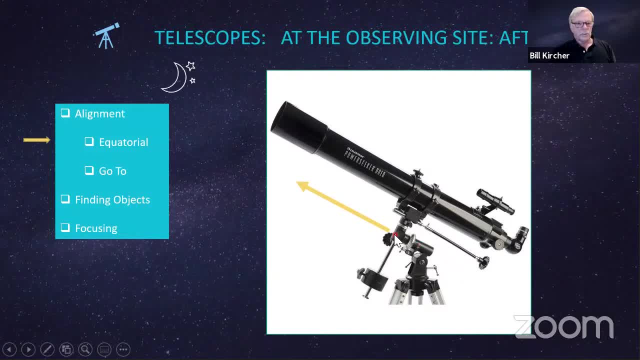 built into the polar axis So you can actually sight through the, So you can actually sight through the, So you can actually sight through the axis directly to axis, directly to axis, directly to Polaris, to make sure your Polaris, to make sure your Polaris, to make sure your alignment is accurate. 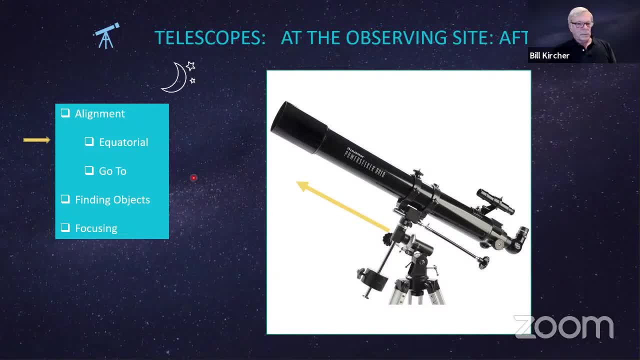 Now, if you have a go-to mount, Now, if you have a go-to mount, Now, if you have a go-to mount, you need to align the telescope so it. you need to align the telescope so it. you need to align the telescope so it will go places. 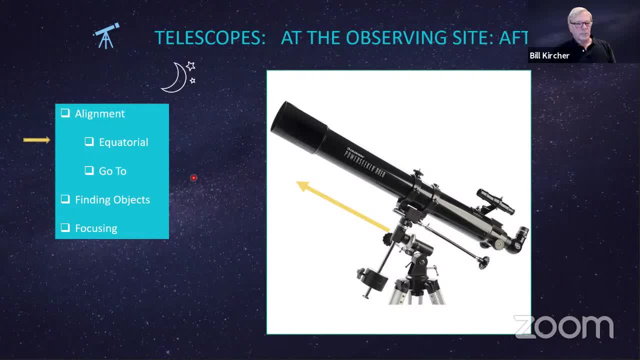 will go places will go places. It will go where you want it to It. It will go where you want it to It. It will go where you want it to It. doesn't just do that First the. doesn't just do that First the. 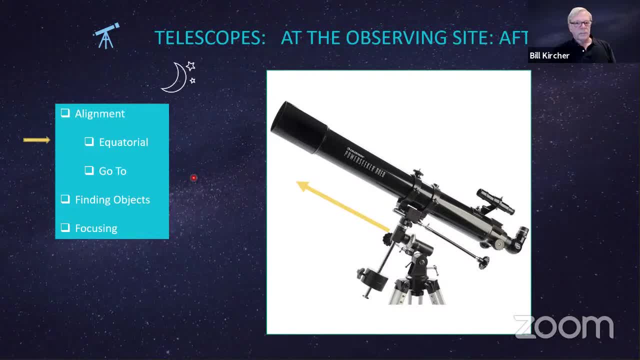 doesn't just do that. First, the telescope has to be aligned, which is telescope has to be aligned, which is telescope has to be aligned, which is a process of the telescope developing a, a process of the telescope developing a, a process of the telescope developing a kind of an internal map of the sky. 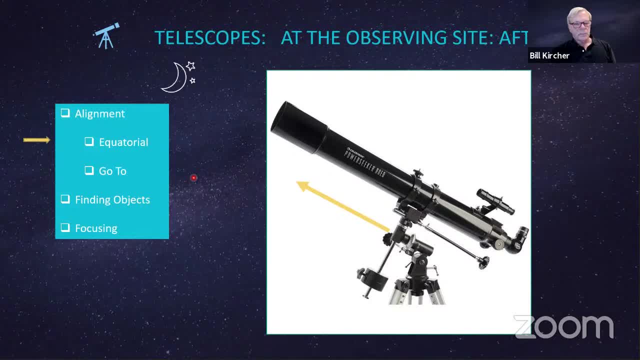 kind of an internal map of the sky. kind of an internal map of the sky, so it will know which way it's pointing. so it will know which way it's pointing. so it will know which way it's pointing If you have a Dobsonian or a manual. 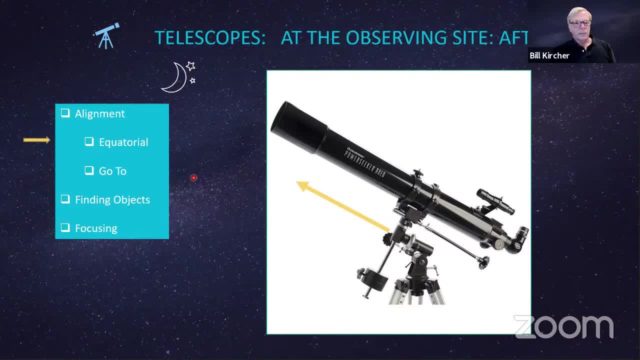 If you have a Dobsonian or a manual. If you have a Dobsonian or a manual, alt-azimuth telescope, you are home. alt-azimuth telescope, you are home. alt-azimuth telescope. you are home free. You're free to go and start. 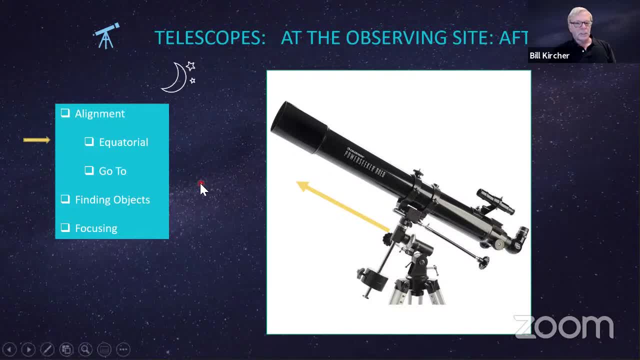 free. You're free to go and start free. You're free to go and start observing. But those of us who have observing, But those of us who have observing, But those of us who have go-tos, the fun is just beginning. 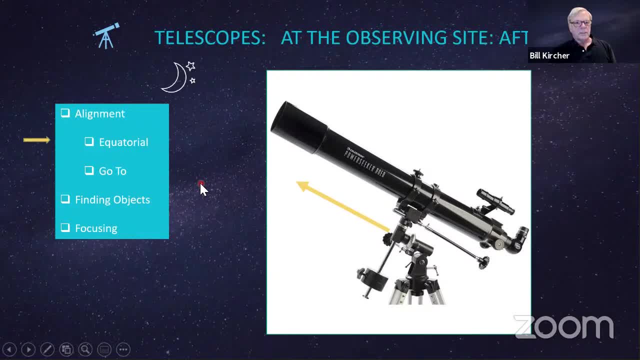 go-tos, the fun is just beginning. go-tos, the fun is just beginning, because now we have to align our, because now we have to align our, because now we have to align our telescopes, telescopes, telescopes. It does get easier with experience, but 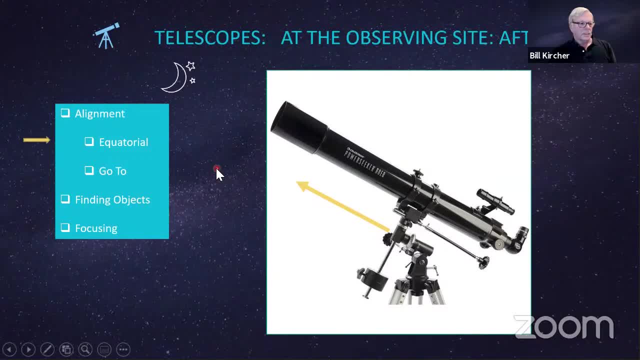 It does get easier with experience. but It does get easier with experience, but it has various steps and it has various steps and it has various steps and you have to go through this sequence. you have to go through this sequence. you have to go through this sequence in a particular order. Some of the 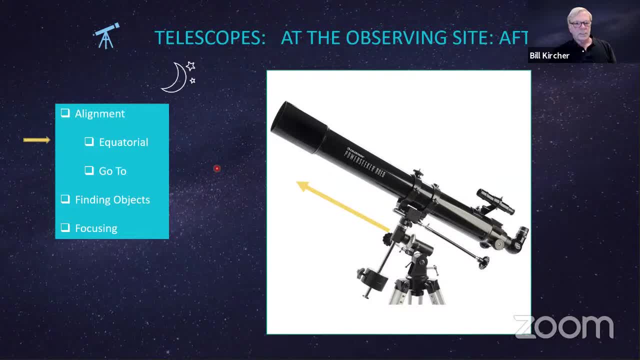 in a particular order. Some of the in a particular order. Some of the more recent and more expensive, more recent and more expensive, more recent and more expensive telescopes have a plate solving telescopes have a plate solving telescopes have a plate solving type of software. that's a little. 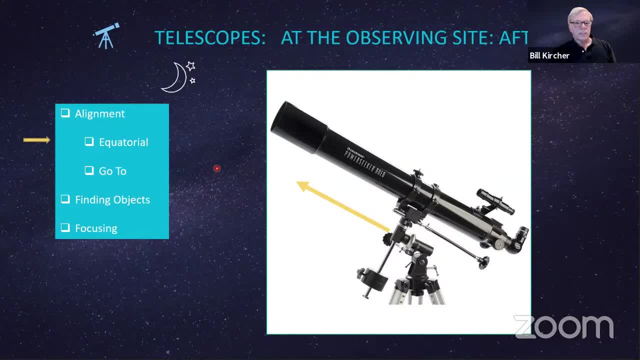 type of software. that's a little type of software. that's a little different, different, different With my EV scope, for example, the. With my EV scope, for example, the. With my EV scope, for example, the alignment is virtually automatic. 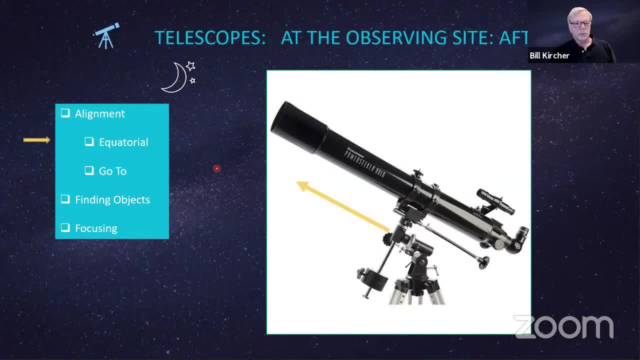 alignment is virtually automatic. alignment is virtually automatic. Otherwise, though, you have to. Otherwise, though, you have to. Otherwise, though, you have to. you're a participant, You have to, you're a participant, You have to, you're a participant. You have to find certain objects and align on. 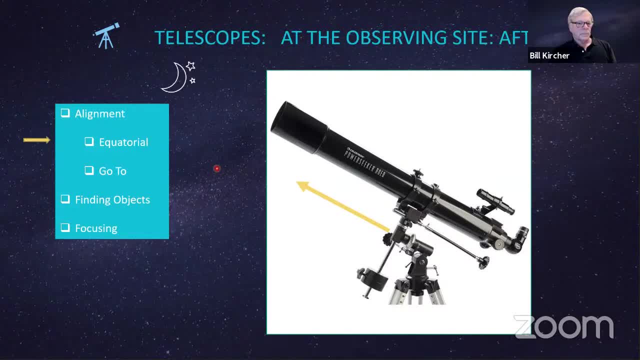 find certain objects and align on. find certain objects and align on those objects, those objects, those objects. So here is the, So, here is the. So here is the sequence for my Celestron 8SE. sequence for my Celestron 8SE. 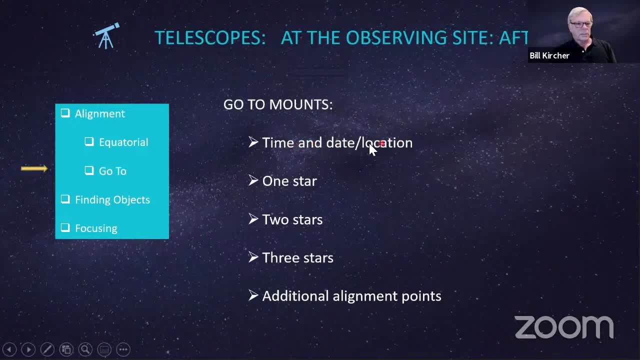 sequence for my Celestron 8SE. We're back to entering the time. We're back to entering the time. We're back to entering the time and date, the location and date. the location and date. the location Presumably I've already entered. 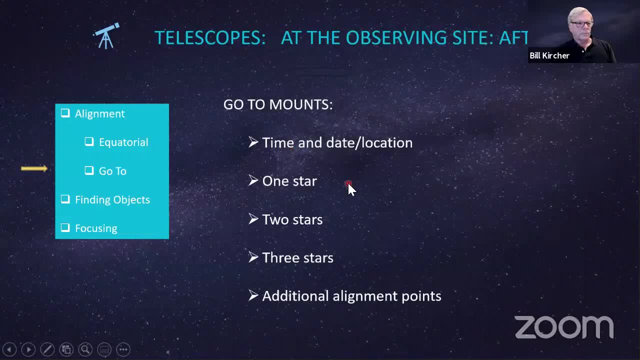 Presumably I've already entered, Presumably I've already entered that. but it needs that that, but it needs that that, but it needs that information to start, information to start, information to start GPS module. maybe it automatically. GPS module, maybe it automatically. 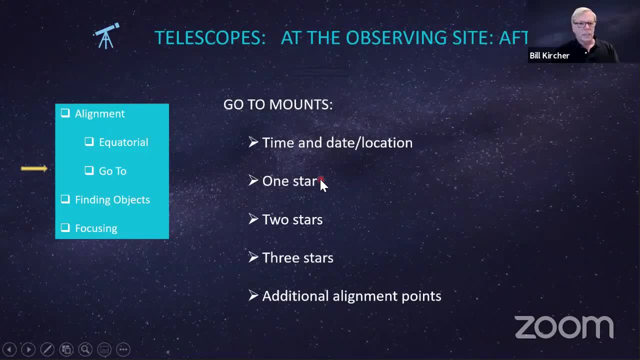 GPS module. maybe it automatically acquires it, acquires it, acquires it. It just wasn't reliable on my, It just wasn't reliable on my, It just wasn't reliable on my telescope, so I do it manually. telescope, so I do it manually. Then you have a choice, one star. 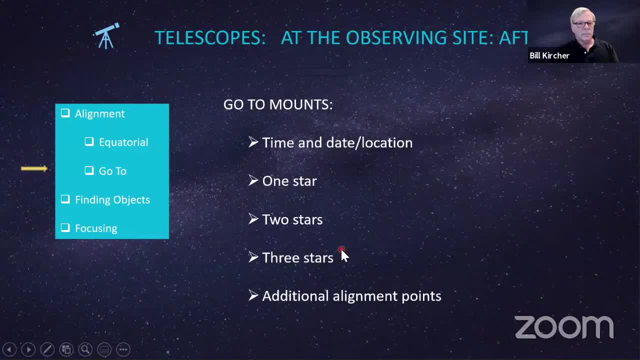 Then you have a choice: one star, Then you have a choice: one star, two stars, three stars, two stars, three stars, two stars, three stars. One star is a quick alignment. One star is a quick alignment. One star is a quick alignment, like we did in our practice: dry run. 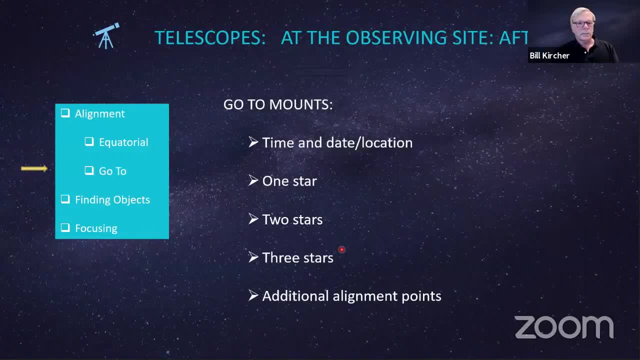 like we did in our practice dry run, like we did in our practice dry run session, session, session. And if all you want is tracking, let's. And if all you want is tracking, let's. And if all you want is tracking, let's say you want to observe Jupiter. 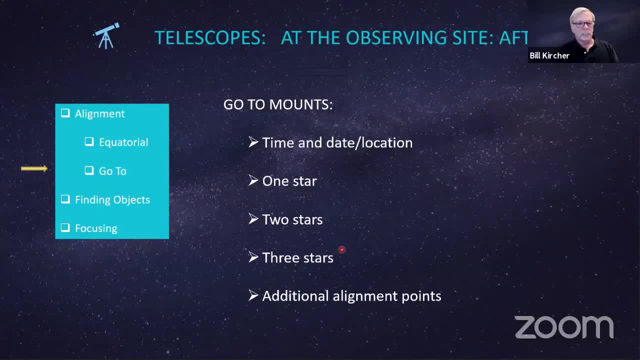 say you want to observe Jupiter, say you want to observe Jupiter, you can find Jupiter easily on your. you can find Jupiter easily on your. you can find Jupiter easily on your own. but you want your telescope then own. but you want your telescope then to track, do one star alignment. 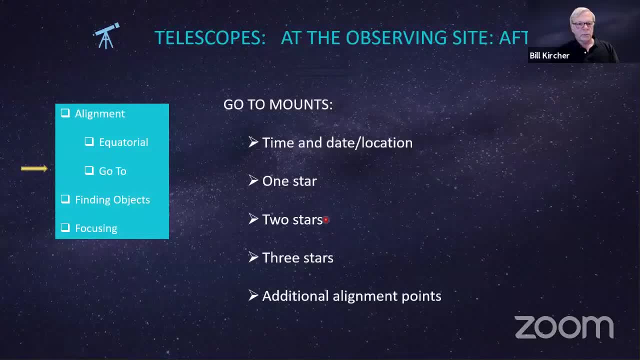 to track. do one star alignment to track. do one star alignment. Two stars: I use when my view is Two stars. I use when my view is Two stars. I use when my view is obstructed and I'll never find three obstructed and I'll never find three. 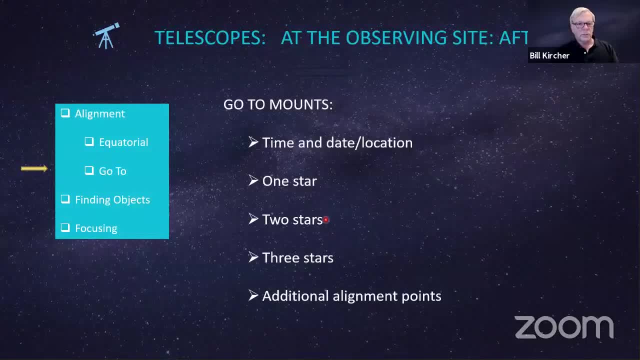 obstructed and I'll never find three stars, stars, stars. A good view of three stars. There's a? A good view of three stars. There's a? A good view of three stars. There's a building. there's trees. building, there's trees. 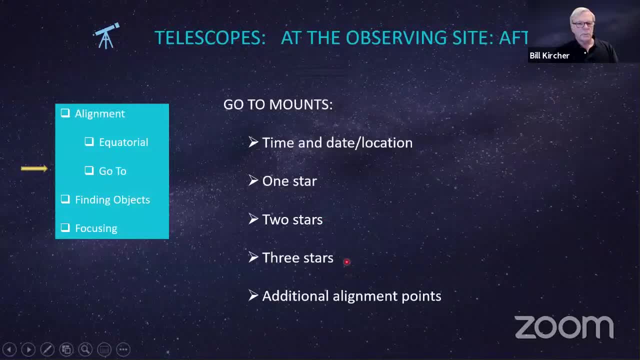 building there's trees, But the typical alignment if you want, But the typical alignment if you want, But the typical alignment if you want to use GoTo would be three stars. to use GoTo would be three stars, So you need to find three objects, center on them and enter the right commands in your controller or your cell phone if you're using an app. 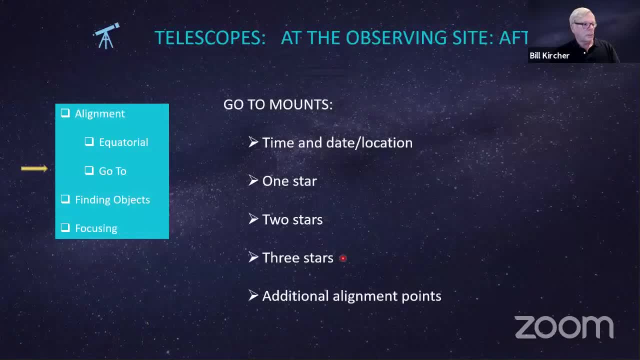 And then you've completed the alignment and then you can use the go-to If you're looking for an object that's hard to find. actually, you're probably going to have to go to that region of the sky and start adding additional alignment points. 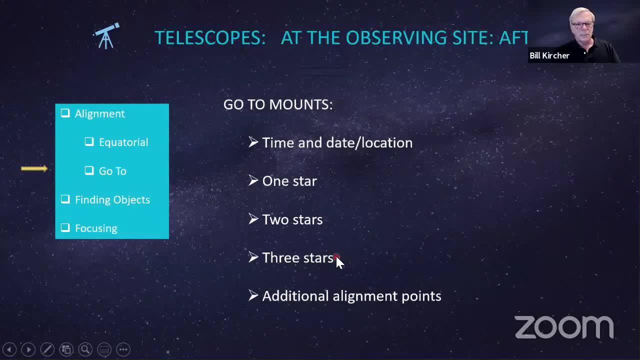 It's a tedious process, but it may be necessary if you can't find the object with what you've already entered. The go-to equatorial is going to be a bit different, have different steps, different manufacturers have different programs, But I think many of them follow something like this regimen. 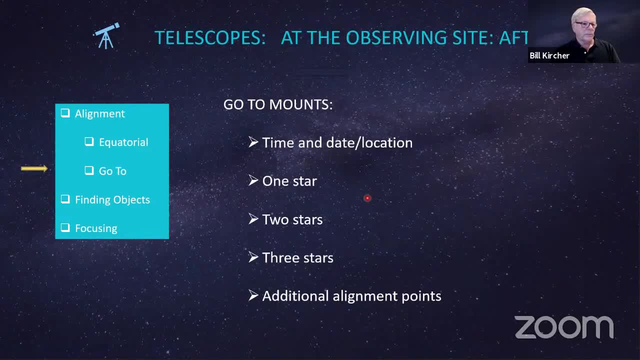 You'll need to customize this for the particular telescope you have. Finding objects: Okay, Apart from go-to, how would you find an object that's hard to find? So here's an exercise: We're going to find the Andromeda Galaxy. 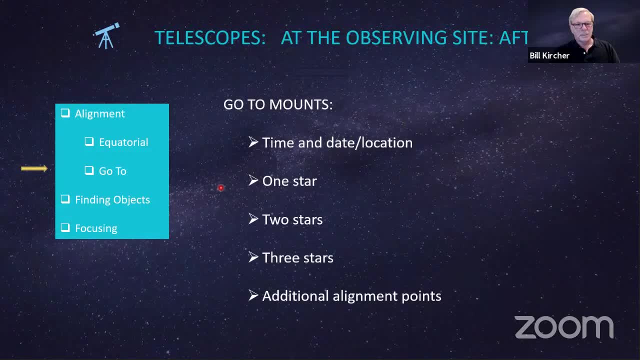 This is not an ideal time to observe it. It is up. if you wait for the right time in the evening, You'll have a better experience in October, November, but it seemed like a good example, so bear with me All right. 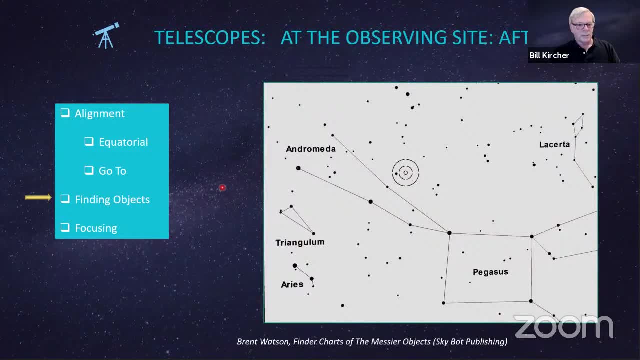 So this is from a great researcher, This is a great resource: the Skybot series of maps, this one on Messier objects- Messier, I guess, would be the right pronunciation: objects- And we're looking for the Andromeda Galaxy. 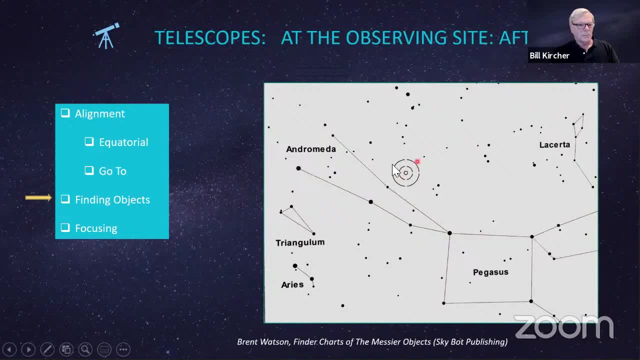 Well, in this spiral-bound book of maps the reticule of the Telrad is already included. So in the bullseye that's where the Andromeda, Andromeda Galaxy is. It's a big galaxy. so actually it's not just in the bullseye. 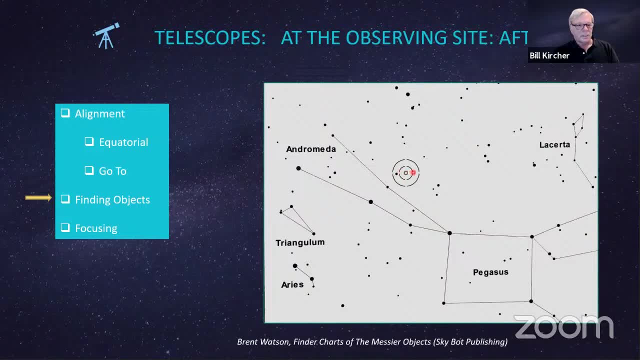 But let's say the center is in the bullseye and then the galaxy actually spreads out a bit across the reticule. But you may not be able to see it at all. It may be just barely visible, Visible through binoculars, maybe as kind of a smudge, but not really visible to your finder. 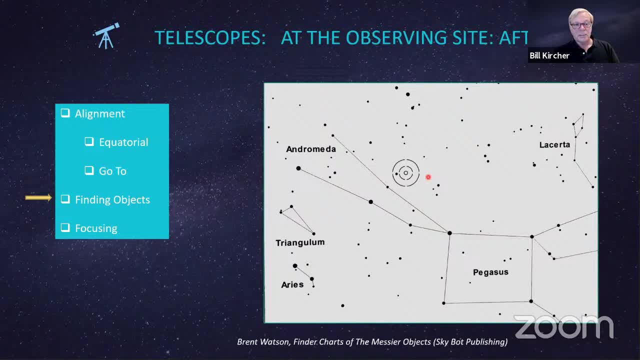 And you have a Telrad. You have the setup. I have a Telrad, but also a magnified finder. So let's walk through this. First, we need to get oriented. We'll start with an asterism, which is this great square in the constellation Pegasus. 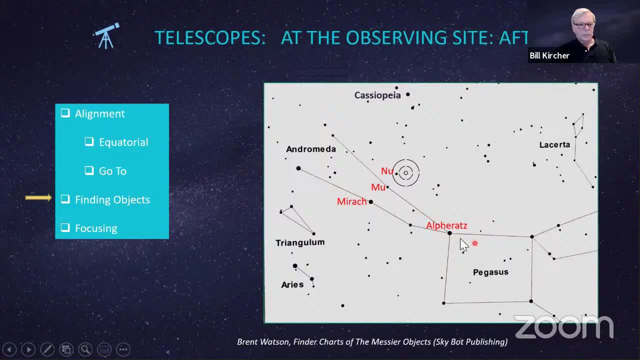 And, in particular, once we found the great square, find this bright star, relatively bright star, Alpharetz. It's a second magnitude star, About as bright as the Polaris. And then look for Merak, which is the same about a second magnitude star. 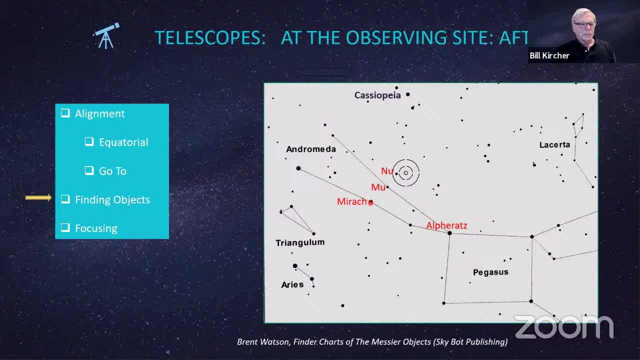 I think it's pretty easy to find because there's not a lot else around it. So, by the way, the great square is part of Pegasus And the Andromeda Galaxy. is this V shape here that appears to be attached to Pegasus? 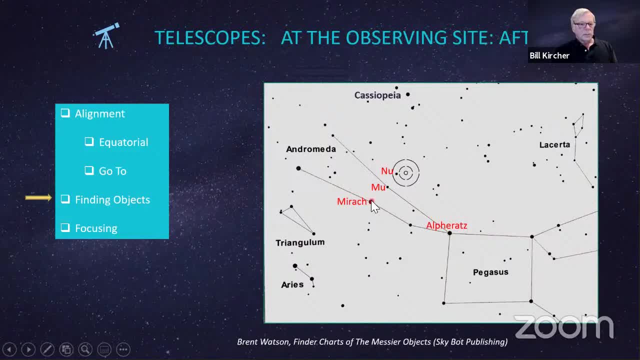 So if we go above Merak we'll see Mu, another star, but quite a bit dimmer. Probably can't see it with the naked eye in conditions around the Bay Area And Nu above that, which is even dimmer. 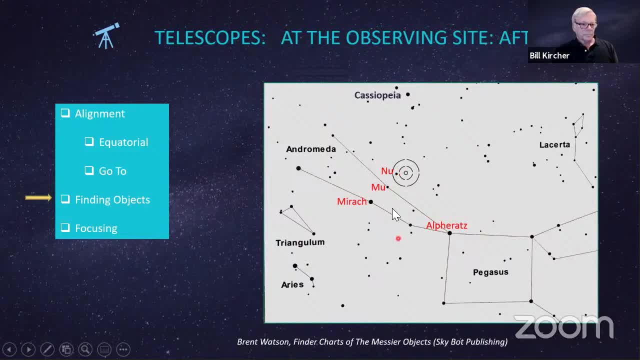 So, and, by the way, the constellation Cassiopeia is out there. So if we go above that, we'll see Mu, another star, but quite a bit dimmer. Probably can't see it with the naked eye in conditions around the Bay Area And Nu above that, which is even dimmer. So if we go above that, we'll see Mu, another star, but quite a bit dimmer. So if we go above that, we'll see Mu, another star, but quite a bit dimmer. Easily recognizable the asterism W. 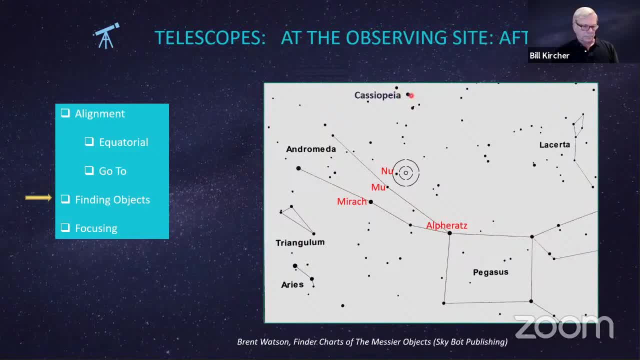 Or, if you look at it from the other side, a big M in the sky. So Cassiopeia would be north of Pegasus. So how are we going to get from Alpheraz and Merak over to the galaxy? 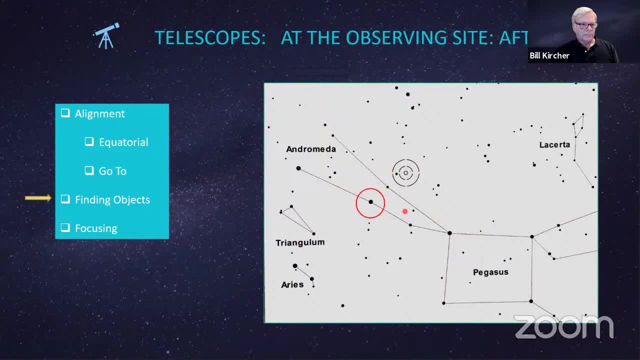 Well, let's start with our Telrad. So the red circle is the Telrad, The Telrad focused on Merak. Now we're going to move towards Andromeda in the direction we think Andromeda is located. So the red circle now has moved, so that Merak is now down towards the edge of that circle. 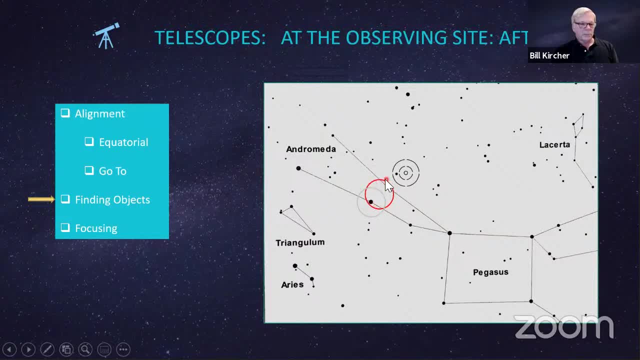 And, by the way, here I will have Swayed. So I'm going to switch to my magnified finder, which the field of view is slightly larger than the reticule on the Telrad. So I want Merak here down in. let's say, this is about the 8 o'clock position, would you say. 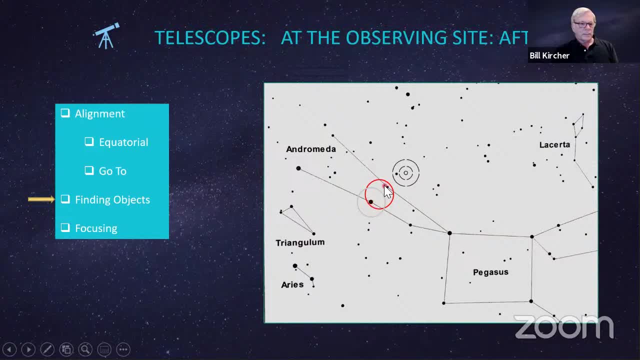 Something like that. if this were a clock face- And since it's magnified, I should now be able to see Mu up here. And what does that look like? Maybe 2 o'clock? Well, let's see Clock face. 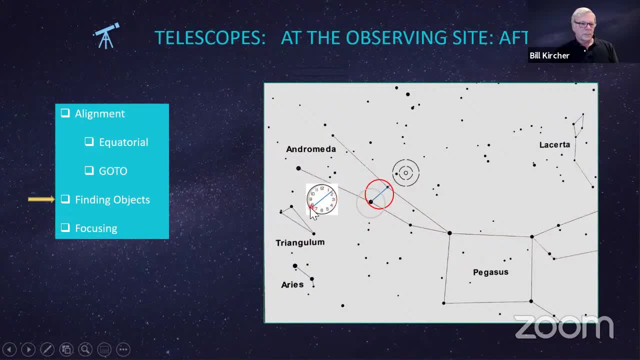 Okay, not quite 2 o'clock, These are parallel lines, So about 8 o'clock for Merak and close to 2 o'clock for Mu. Again, we're now looking through the magnified finder, Otherwise I wouldn't be able to see Mu. 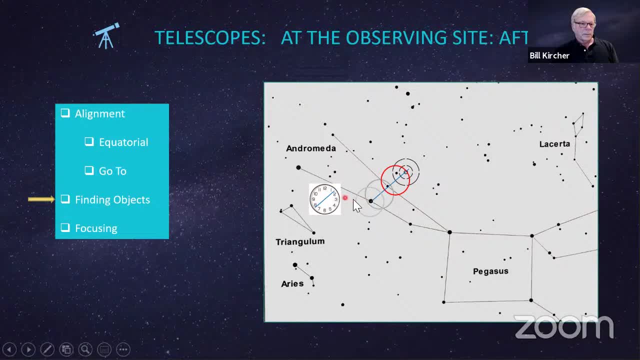 And then the next step. the third step is to keep going in that same direction, so that now Mu is down in the 8 o'clock position And here, up here at 2,, the Andromeda Galaxy through the magnified finder. 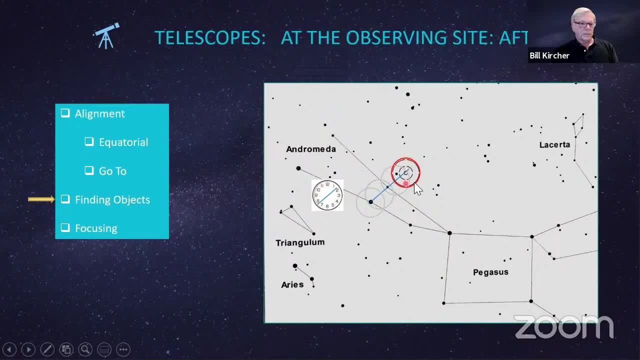 Let's go one more step Now. the finder is over superimposed here, meaning that the Andromeda Galaxy should now be centered. Well, let's look through the telescope and see if it is. If it's not, it should still be something that's visible. 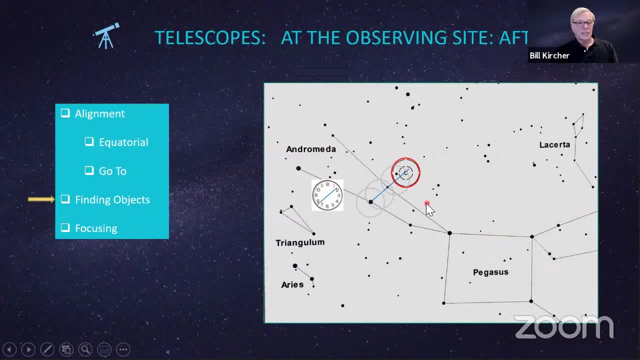 And now we can center it in the telescope. By the way, the Andromeda Galaxy is pretty big. I couldn't fit the whole thing in my field of view, But you get the idea. So this is an example of star hopping using finders. 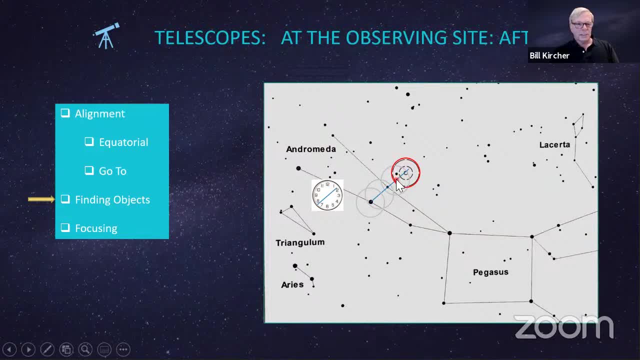 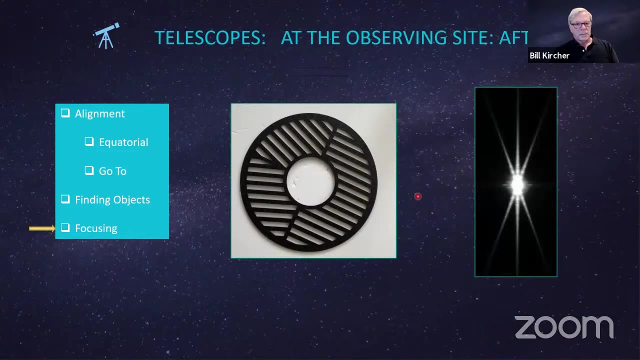 And you'll have to use what you have and spend some time planning it and thinking about how you're going to do it. But this is the process, Okay, So let's go on to focus. Here are some focusing. Here is a focusing aid: the Battenhoff mask. 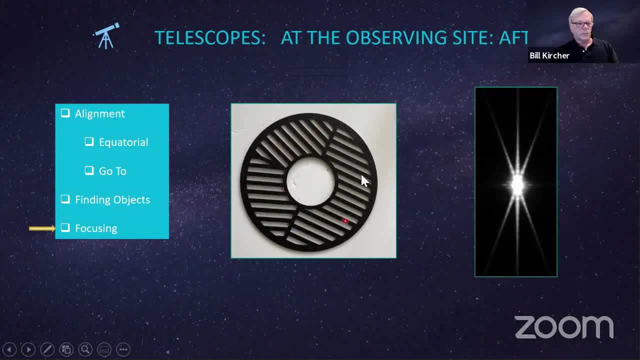 You can buy this on Amazon. Buy one for your telescope. This is for my telescope: Eight inches with a central cutout, because that's what I have on the corrector plate of my telescope, Fits right over the front, Just pops on. 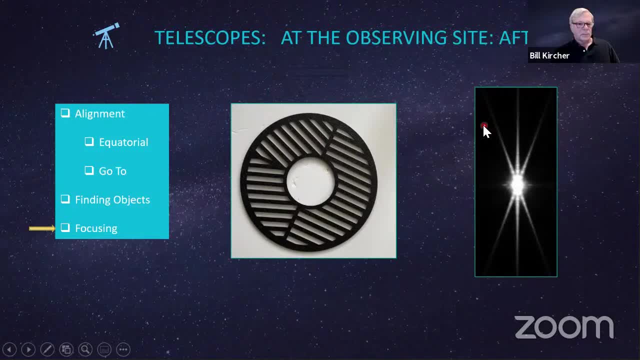 And then you get an image like the image on the right, That looks like an X with a spike in the middle. If the spike is perfectly centered in that X, you're focused. If it's to one side or the other, you're not. 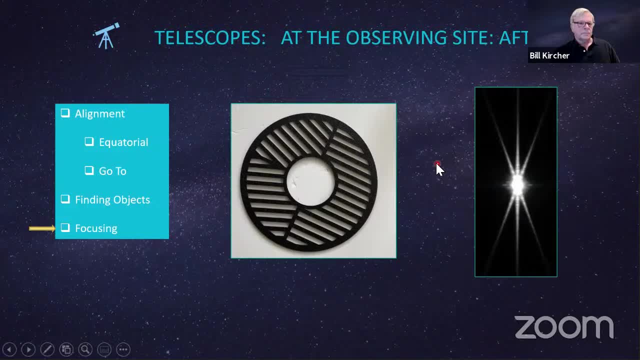 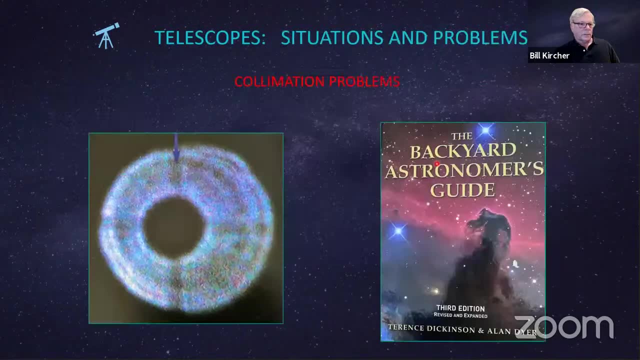 Move the focus until that spike is in the middle. Okay, Problems, Collimation: This is a subject I could go on about for quite a while And I'm going to go through it. I'm going to have to leave it with just sort of an introduction to the issue. 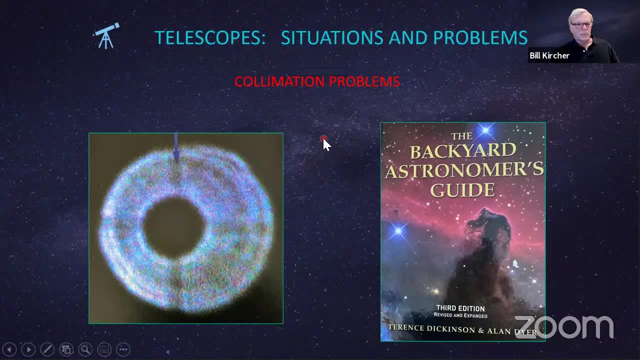 Dobsonians, Newtonian reflectors have collimation issues. Sooner or later they probably have to be collimated. Even my Schmidt-Cassegrain had to be collimated. Of course I dropped it on the floor first, But sooner or later, because of jostling as you move, the telescope around, the mirrors can get out of alignment. 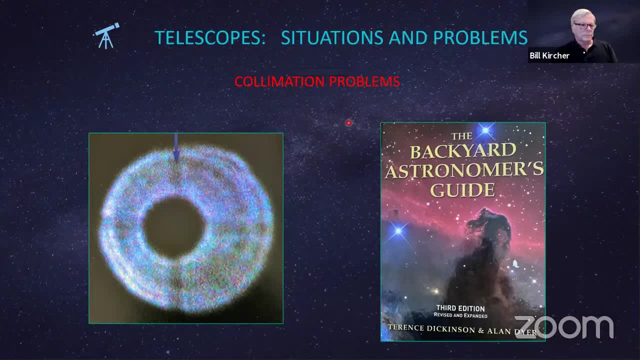 The main mirror, or sometimes the secondary mirror, And the collimation process is different. But here's a quick test that you can do. if you think you might have a collimation problem, Look at a reasonably bright star. Center it in your eyepiece. 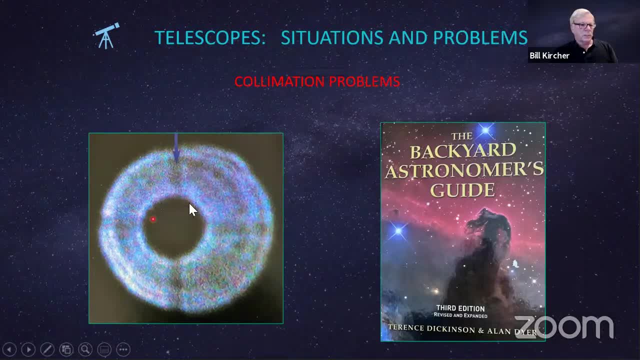 And then defocus it, And as you defocus it it will get bigger and start to look like a donut. This black portion here is caused by the central obstruction, Your secondary mirror, And if it's off-center then you need to collimate. 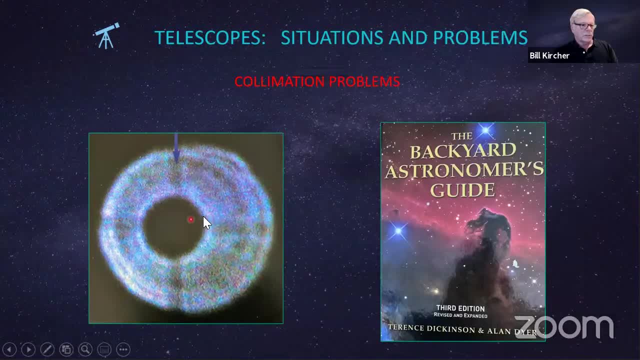 Now see, this is off-center. It should be perfectly centered in the donut. I have, on the right, shown you the cover of the Backyard Astronomer's Guide. This is a great book And it covers many subjects, including collimation. 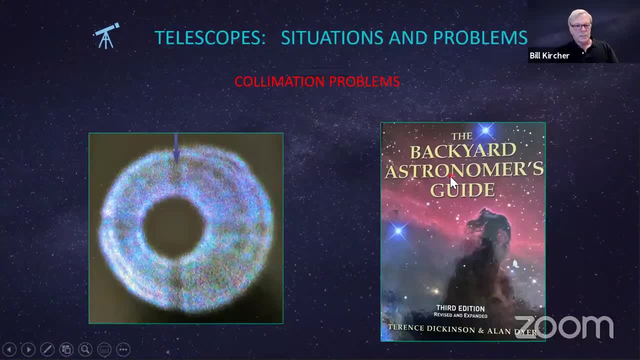 And this image is from the Backyard Astronomer's Guide. One caveat: I think Fourth edition is about to come out. I tried to pre-order it. I hope I'm on the list. Well worth it A little out of date. 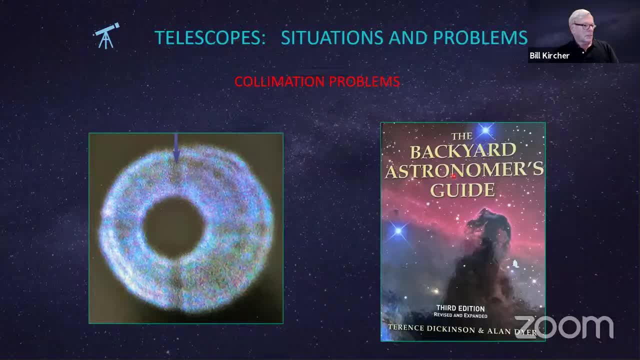 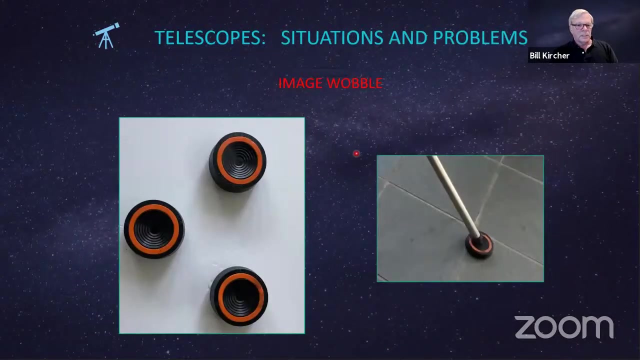 But a great resource on all aspects of amateur astronomy and telescopes. So again, highly recommend it. Okay, Another problem is image wobble. You're trying to observe, say, Jupiter, And you can't see any detail because it's jiggling and wobbling and all over the place. 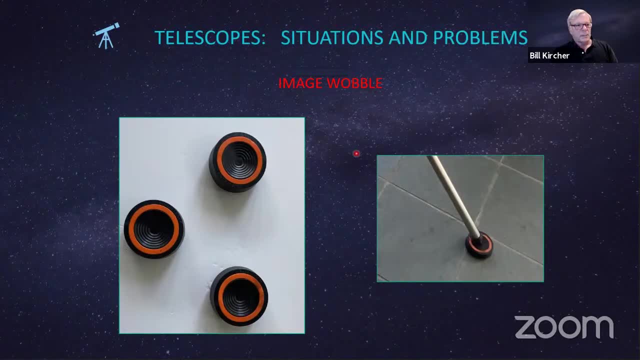 Like you're looking through liquid or boiling water. Well, that could be a scene problem. It could be. you know, the air is so turbulent above you that it's distorting the image And there's not much you can do about it. 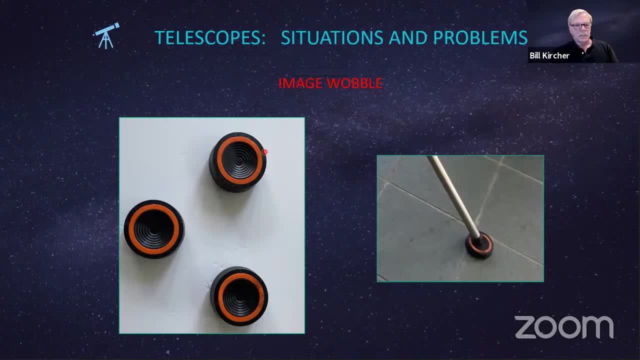 Or it could be something closer to home. Your telescope may not have cooled off enough. Maybe the convection currents Inside your telescope are causing this, Or maybe it's the asphalt parking lot at the Mount Tam Rock Springs parking lot. If it's the latter, then just wait until things cool down. 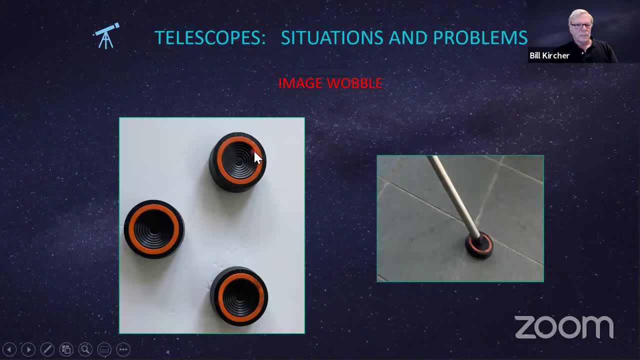 But it could also be vibration If you have a mount that is subject to vibration. Any vibration from a car or even people walking around is magnified a lot by your telescope. You don't notice it until you look through And see a magnified image. 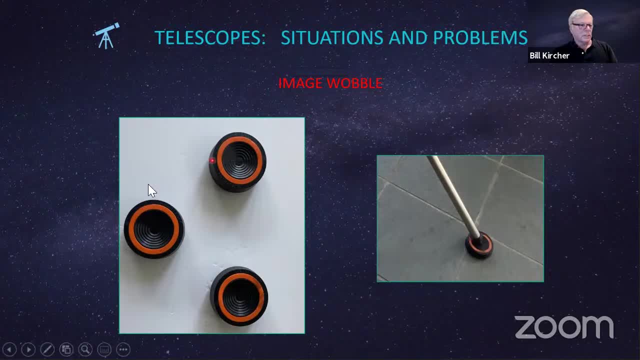 So here's a solution, a partial solution. Celestron sells these pods that you can put your tripod on, So here's on the right is an image of the tripod in one of these holders. You can also buy these, apparently, in a version that's illuminated for safety. 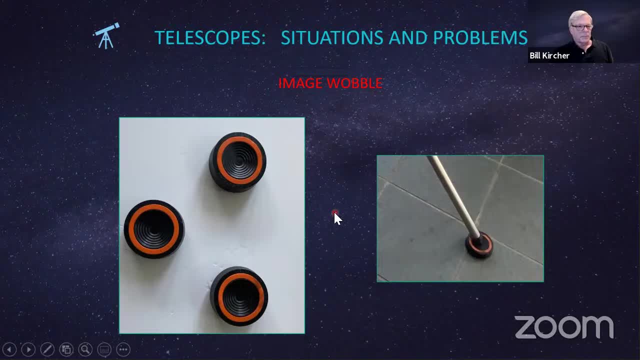 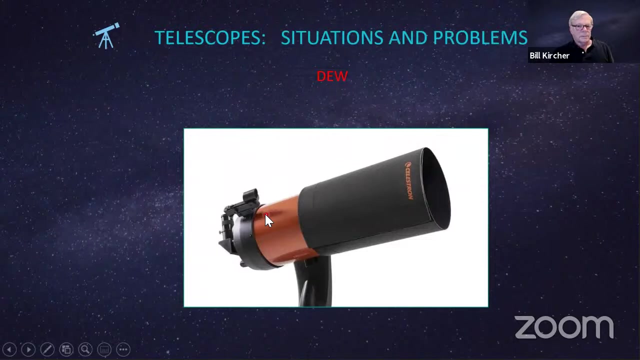 And that's a good thing, And that's a. that's another possibility, a partial solution, and can can improve your experience a bit. Another problem is dew. So dew happens because of changes in temperature. This is a dew shield available from Celestron. 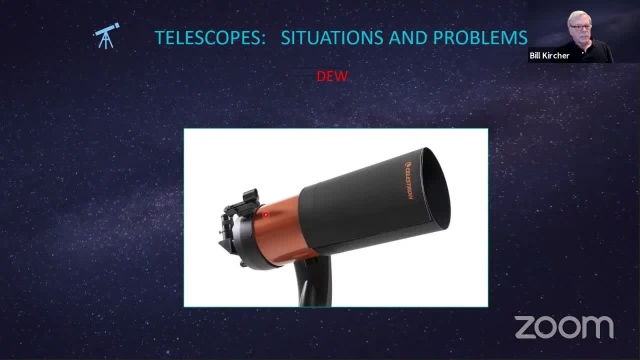 Wraps right around your telescope and creates a kind of a buffer zone to keep the corrector plate warmer. Yeah, You can do something, Something similar with a refractor. if that doesn't work, then you probably need to buy. You could use a small hairdryer just to warm the corrector plate or objective lens up a tiny bit. 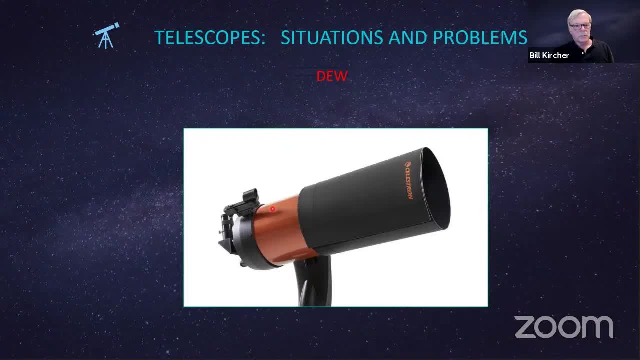 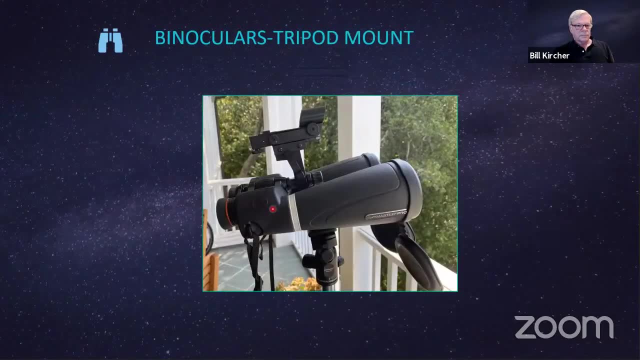 There are also devices that are dedicated warmers. Okay, so let's go on now to binoculars. A lot of what I've already said about telescopes applies to binoculars: planning, red light control, Care of your lenses. 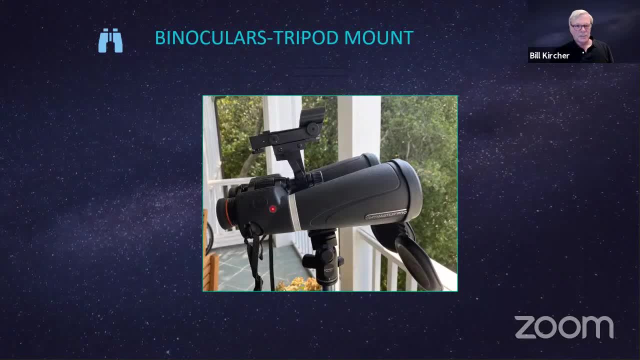 Keep your lens caps on. Don't plant a thumb plant on your lenses because these- the eyepiece lenses and the objective lenses- are also coded. So handle with care. But you don't have all the hassles with setup and so forth that you have with the telescope. 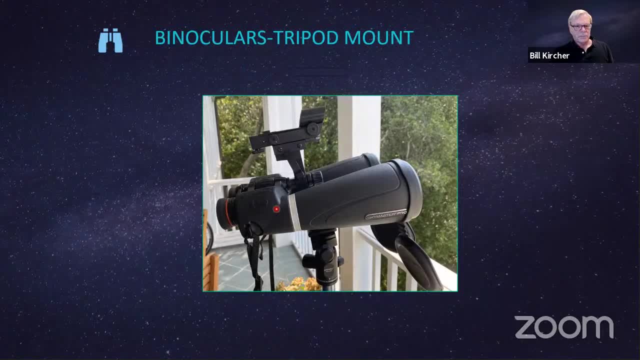 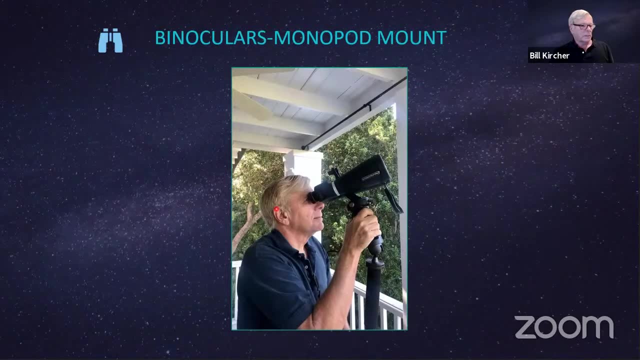 Here I have a set that is mounted on a tripod. That's one possibility. Here I am looking through the binoculars on a monopod. That's just a single pole with a trigger ball head mount so I can swivel it around. 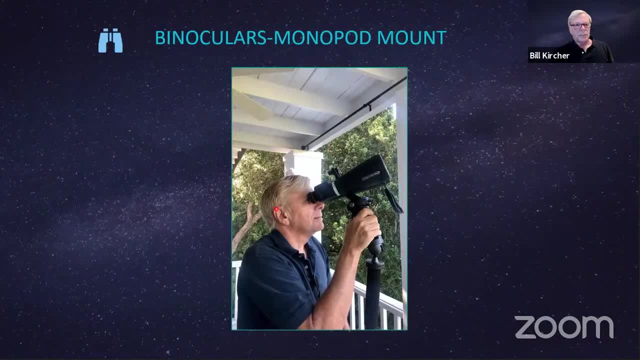 This is handy when you have to move around a lot, go up and down steps. The street I live on is quite steep And if I'm going to stand on that street I'll never get a tripod aligned, So I use the monopod. 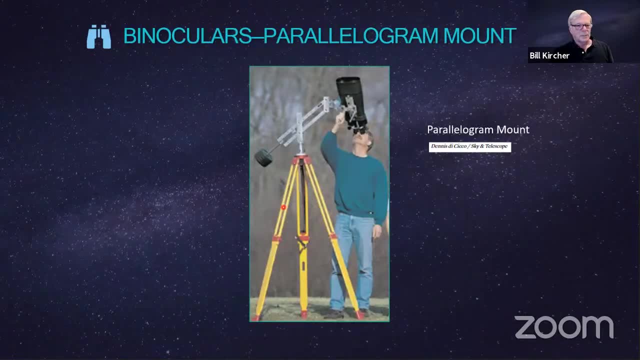 Another solution: the parallelogram binoculars, sort of the gold standard, But more expensive, heavy. You have a counterweight. Of course these are very large binoculars in the image And wouldn't work for me at home because I have to move around a lot. 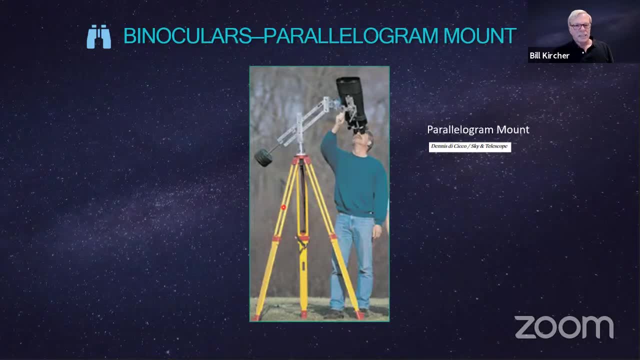 But very convenient. You can lower the tripod, You can lie down on a lawn chair and look up. When you let go of the binoculars, they stay. They just hang there. Very, very, very nice solution if you're going to a stable place and you'll be there well. 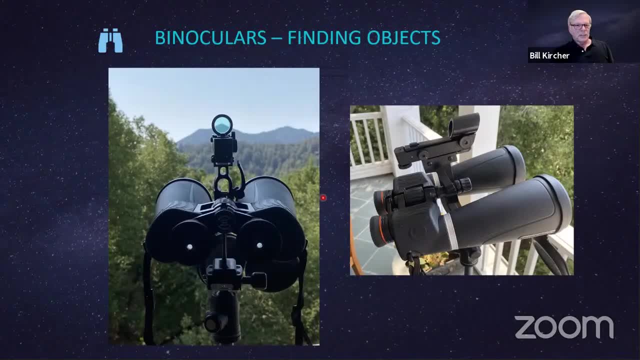 Well, what do we have here? Here's the red dot finder I told you about. It's been repurposed as a finder on my binoculars that came with a rail on top. Now, this is something you would only use if you had your binoculars mounted on some sort of a tripod. 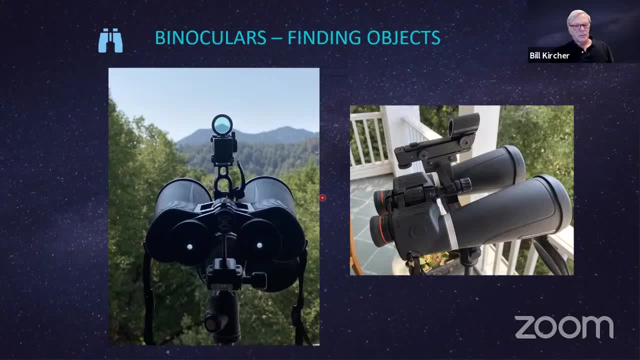 Because a major problem with binoculars is just steadying them enough to use them. If you don't have any kind of tripod or monopod, you should at least have some strategy of leaning against a post or a tree or a building. 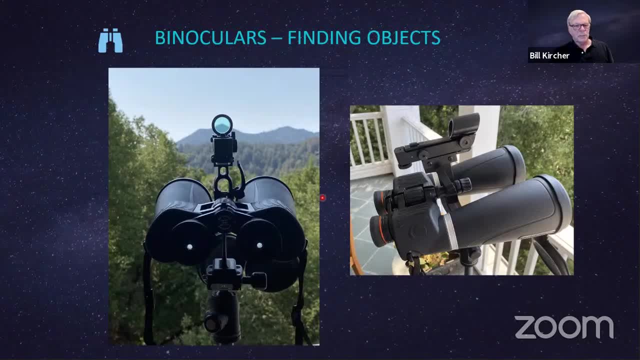 Something to give you a little more stability, because every little movement is going to be magnified. But if you are trying to find an object and it's one of those hard-to-find objects where a finder scope could be a help, here's a possible solution. 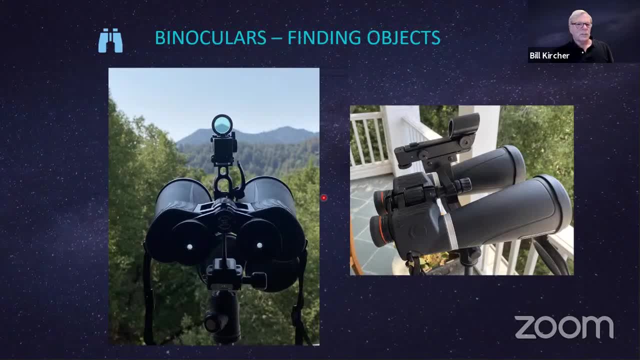 Use the red dot finder. I understand Celestron now has a finder you can mount that is not exactly a TELRAD, but more like a TELRAD. I haven't had a chance to really check that out, so there may be other possibilities. 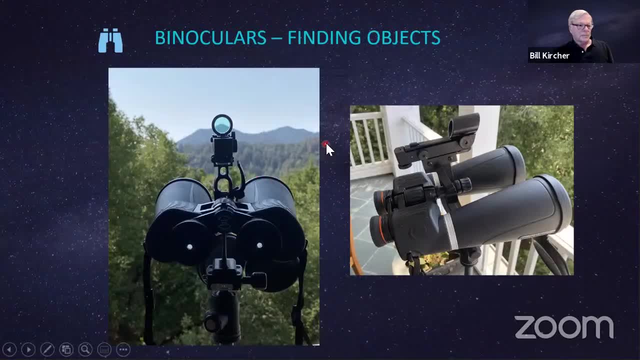 So here I have the red dot finder. It's focused right on a peak of Mount Tam. There is a small lookout station at the top of Mount Tam And actually you can see it in the red dot finder as a small notch on the top. 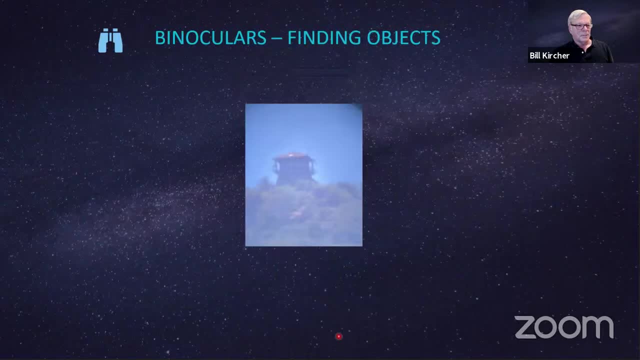 This is it. Look, this is an image I took through my telescope, So it wouldn't look like this. But through a magnified finder you'd still see something like this, but a lot smaller. But the red dot can actually locate this. 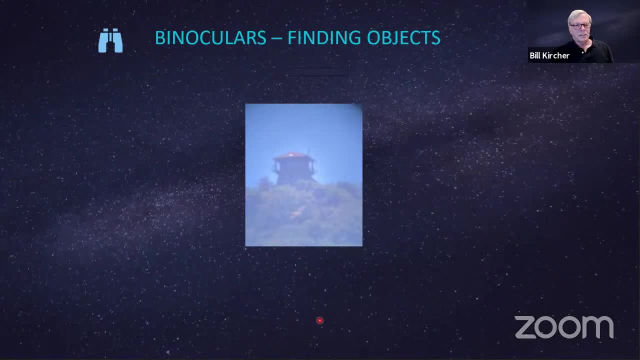 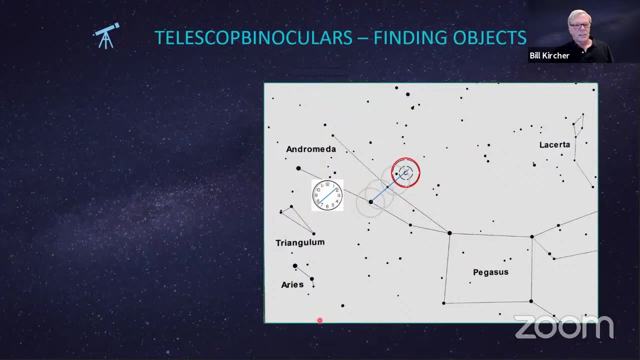 So how would you use this to find something? Well, let's go back to our Andromeda example. It turns out the field of view of this particular set of binoculars corresponds roughly to the reticle of the size of the TELRAD. 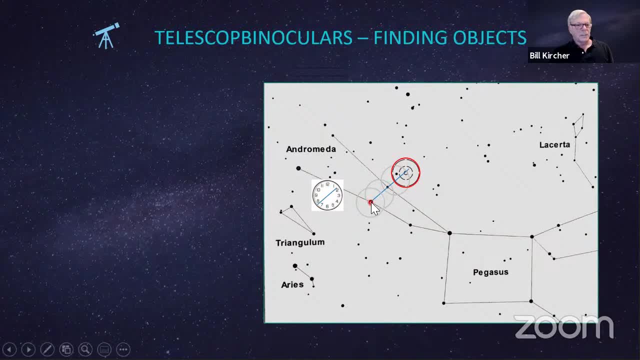 So start by locating MIRAC with the red dot And then go through this same projection, So you move the field of view of the binoculars such that MU is now at the eight o'clock position, And then you should see. 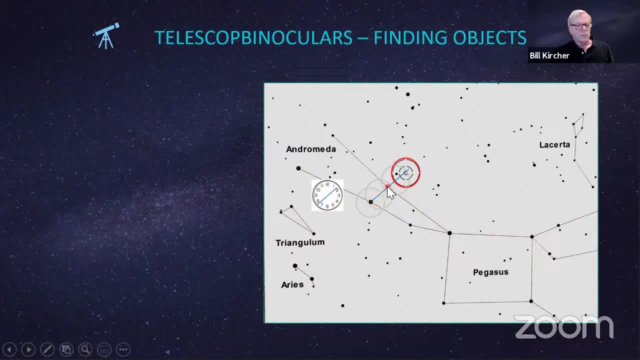 I'm not. I'm sorry. MIRAC is at the eight o'clock position and MU is at about the two o'clock position, And then you just have another step to keep going And there's Andromeda, Or one or two more steps. 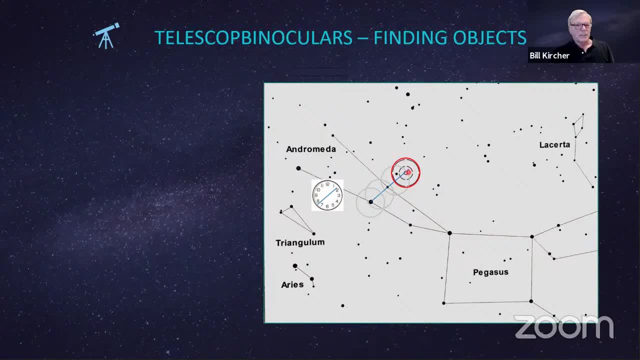 Now, in reality, Andromeda, for a pair of binoculars. it's so big it's not that hard to find. I'm just using this as an example. But there are some objects that are kind of hard to find but they're still worthwhile observing through binoculars. 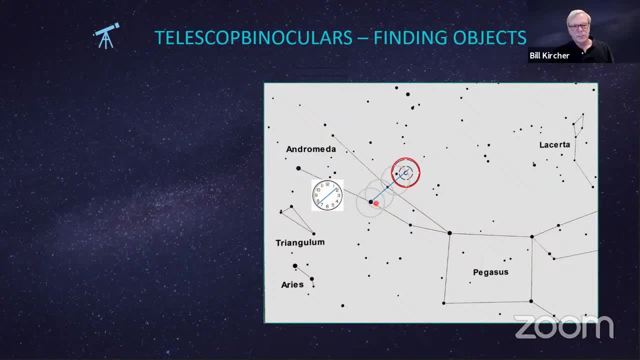 So if you're having trouble finding something, this is another alternative That may or may not work for you. Bear in mind that binoculars the magnification is lower than what you have through a telescope. At some point the binoculars are not going to make out details on Jupiter. 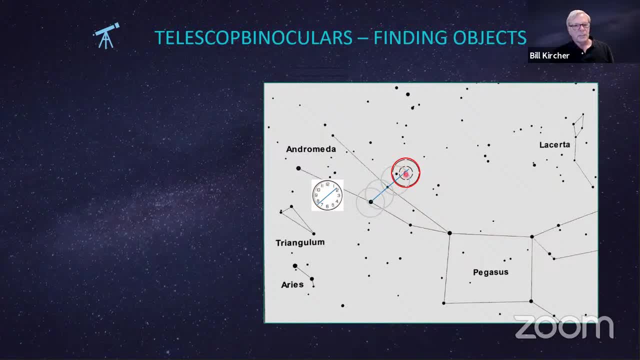 for example, You can find Jupiter but you won't see the bands of Jupiter. But binoculars are spectacular for objects like open star clusters And you can try to locate those clusters specifically, Or just go out and scan the Milky Way at night. 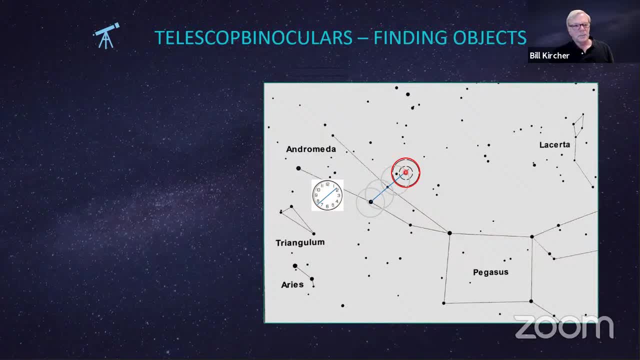 Sooner or later, you'll probably come to something that's pretty amazing. That'll be some kind of a large cluster, Particularly this time of year when the Milky Way is more overhead and we can see Sagittarius looking towards the center of our galaxy. 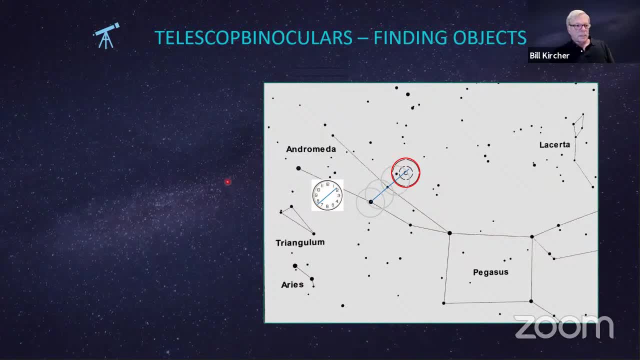 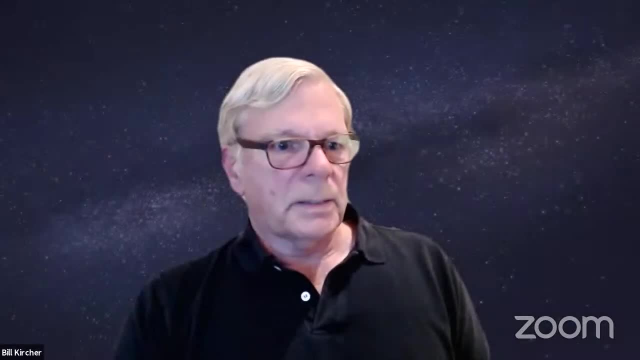 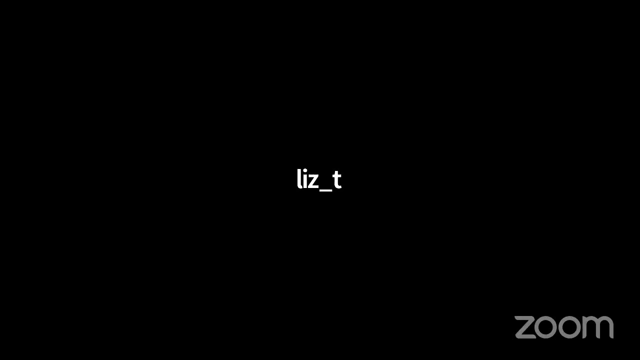 All right, So that that concludes the presentation, And let's I'll stop my share, And then let's let's move on to your questions. Hey, Bill, I'd be happy to kind of go through the questions that we've accumulated in chat. 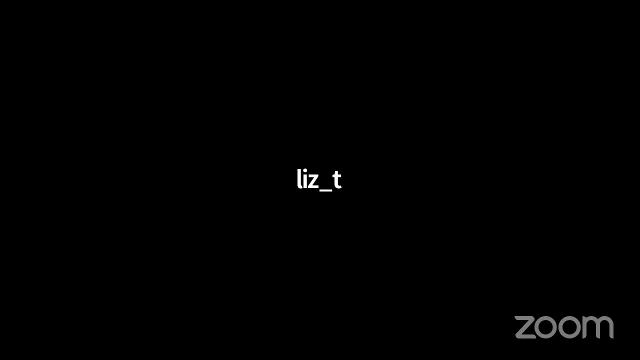 and put them out there for you so that you can just take care of responding. Sure, I don't know if you had a chance at the beginning, when we asked people what kind of telescopes they had, Some people did give us some info there. 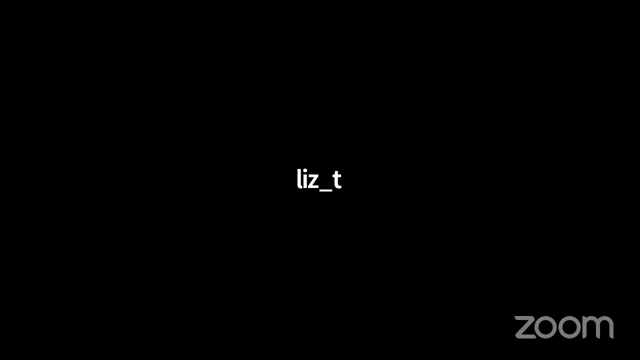 And I thought that I might let you know what what we've heard from members. I have a Dobsonian. Jerry has a six-inch Celestron SC. Ikea is probably going to. he had to drop off of the call. He'll probably be on the Slack channel in the near term. 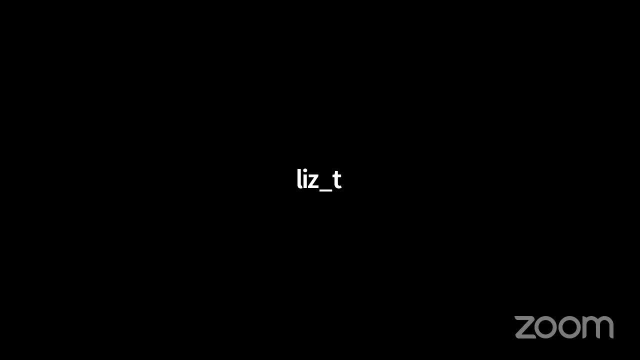 He wanted to learn more about the scopes And I thought that you might get on Slack to ask a few more questions. Helen has an Orion Skyview 6.. And that was the end of people putting in their info on on specific models. 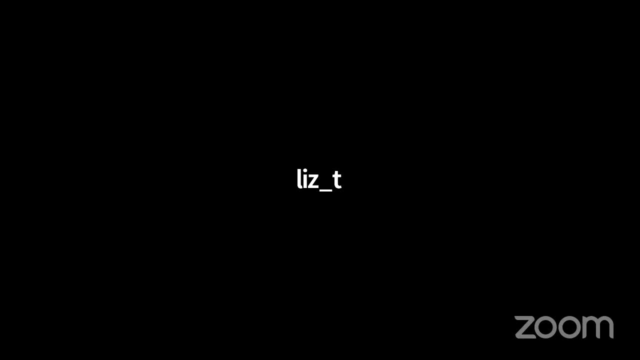 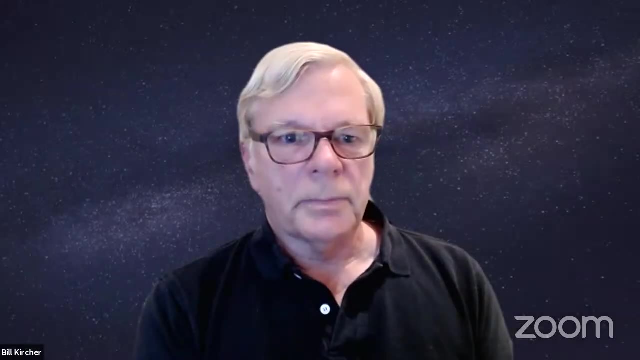 So maybe people saw that somebody had already listed something that they had, but I didn't know if you wanted to address any of those in particular. Bill, Yes, Was that a Celestron 6 SE or SC? SC is what it says here. 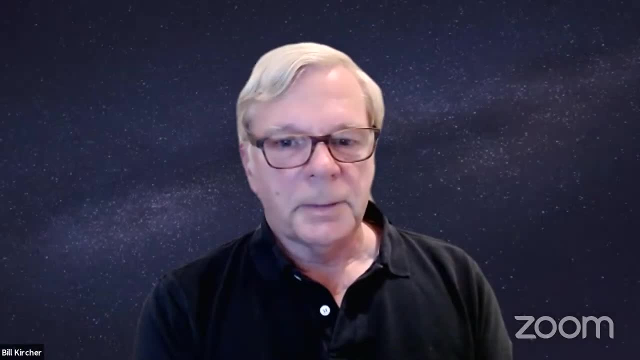 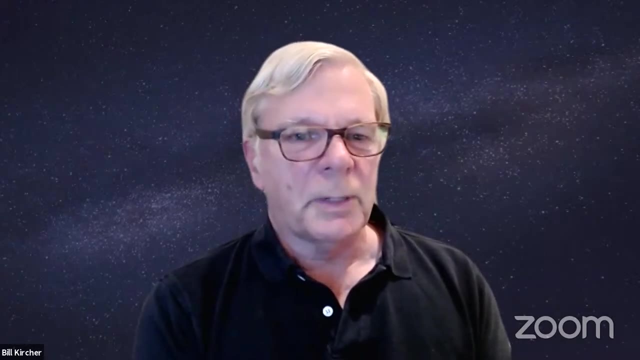 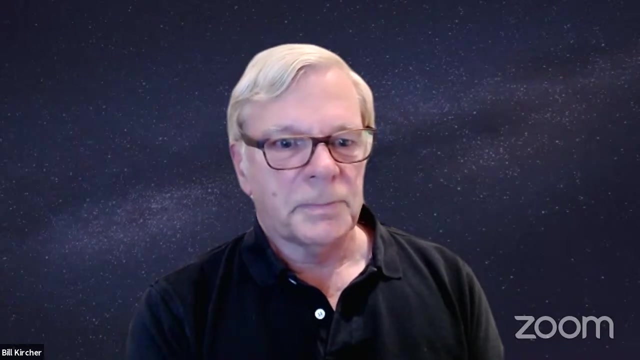 Okay, Yeah, Well, that that would be if I, if I, if I'm correct about this, that would be something similar to what I have, just a a bit smaller in terms of diameter, And so the my experience with my 8 SE would be directly applicable. 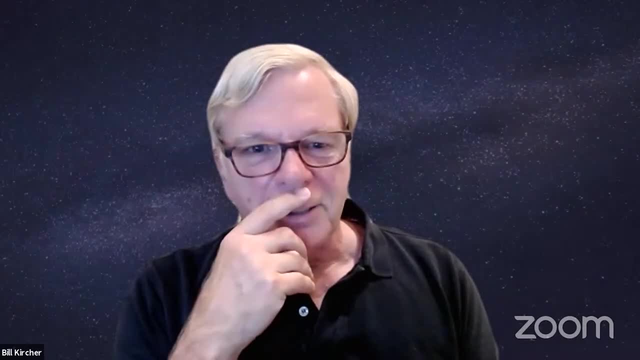 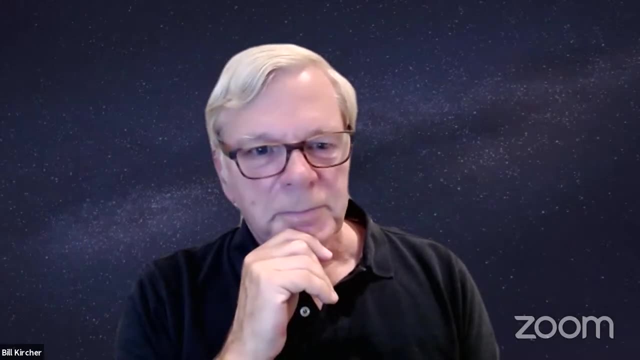 The Orion. I've, I've tried to call to mind what that that look look like. And I, I, I can't readily do that. And what was the other one, Liz, Let me scroll back, Oh you're. 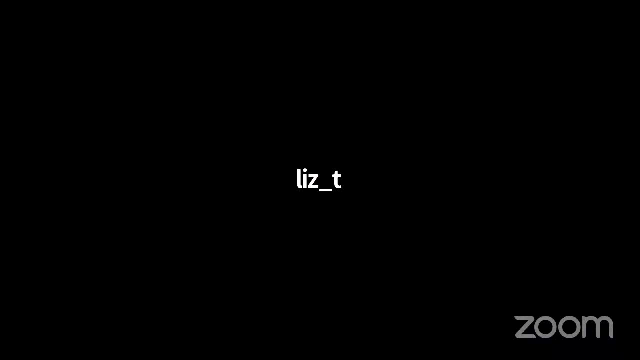 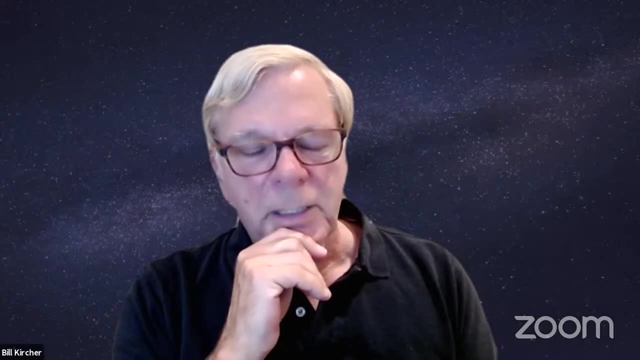 you're a daub, I know about you. And we had the Orion Skyview 6.. Skyview 6.. Yes, That's the one that I couldn't, couldn't, immediately recall. And then Bill, while we were just chatting about those, 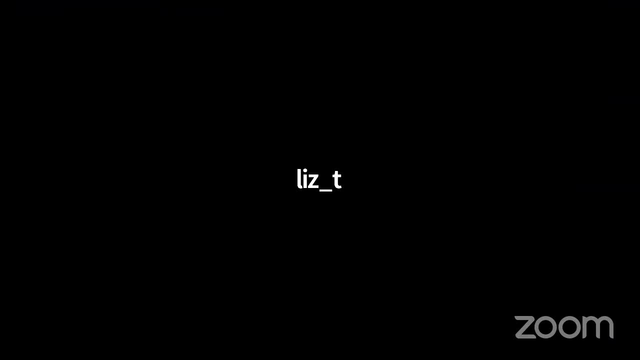 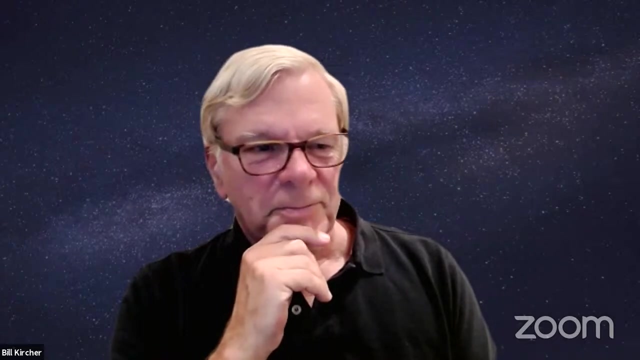 Tim chimed in is a 9.25 Celestron Next Star Evolution, And John has a Stellar View SVX80 and a Celestron Edge HD8.. Yeah, Nice, Very nice 9.25.. And then the Celestron Edge. 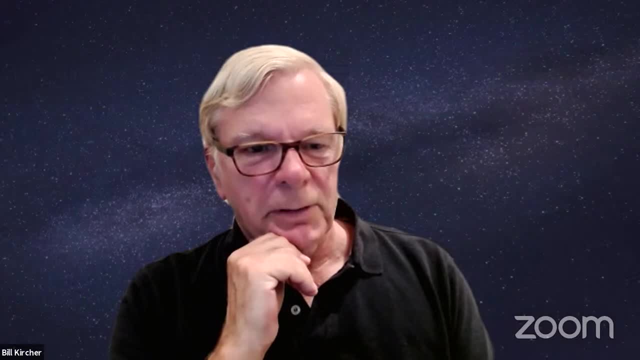 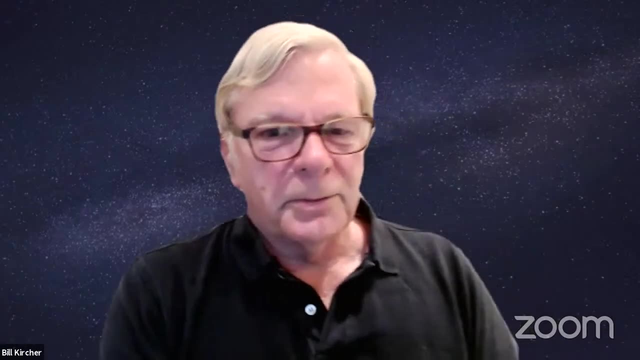 very nice scopes And Stellar View, of course, very, very high quality. Well, it looks like we have quite, a quite a range of of telescopes, Very true, And you know there was also a little bit of a dialogue going on before you started. 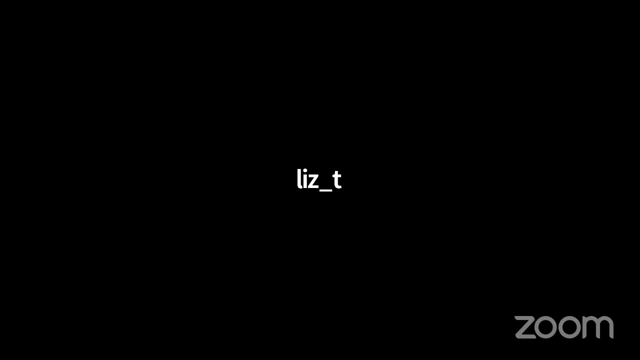 Jessica had mentioned about Douglas teaching the class on telescope making, So just a quick plug for that. Doug Smith is one of the SFAA board members. He's also in charge of our telescope loan program, which is available to members And when classes can be resumed. 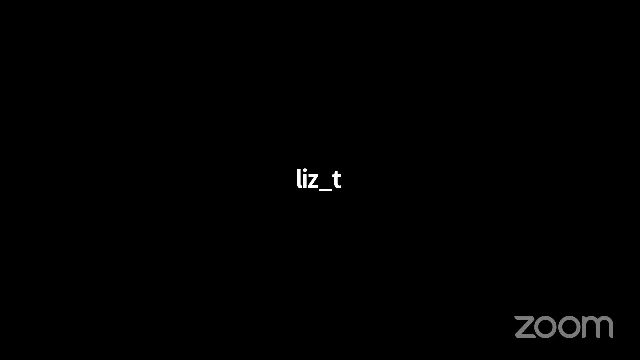 Doug will try to get that on the schedule again at some point in the future over at the Randall Museum. So if you have any interest in building your own scope, which a number of our members have done, then stay tuned for that And we'll 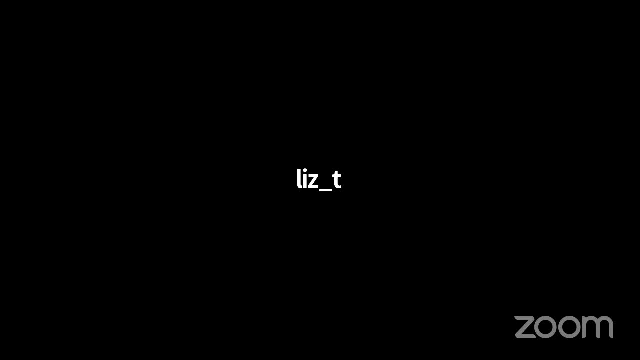 we'll let you know as that comes back online. Great, We had a couple of comments that that folks put in. I just thought you might like to comment on that, Cause it was nice that they put these in, kind of as you were talking and they were reacting to things that you had put in your presentation. 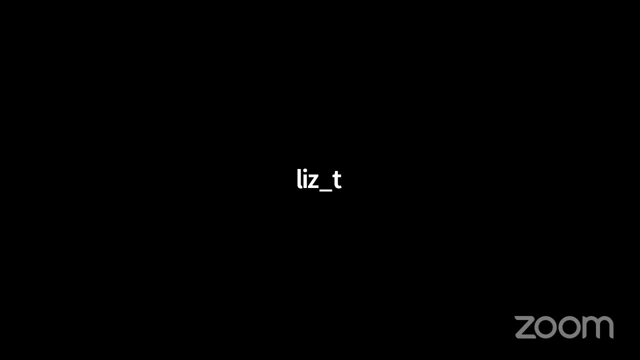 which I thought was loaded with great tips Bill Jessica had noted. she says I personally always have a roll of red electrical tape in my car When I go to star parties. it's easy to tape over those small lights in the car. 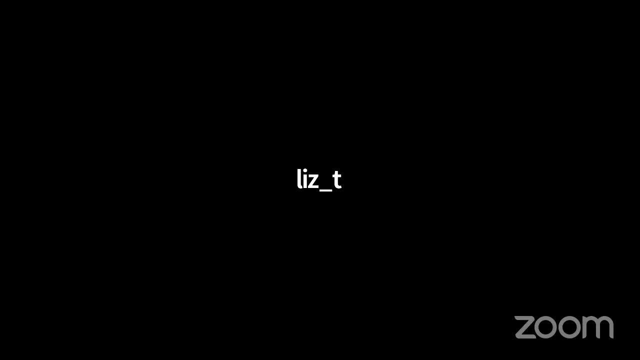 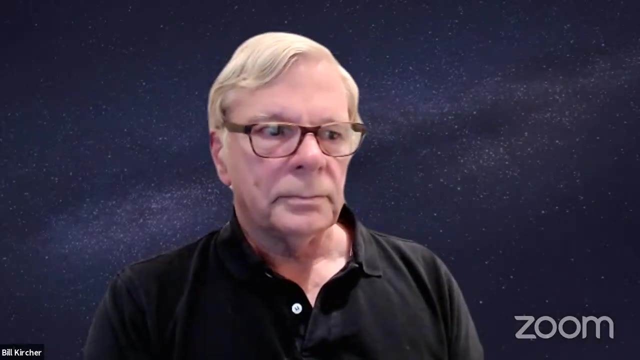 over a flashlight, et cetera, And then it's easy to remove after, And that's what you were talking about too. I think that's a great tip. Yes, And then Thomas had reacted to one of the things that you were talking about. 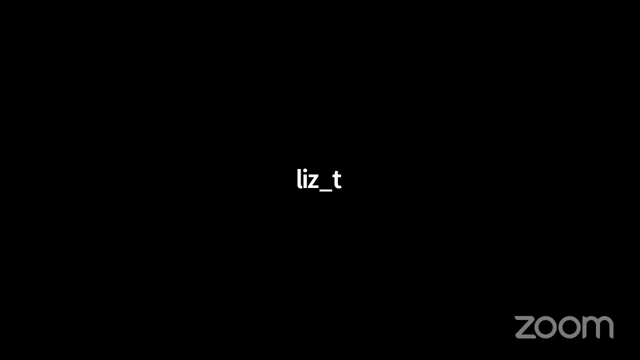 Bill. he said definitely recommend aligning the telescope and finder scope during the day with something like a tree or sign or other landmark object. on a dark night you'll get lost in a sea of stars. Totally, totally agree with that. Things look different. 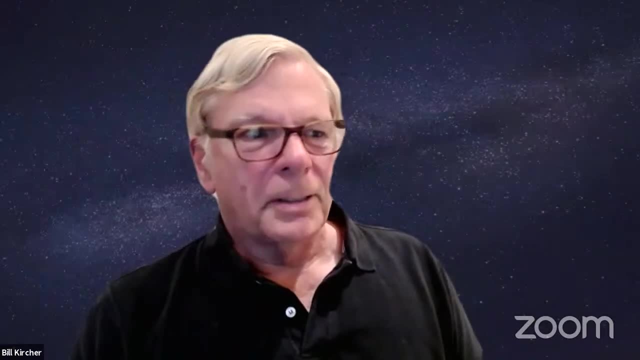 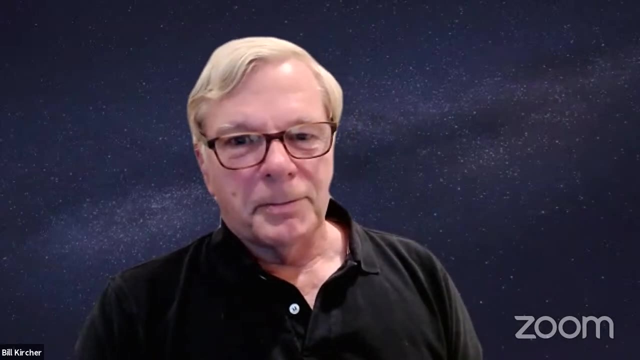 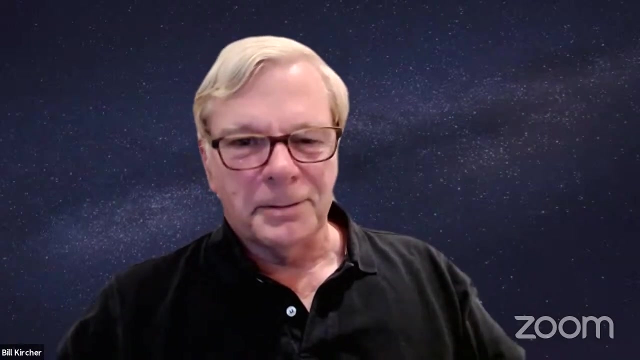 The sky looks. when you look at the sky, you see one thing: When you look through a finder scope that's magnified, you see more stars, a lot more stars, and the distances appear to be greater. And then you look through your telescope and, oh my God. 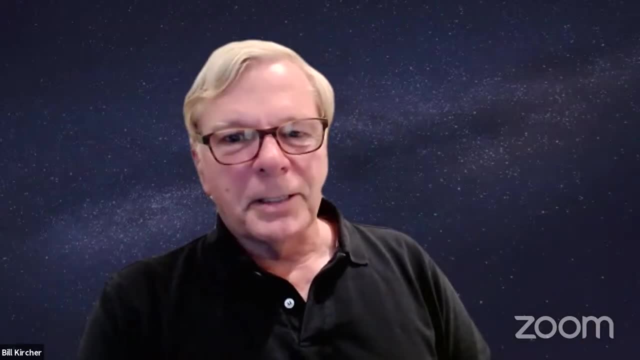 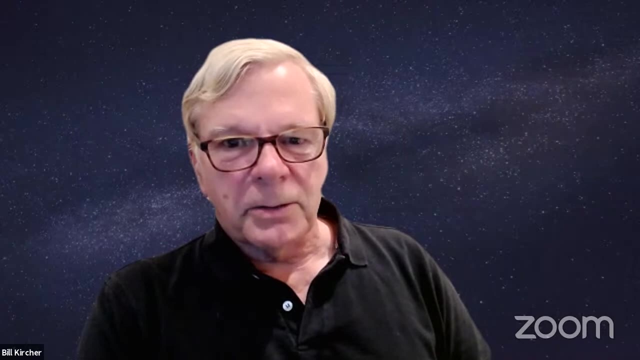 you know the even, it's even more disorienting. but during the day you're much better able to sort all that out And plus, as Thomas points out, during the day you can. you can find some sort of terrestrial object. 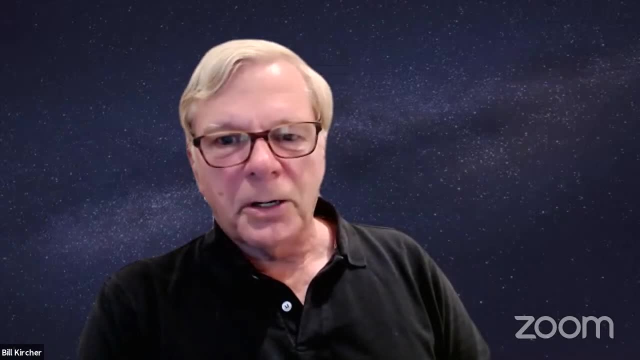 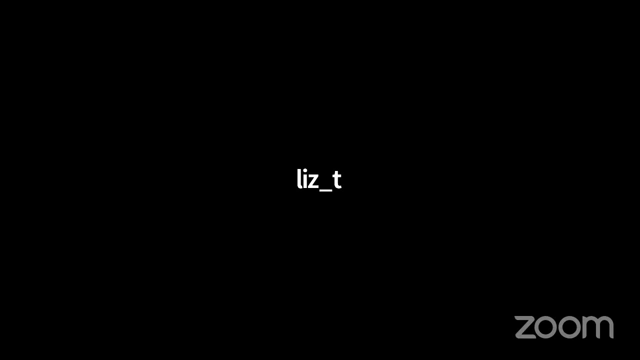 which you probably can't at night. You're you're just stuck with stars, and that is that is difficult. Well, that's a good point, And you know, I'm still such a beginner, One of the things that I'll definitely take away from your presentation. 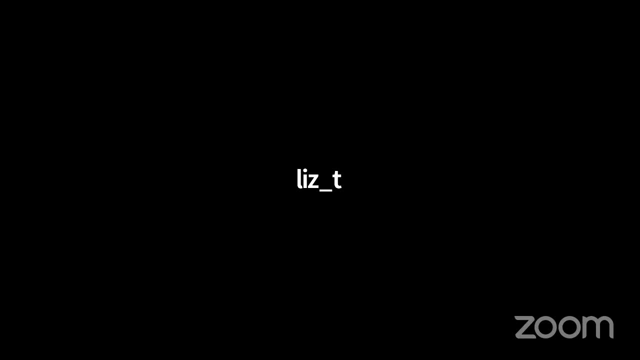 It's not just the preparation that you do at home to make sure that your, your telescope is acting properly and that you're familiar with it, because we do have to reacquaint ourselves with them from time to time, of course. But the other thing was your recommendation to have a plan for what you're. 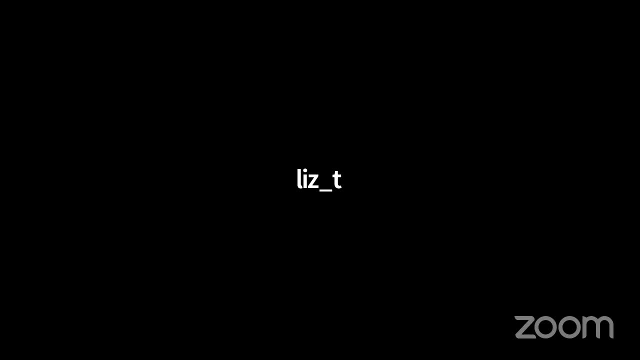 going to be looking for through your scope, And that's a great way to have an you know, make efficient use of your time and know where things are too. I found it to be a big help. At first, I didn't have a plan. 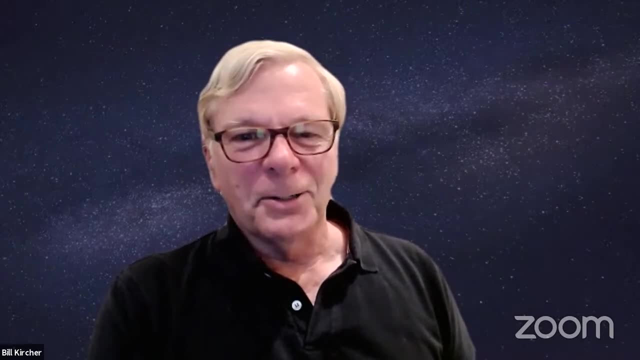 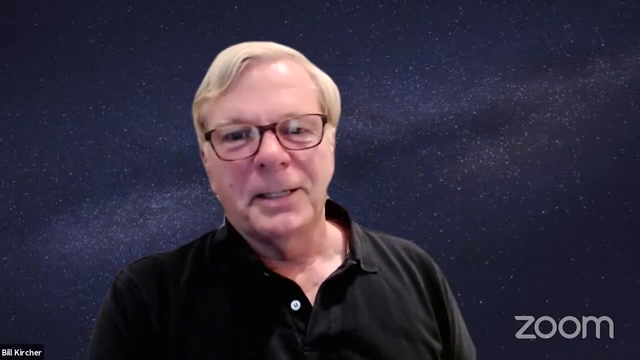 And when I finally got my telescope aligned I didn't really know quite what to do. And one one great thing about being at a star party is you can sort of walk around and see what other people are doing and get some tips. But still, 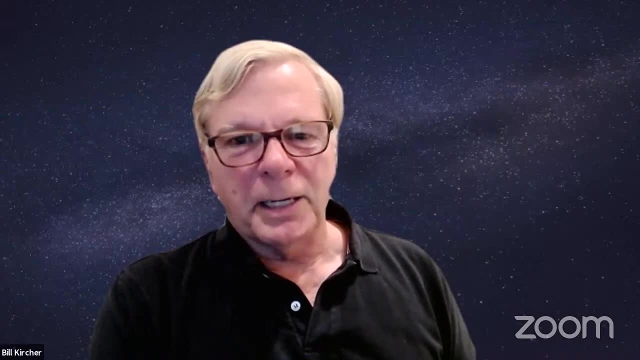 I think you you will always have a better experience if you do have a plan in a in a priority or prioritization of what you're going to do, But also an attitude where you're you're flexible If things change okay. 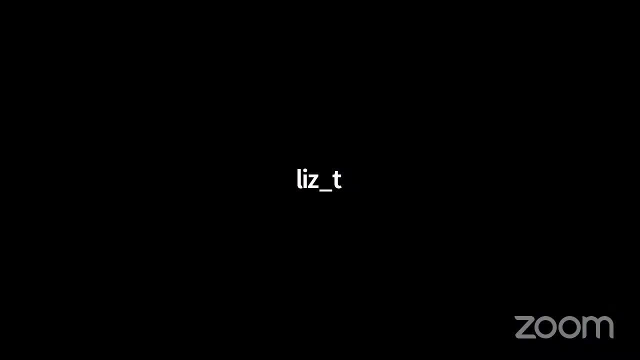 you change. Now. one of the SFA members told me that not only does he do a plan for what he's going to look at that night, but he keeps kind of a journal so he can keep track of not only what he was planning to see. 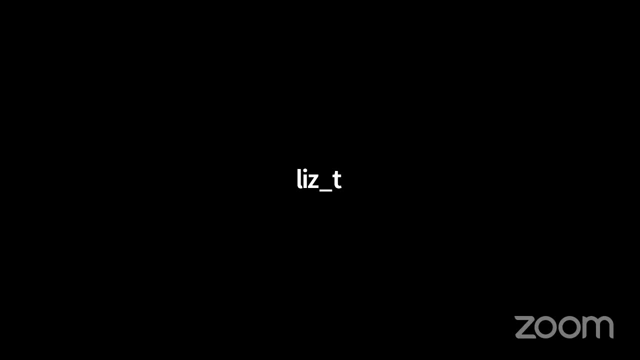 but then he knows what he has seen And then I guess from time to time he may want to see something again, but it helps him to sort of progress. It's a big sky, So it helps him progress through a wide range of things that he wants to. 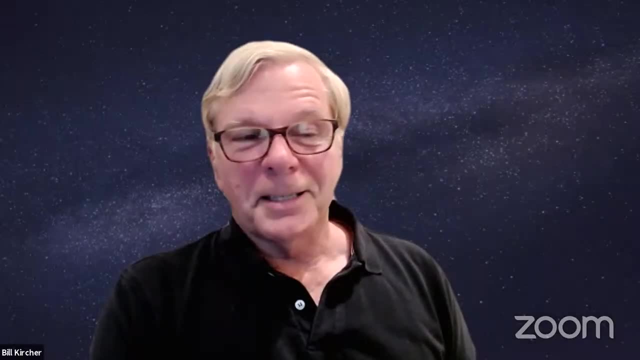 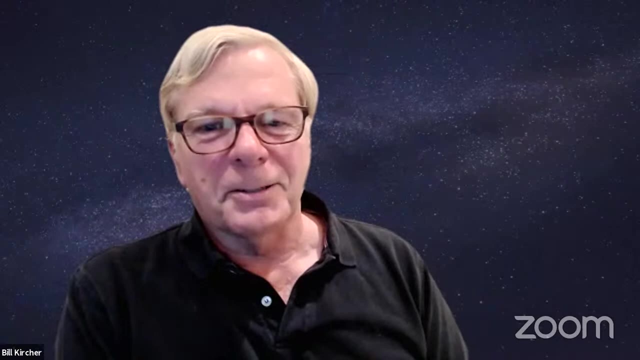 see over his lifetime. I think that's a great idea. I should do that, I keep intending to do it, but I I haven't really done it And I had this odd experience of using my EV scope to do some astro imaging. 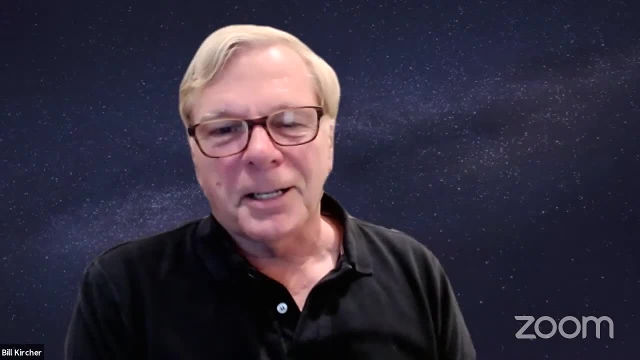 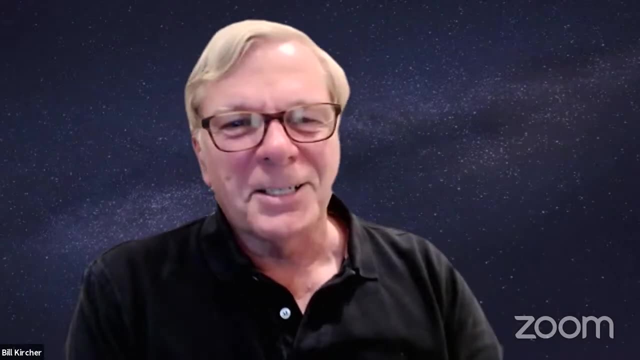 And I I imaged this- I think it was a cluster- And I thought to you that this whole, this whole thing sounds kind of familiar. Well, when I looked through my photos, I had just damaged it a month earlier. So 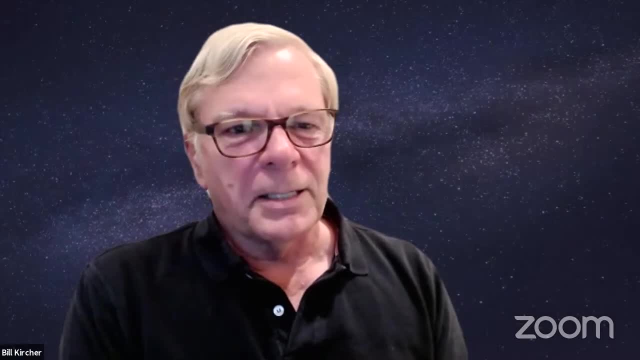 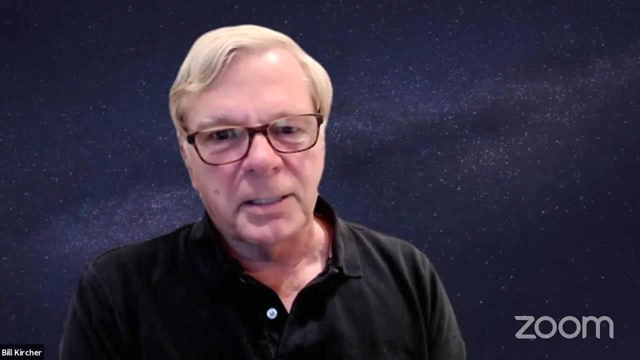 yes, definitely, But the other? the great thing about journaling is that that you, you know, it becomes your kind of knowledge base. You, you make notes and you remind yourself of things And it's, it's your. 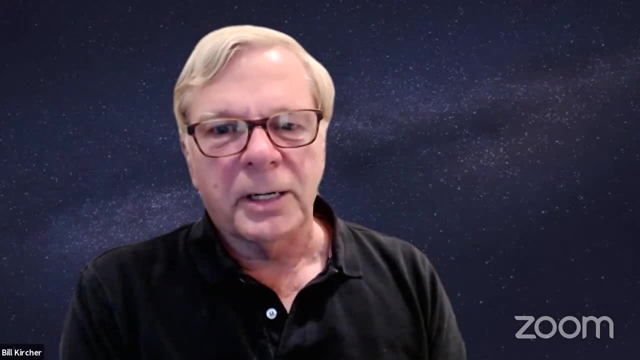 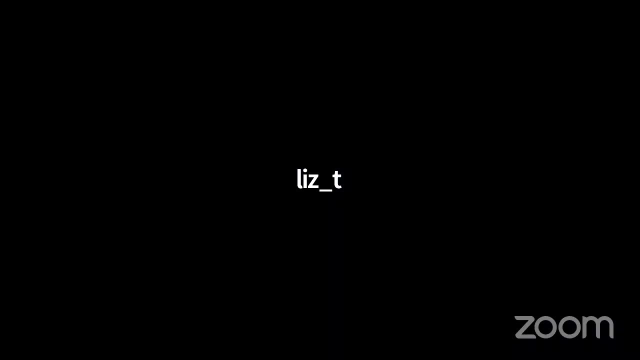 your. your progression, I think, is more, more deliberate and more organized. So great idea. Hey, we're happy to take more questions. If anybody would like, you can go ahead and type them in the chat, or you can unmute if you'd like to just ask Bill directly. 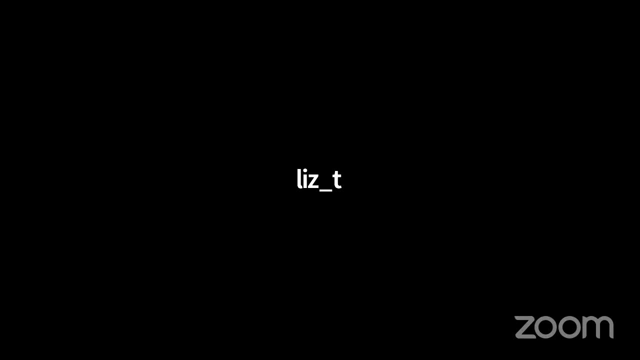 And while we're giving you a moment to do that, Bill, the question I had for you. when you were talking about the lenses and filters, I think you mentioned, and maybe your photos even had- a couple of the brands represented. I liked your point to not necessarily just buy a kit of six or however many. 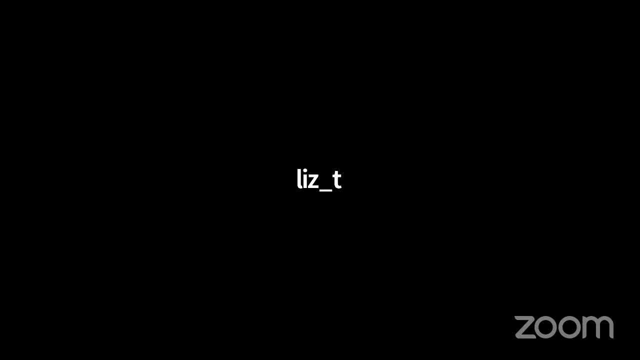 they might be packaged, because that really might not be the highest quality or or really you might not use them. But are there any particular brands that you recommend or that you've had bad experiences with that you'd recommend that we stay away from? Well, 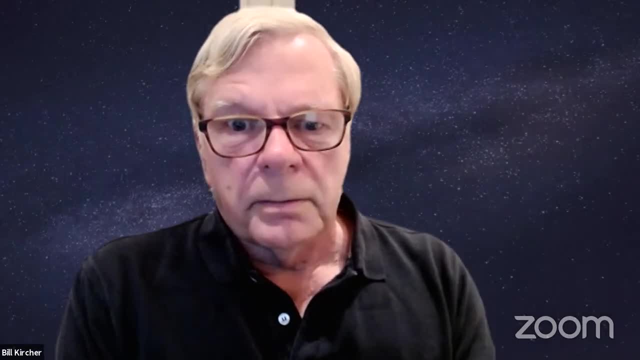 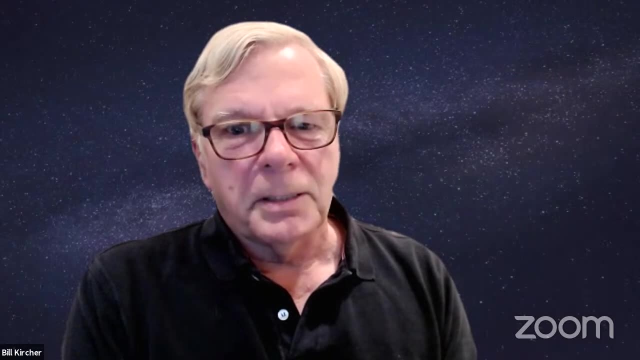 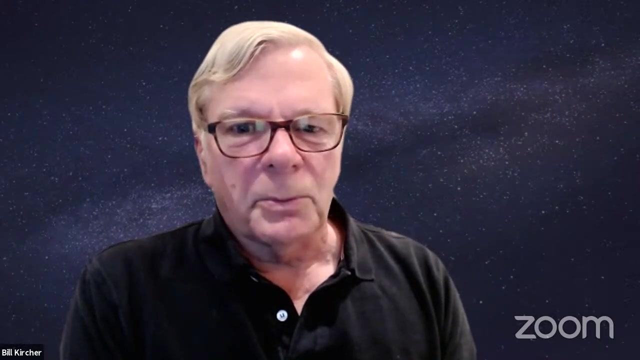 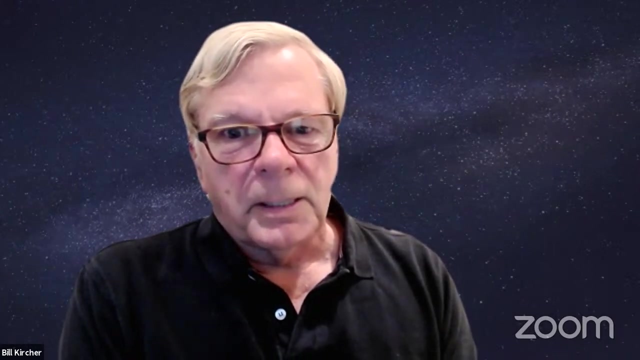 there. there there are some lenses that are are really inferior. I I mean the- even with a relatively inexpensive telescope. you at least want sort of a kilner lens Plus, so would be better. Now, these are more types of lenses. 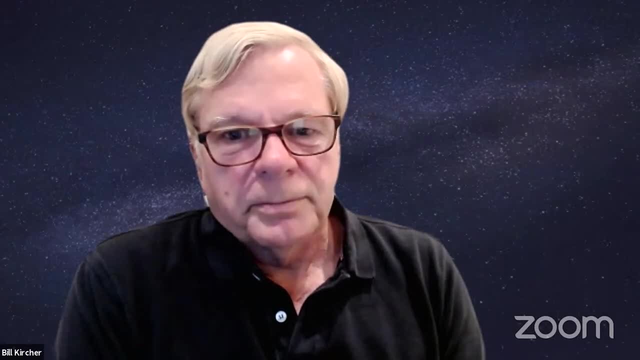 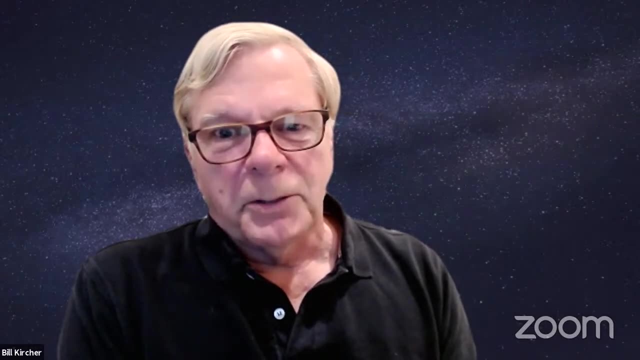 I mean, frankly, when I started out, I just bought Celestron and I was like, well, you know, I'm going to buy a couple of different lenses plus the lenses, But then, when you're ready and you want to buy better lenses, 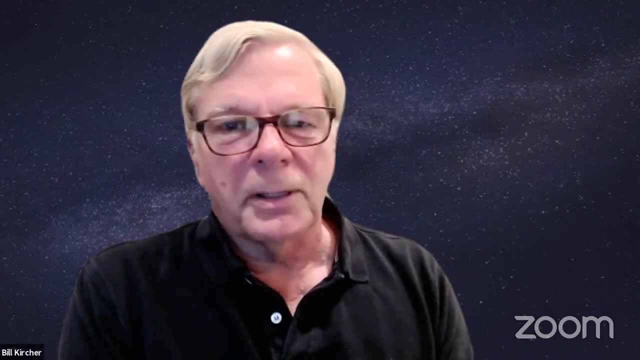 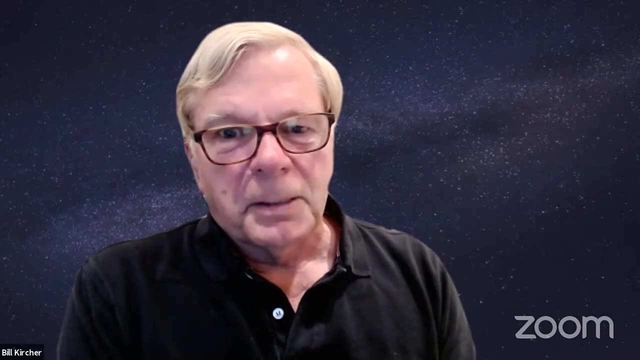 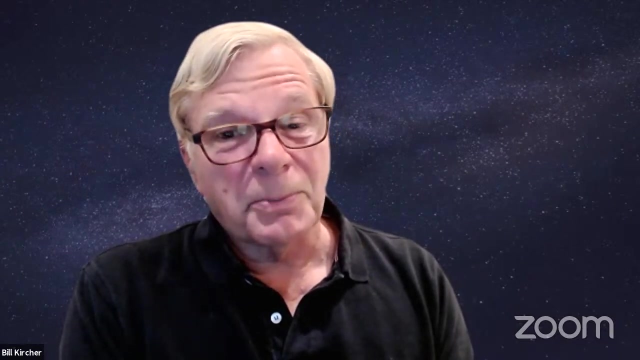 Celestron has a higher level of lens. They're more expensive, They're better. But if you really want a good lens, then you would probably probably go to a different manufacturer. but they're expensive. I mean you easily spend three. 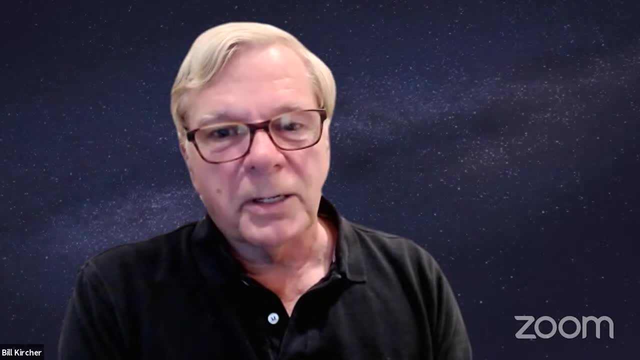 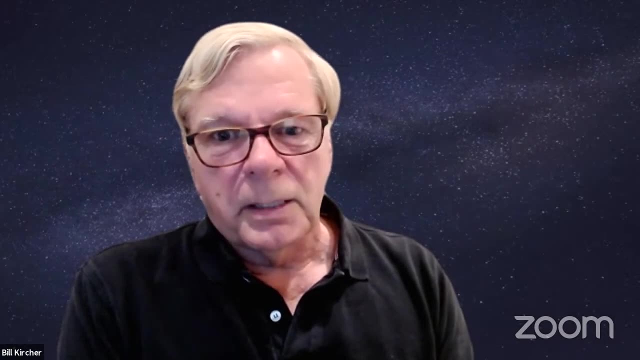 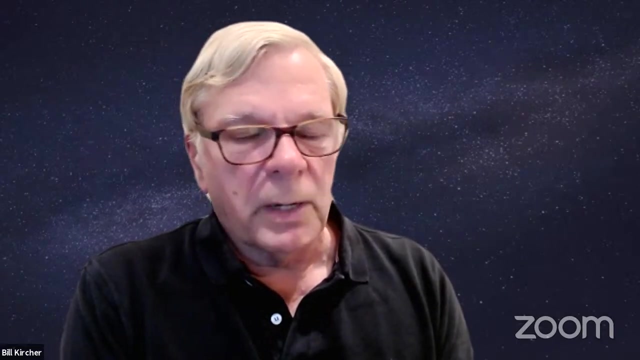 150 on up to 600 or more dollars on a single lens And what you get is you get better quality in the optics, better coatings and some of these more complex lenses that have many parts, mostly to give you a wider field of view and to also eliminate any aberrations. 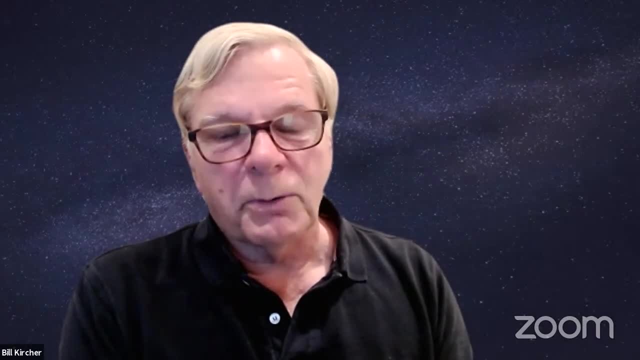 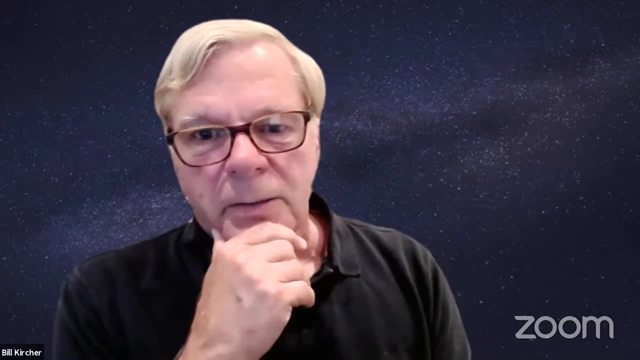 They're they're. they're difficult to construct and therefore quite expensive, and the materials are expensive. So that's why you get these high prices. But there are there. Well, I would just go on the internet and look at the reviews and so forth. 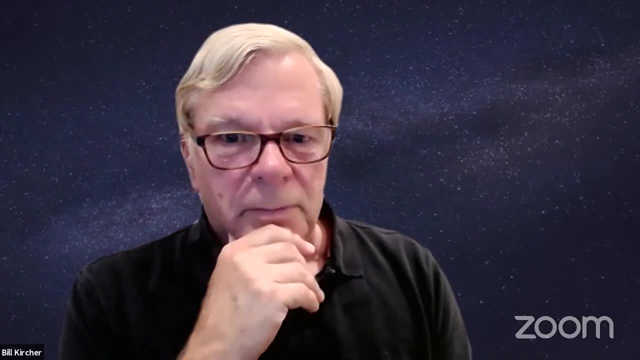 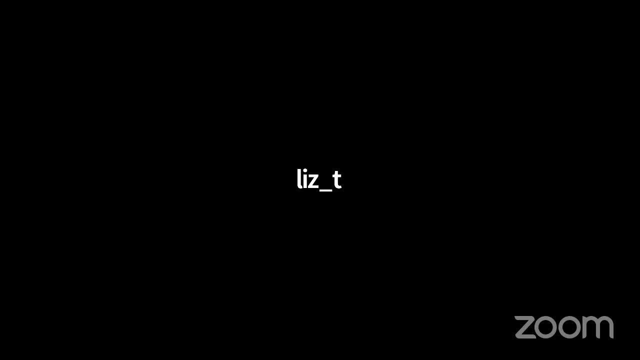 You'll get an idea pretty, pretty quickly, but there are some, you know, manufacturers that have a very good reputation. I think I'll do that, And then you can expect an email, or I'll go on the slack channel and ask for some input as well. 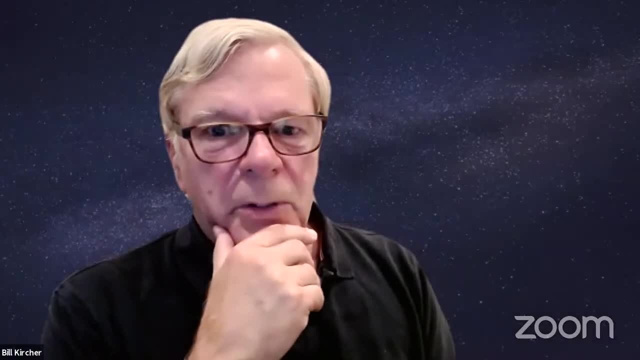 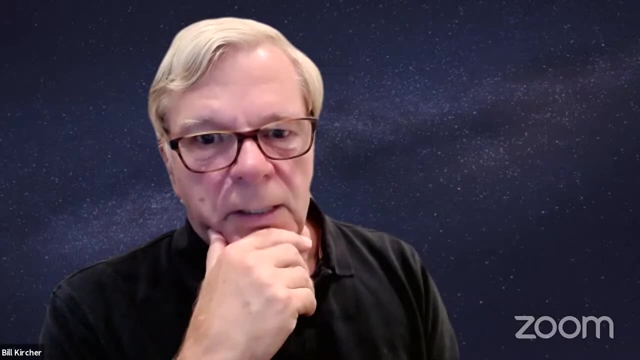 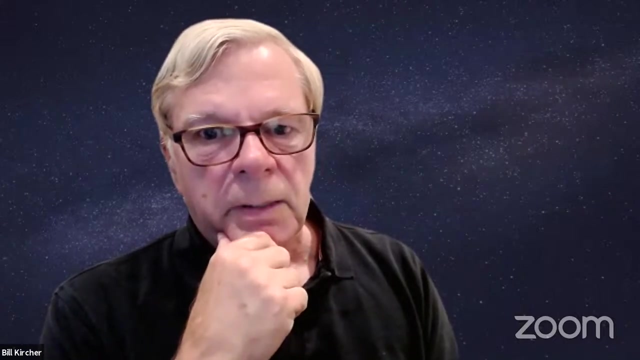 Sure, Yeah, you know that book I mentioned, the backyard astronomer, has a great section on lenses Slightly out of date, but some of these lenses are really classics and they they group the lenses in categories and they make specific recommendations about lenses in different price ranges. 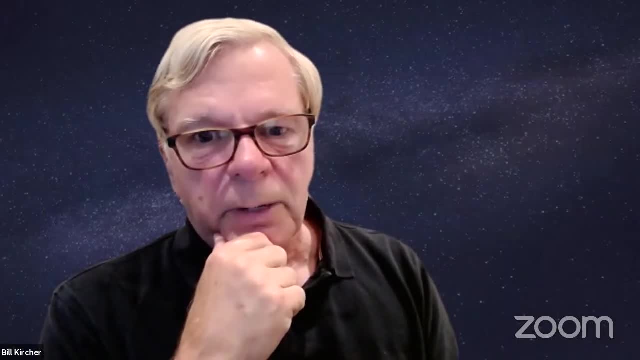 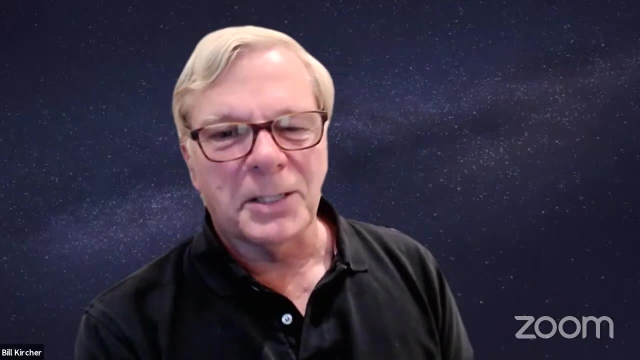 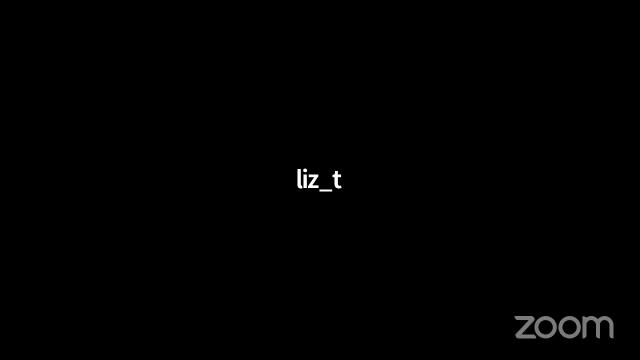 And so something like that would be a great resource. I I'm really anxiously awaiting the fourth edition of that book because there's so much great information in it. Very well done, Very well, Thank you. Good to know. So any other questions?